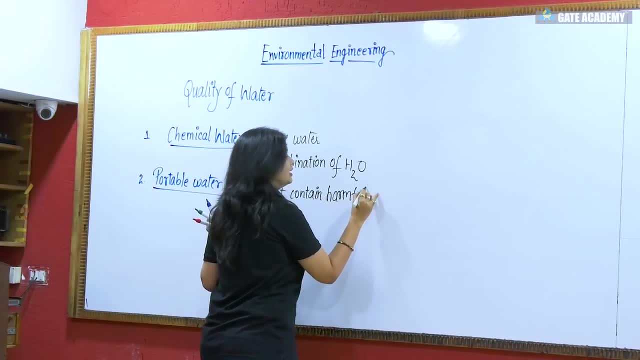 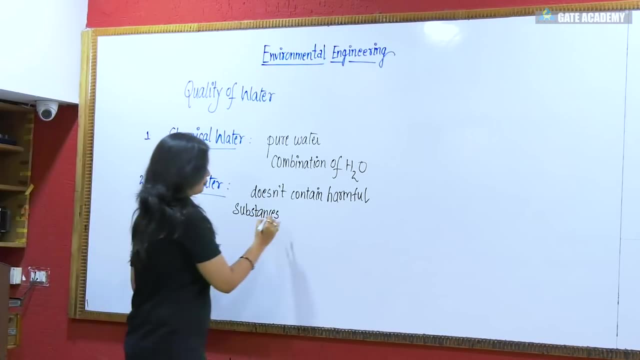 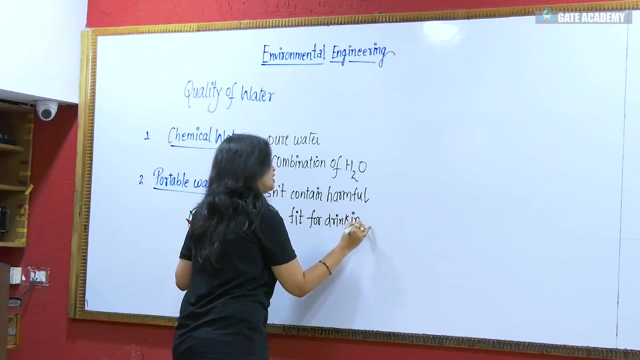 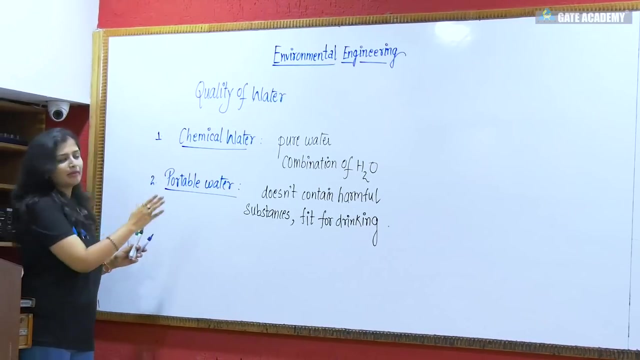 does not contain harmful substances and we can say it is fit for drinking. fit for drinking. Now, after the potable water, we will be dealing with palatable water. these are one liners, just for you to know. what are this- chemical water, potable water, and how you differentiate. 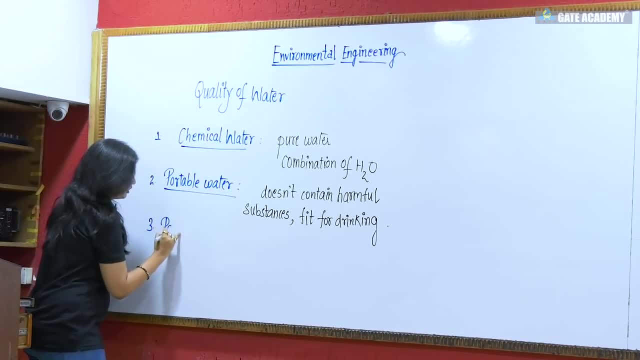 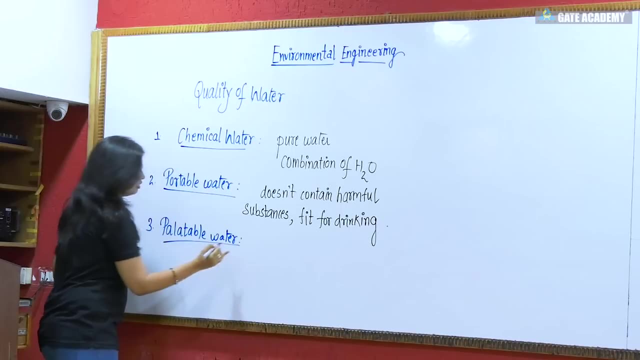 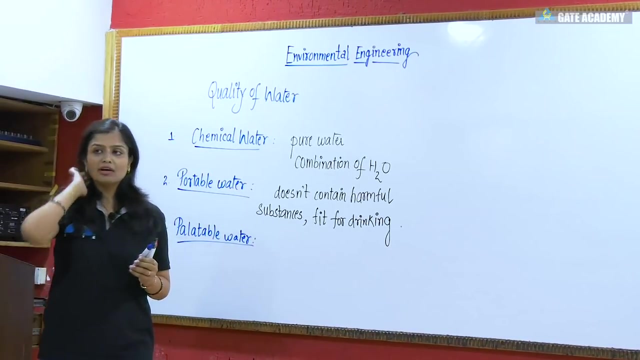 it fine. So the third one is the palatable water. palatable water, Now, this palatable water looks aesthetically good. that is, you can see from the front that the water is good, but you do not know, it is possible that the water contains dissolved. 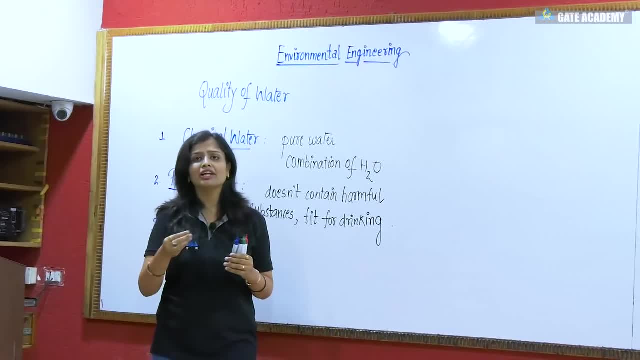 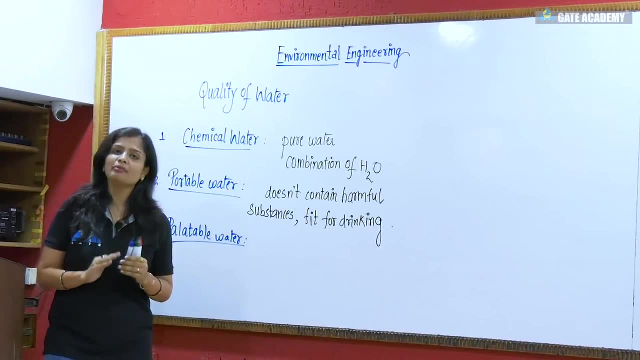 impurities present, okay. Or it is possible that there is any bacteria hidden in it that you are not able to see. so we do not say that this water is good, Okay. We say that you can consume it, but we say that it is good to see, okay. 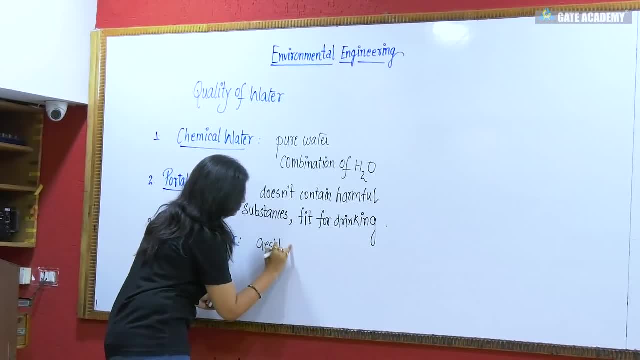 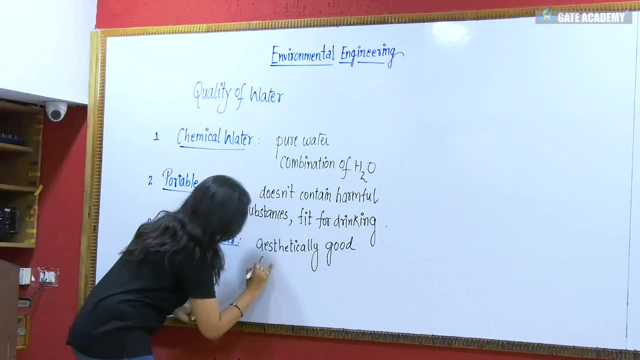 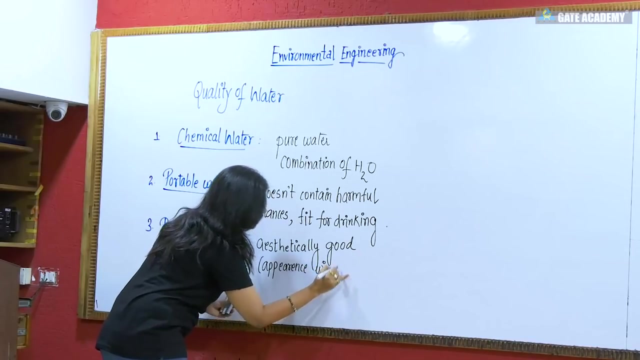 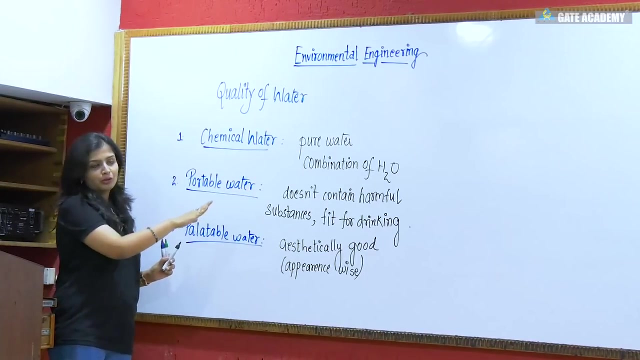 So we will write here aesthetically good. aesthetically good aesthetically means appearance wise, it looks good to see. and one more thing: if any water is palatable, it does not mean that it is a potable water. 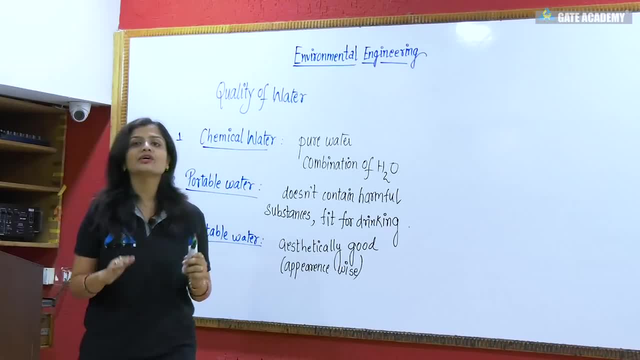 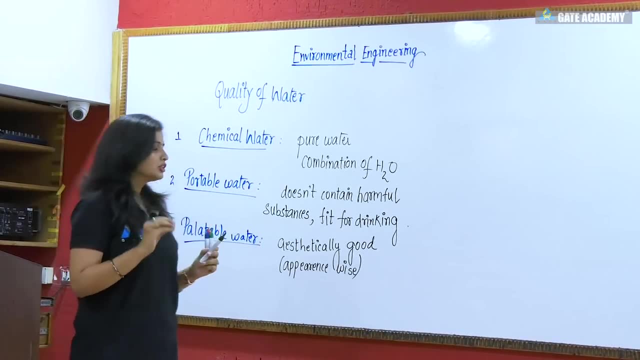 If any water is good to see, it does not mean that it does not have any harmful substances present in it. It may be that there is any amount of dissolved impurity present in it, So palatable water is not necessary, potable water. 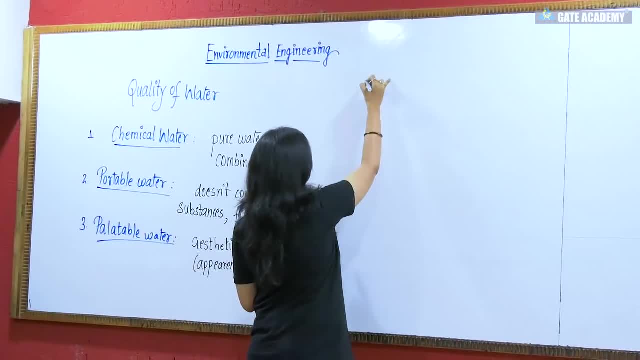 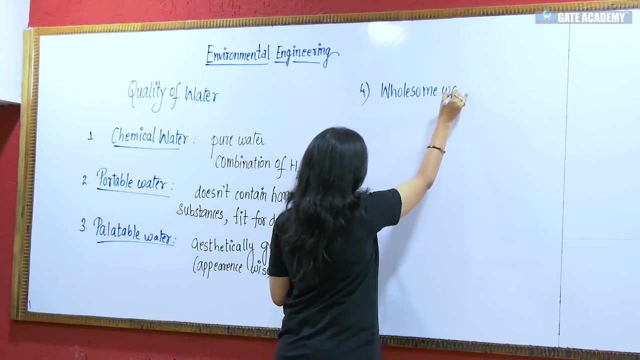 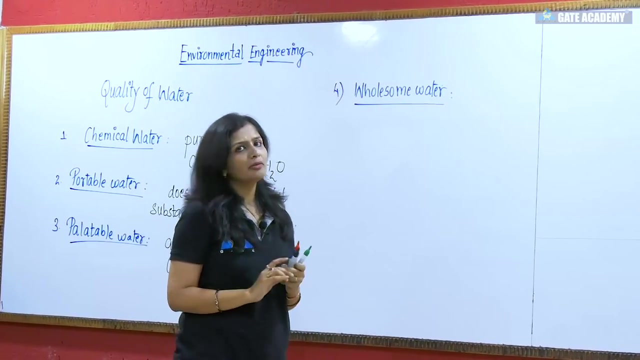 Now coming to the fourth one, after palatable water, is wholesome water. So the fourth one is wholesome water, And water is important. It is important, Okay. The meaning of wholesome water is that it is not chemically pure like what is chemical. 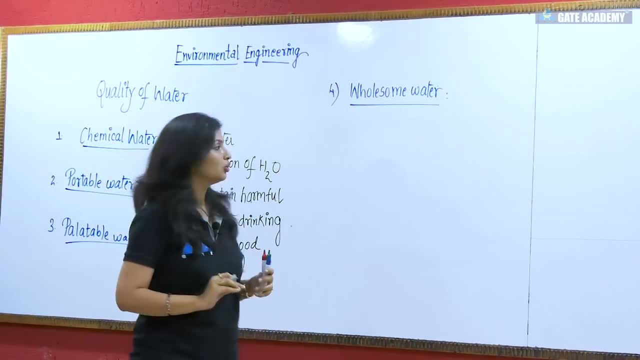 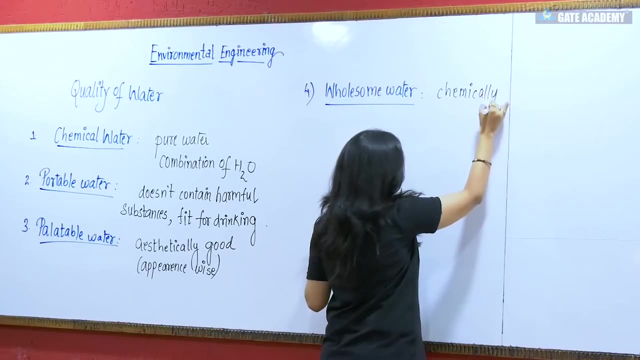 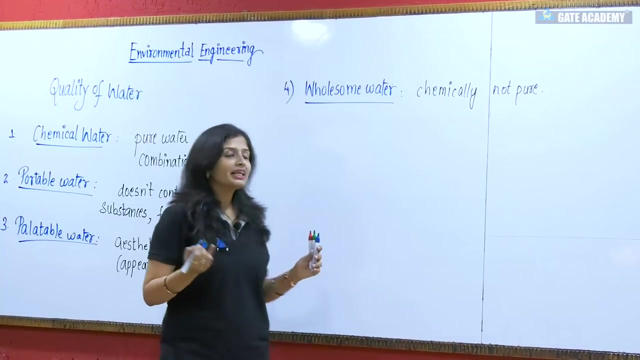 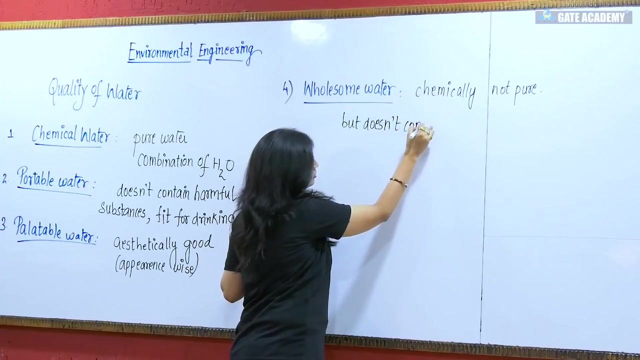 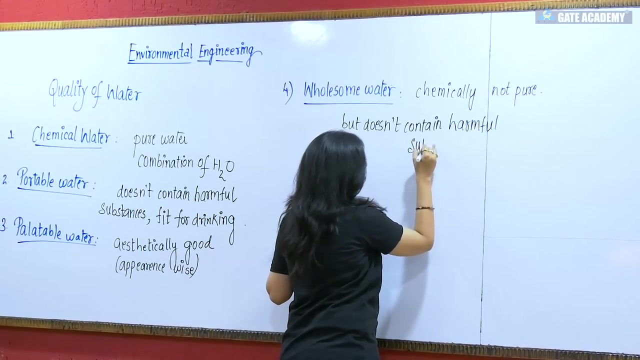 water. It is pure water. it is a combination of H2O, so we call wholesome water that it is not chemically pure. chemically not pure. okay, it is not chemically pure but there are no harmful substances present. but doesn't contain harmful substances. fine, now wholesome water is done. 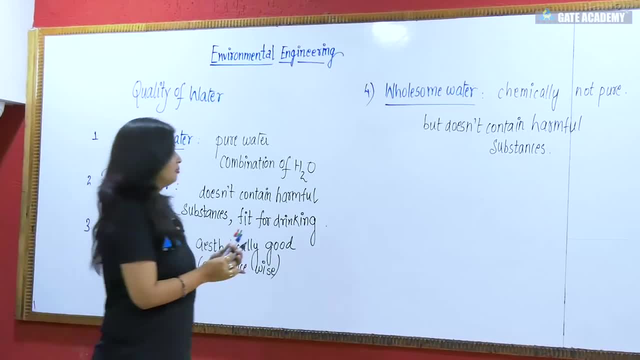 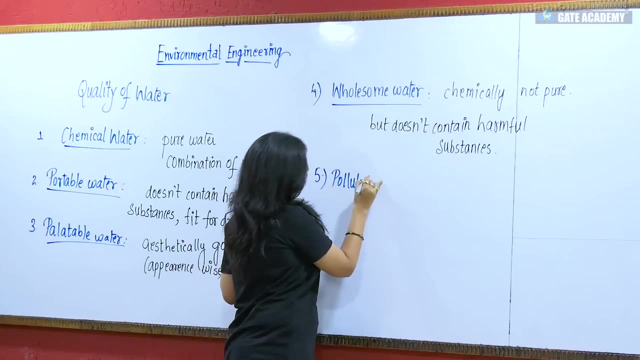 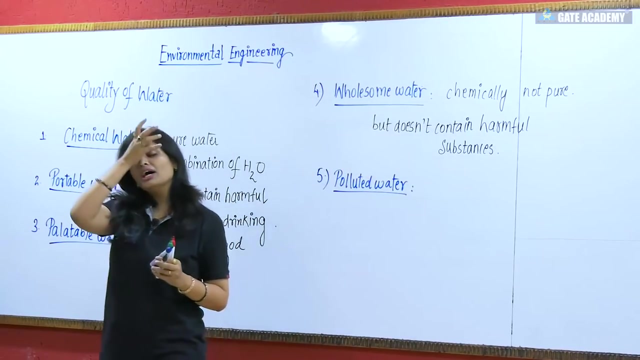 now, after wholesome water, you must have heard about polluted water, that this water is polluted. so if you have heard such terminology, then you should also know that. what is polluted water, What is polluted water? Polluted water is that in which harmful substances are present, means some bacteria are good. 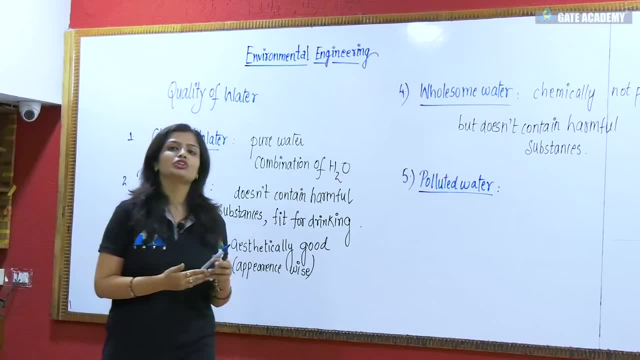 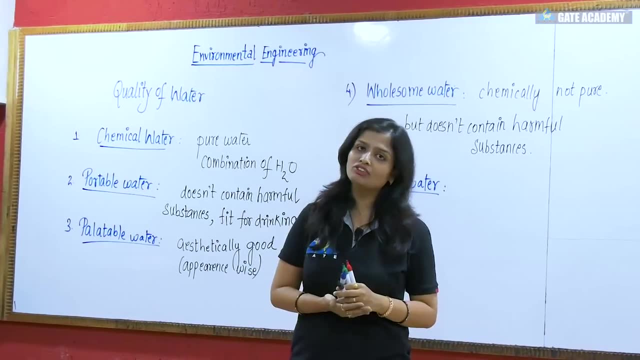 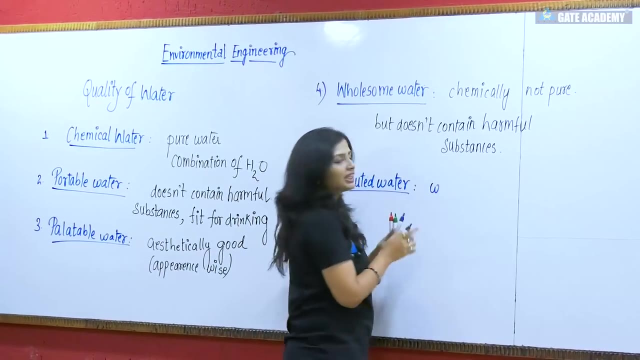 for our body, good for the synthesis of our digestive system, good for digestion. but if anything is more than its permissible limit, then naturally it harms our body. similarly, when we say polluted water, so it means water which contains harmful substances, water which 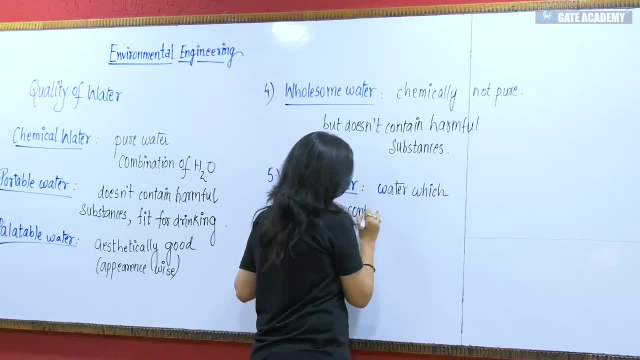 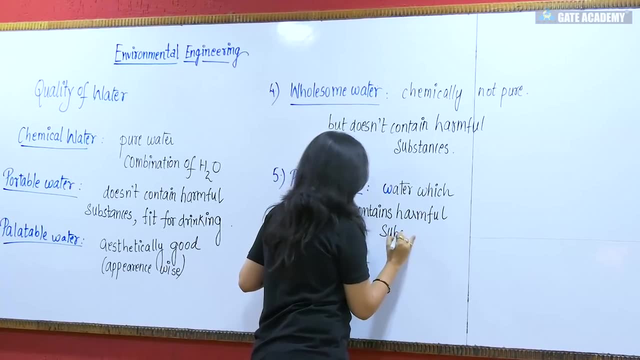 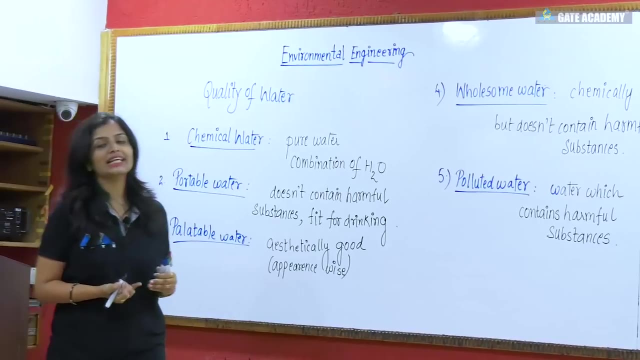 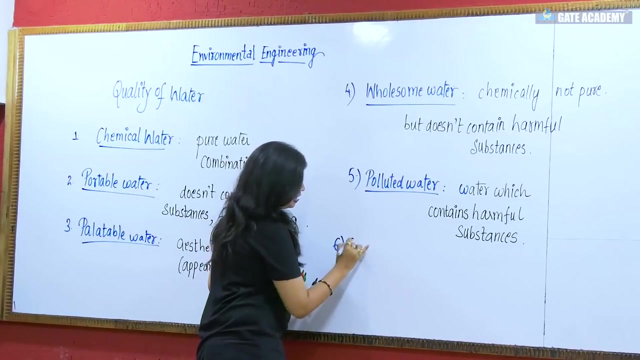 contains harmful substances In that water. you saw the name: polluted water. that means olduğu water which contains harmful substances, which means our contaminated water. so, after polluted water, we are going to say, really well, what is contaminated water now? what is contaminated water? 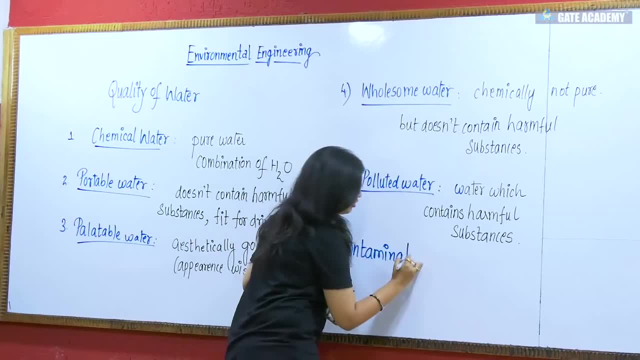 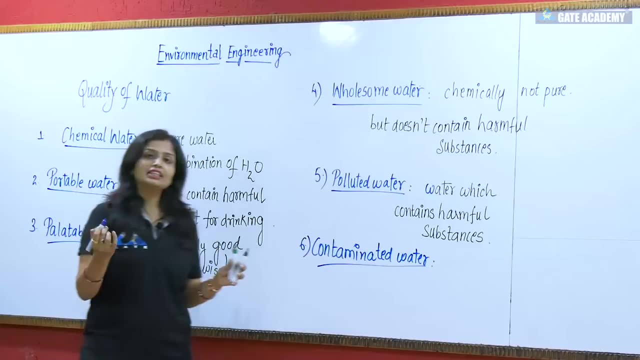 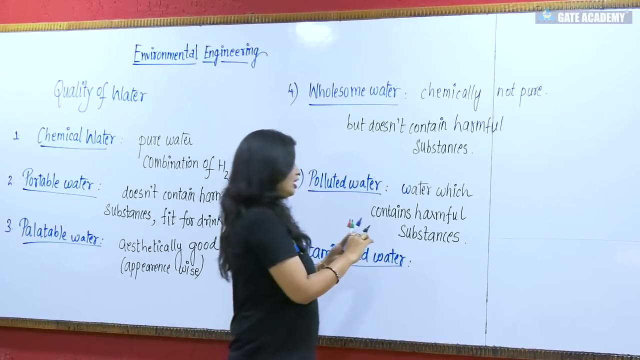 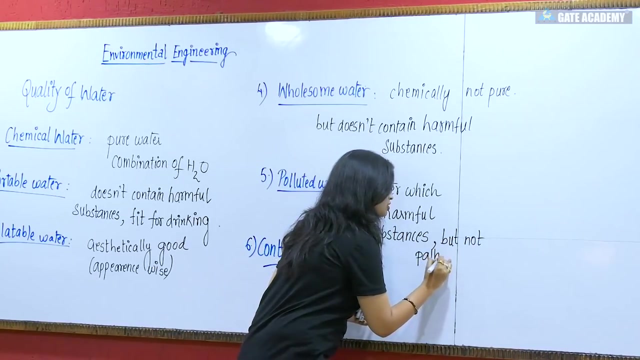 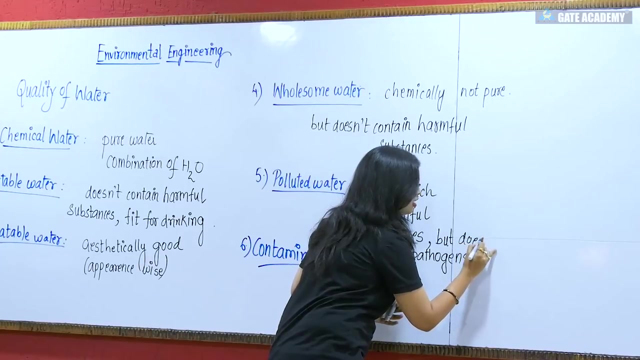 Contaminated water water. Contaminated water means water which contains pathogens. one more thing: when we talk about polluted water, water contains harmful substances, but not pathogens. it does not contain pathogens but not pathogens. we can write, but does not contain pathogens. it does not contain pathogens. 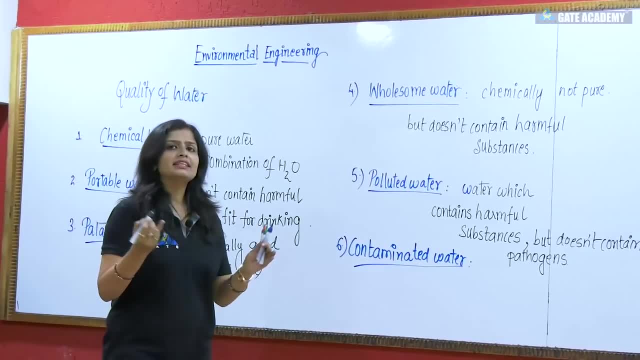 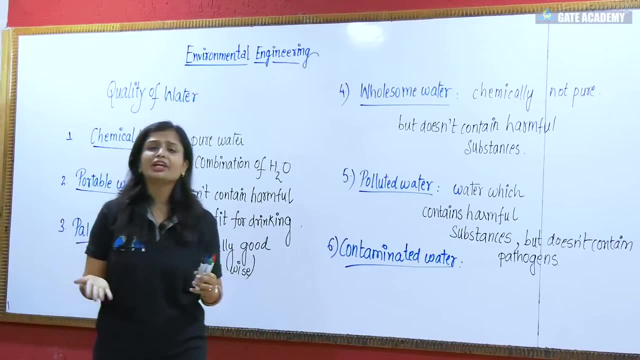 polluted water. but when we talk about contaminated water, like if you say that water has been stored in your cooler for a long time, then you can use that water for drinking purposes- no, because water can be contaminated. this means that water has been stored for a long. 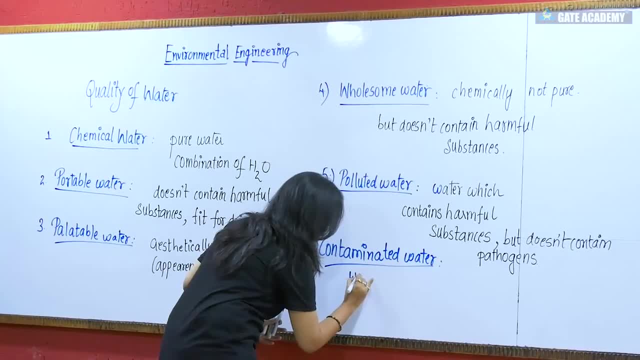 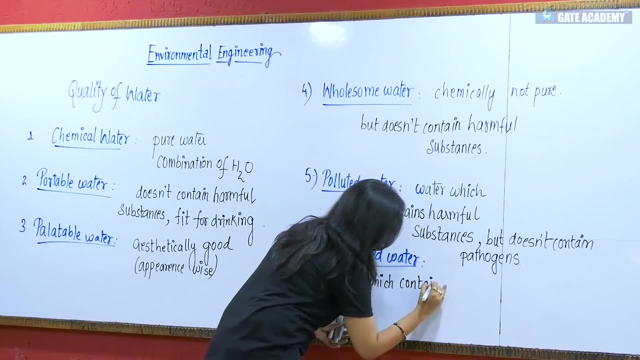 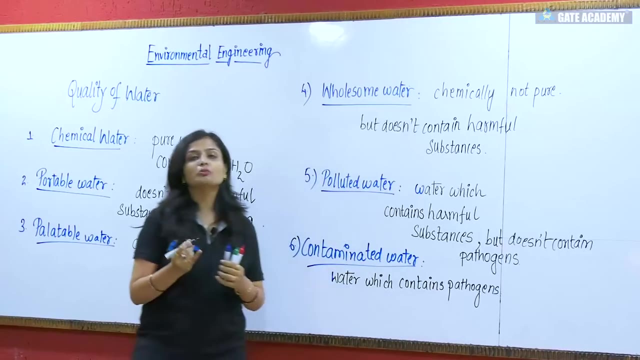 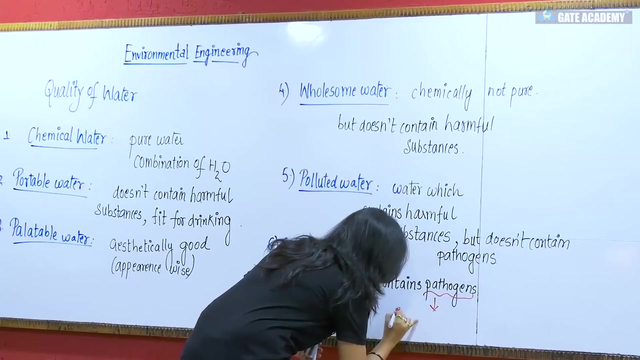 time. so polluted water contains pathogens. polluted water contains pathogens, which contains pathogens. pathogens means, if you ask, what are pathogens, Pathogens are disease causing bacteria, so these pathogens are known as disease causing bacteria. Okay, Okay, Okay. 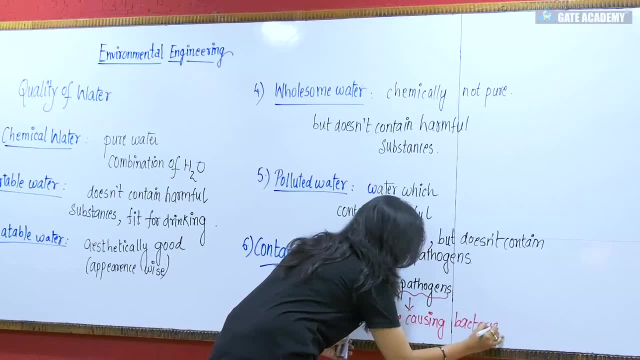 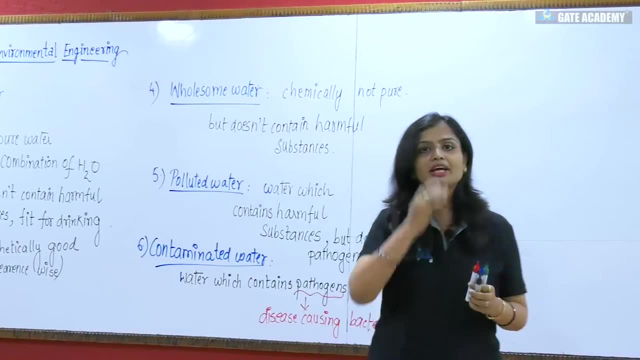 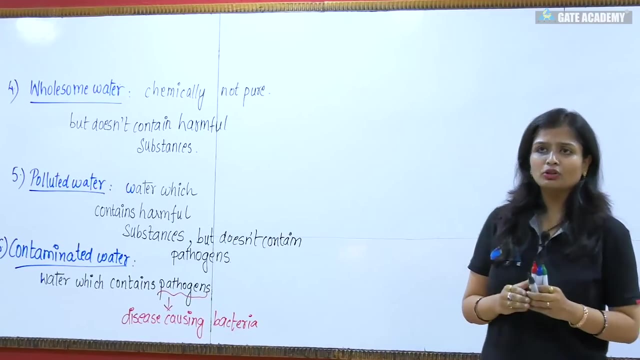 Okay Now the last one is about contaminated water, but apart from this, you must have heard about mineral water. Like the water we drink, we say that it is mineral water. Mineral water means that calcium, iron or other different minerals are present in it. 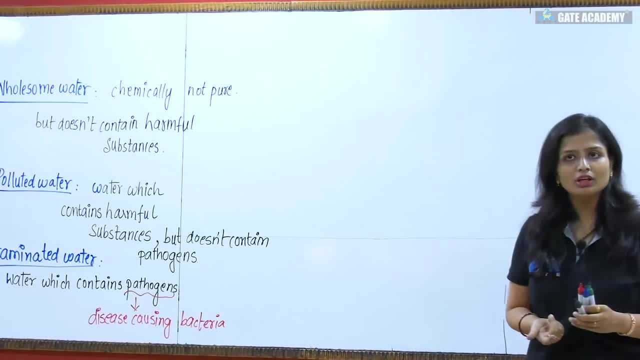 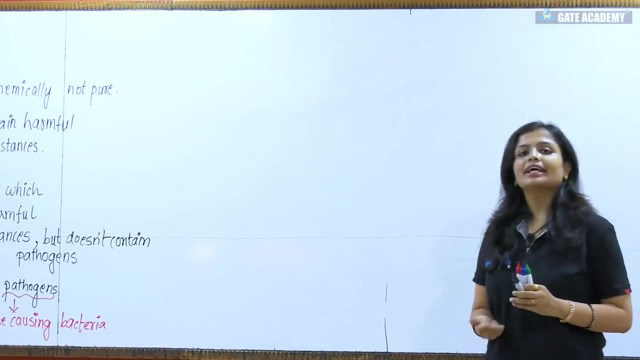 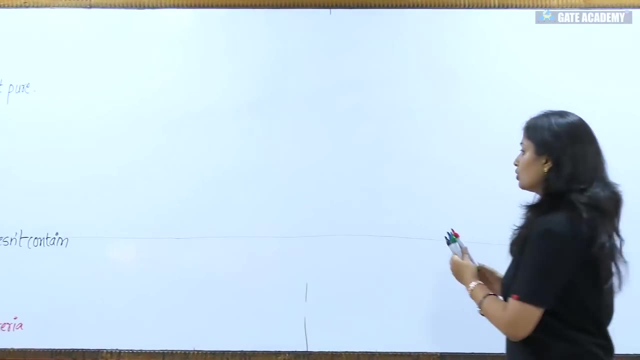 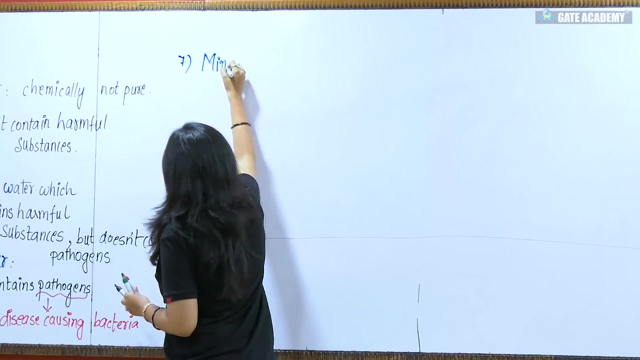 Because our body also needs some amount of minerals, But their amount or content remains in the permissible limit, so that if we consume it, then there should be no water-borne diseases in our body. So the seventh one is the mineral water. 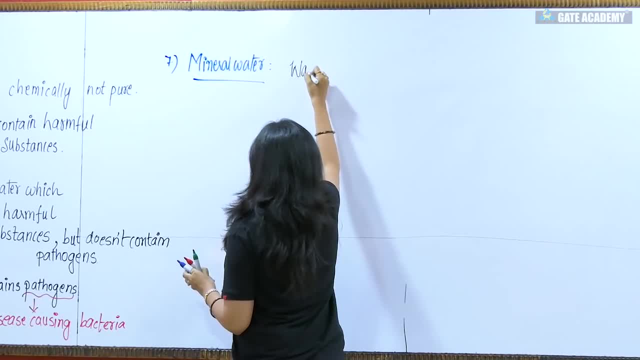 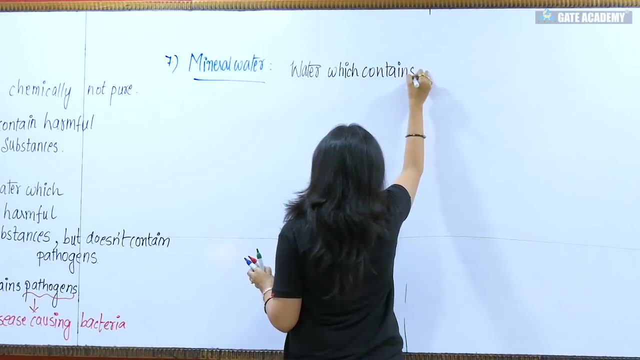 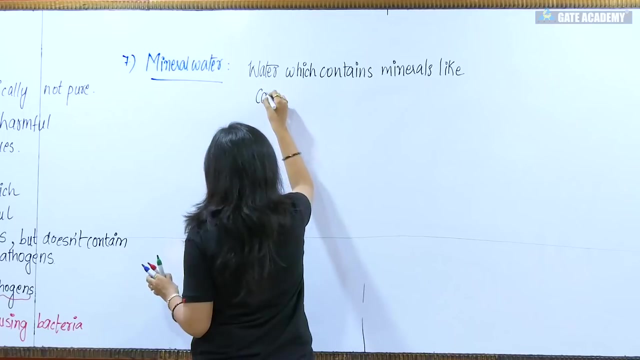 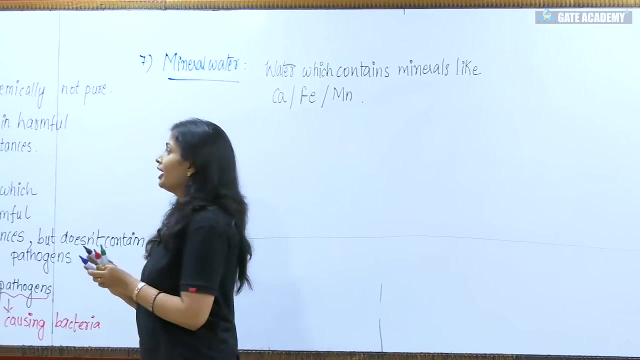 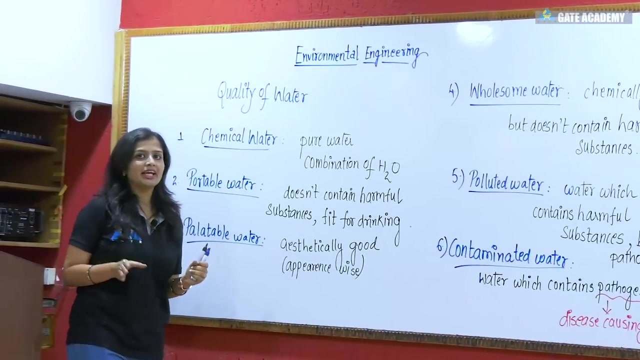 Mineral water means water which contains minerals, Which contains minerals, Minerals like calcium, iron, manganese, Any mineral which is present up to the permissible limit. So these were the different types of water. Let's quickly revise it, Because the basic aim is that you should feel that we are in the classroom. 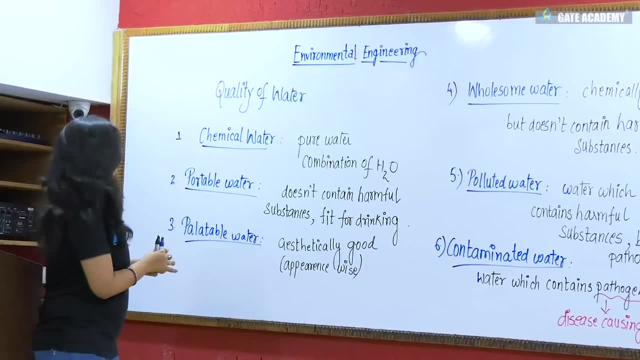 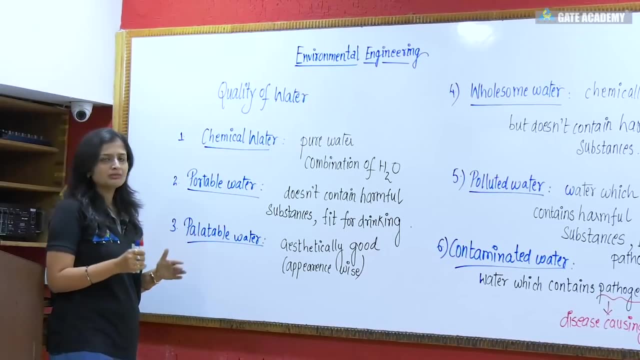 And you have to quickly remember it with me, Fine, So let's quickly see what chemical water is. It is pure water. It is a combination of H2O, That is, H plus ions and OH minus ions. Second, we talk about potable water. 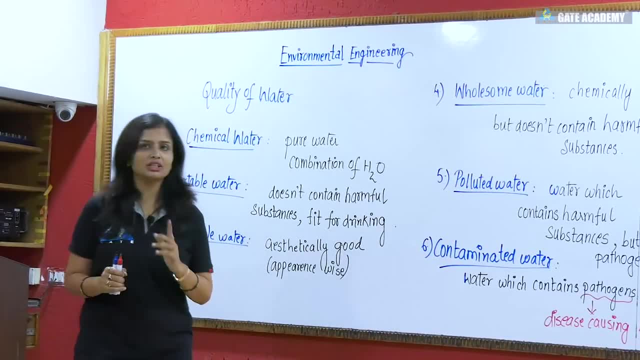 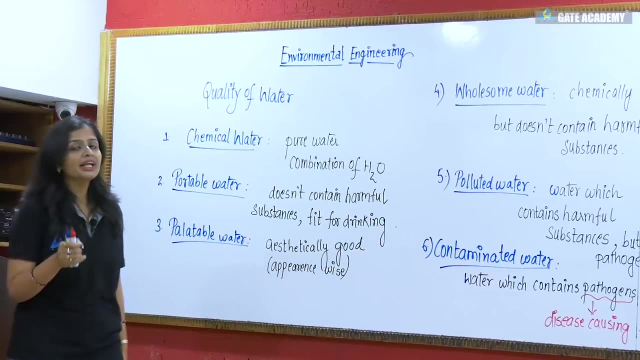 There are no harmful substances present in it. You can consume it- Potable water. Talking about palatable water: palatable means it looks good aesthetically, But it is not necessary that it is not harmful for us to drink. Okay. 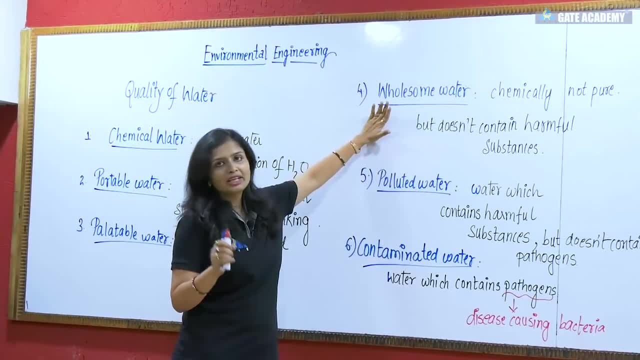 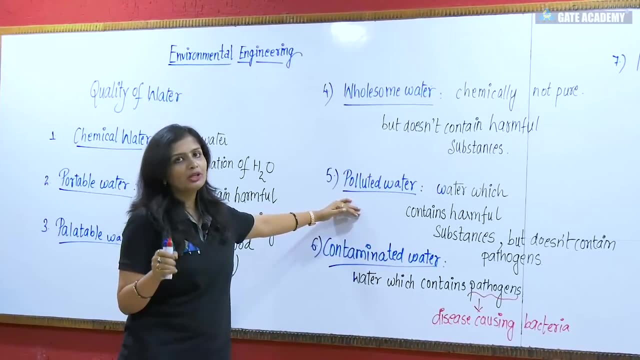 After that we talk about wholesome water. Wholesome water is not chemically pure like chemical water, But there are no harmful substances present in it. Fine, Talking about polluted water. Polluted means harmful substances, But you remember that polluted means harmful substances. 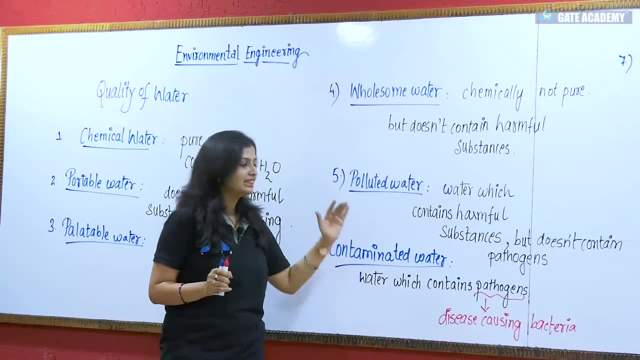 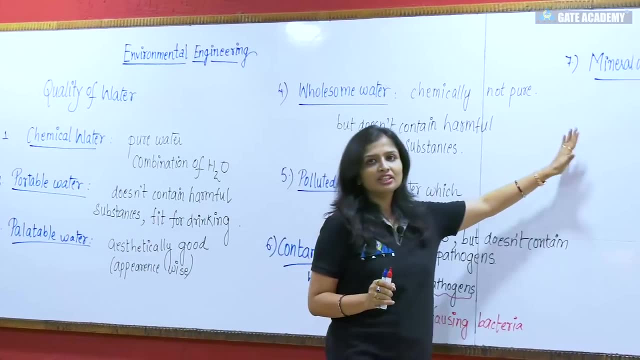 But there are no pathogens. What are pathogens When we talk about contaminated water, And what are pathogens? They are disease-causing bacteria. Now coming to the seventh one, That is, the mineral water. What happens when we drink mineral water? 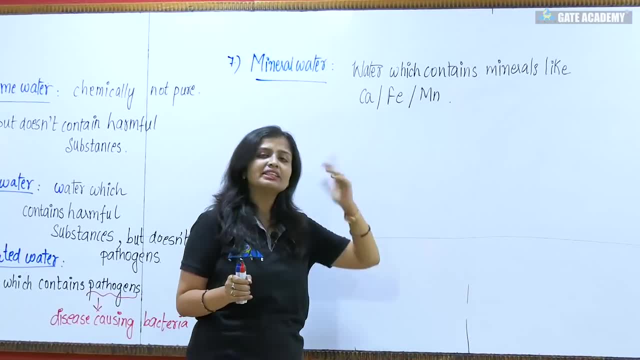 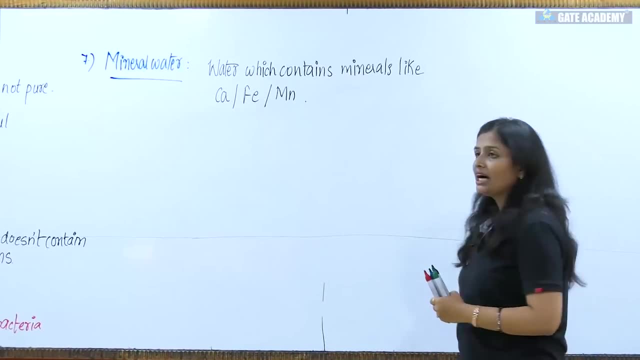 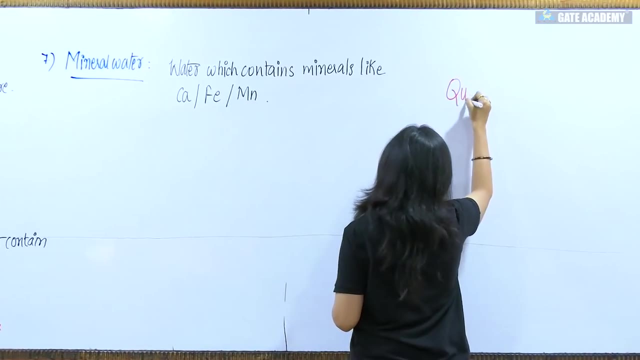 Calcium, iron, magnesium are present in it, But up to the permissible limit. So we have talked about different types of water. Now if we talk about the quality of water, So if we talk about the quality of water, The quality of water. 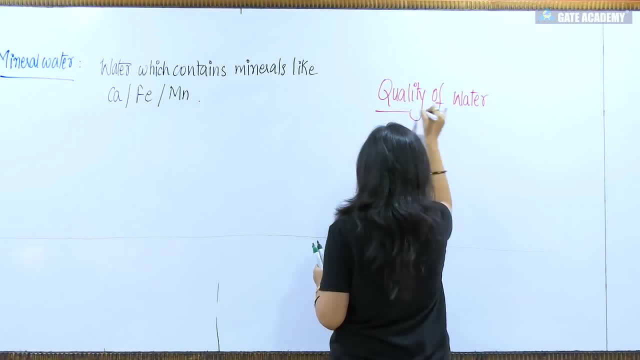 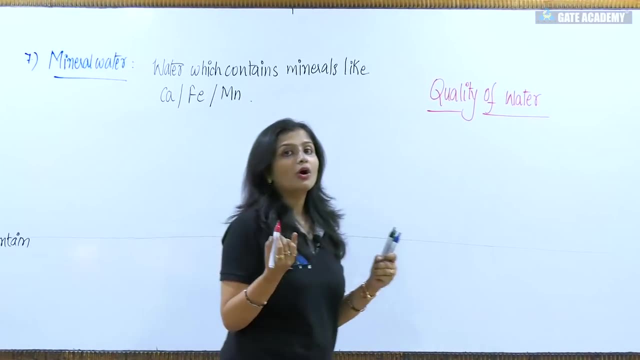 Because water is such a thing. You can live without food for some of the days. Fine, You can live without water. This is a fact. So that is why it is very important for us to study water. So we divide it into three parameters. 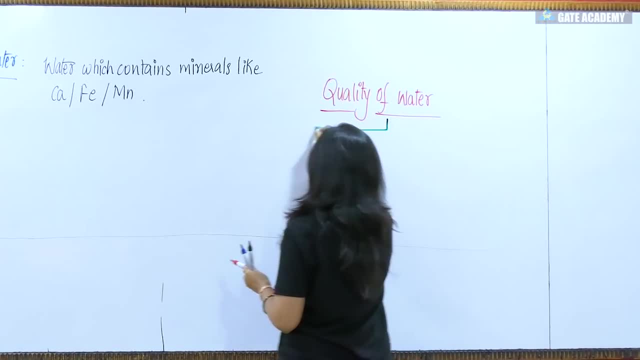 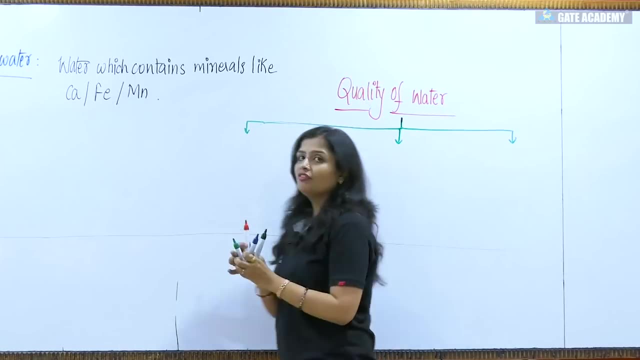 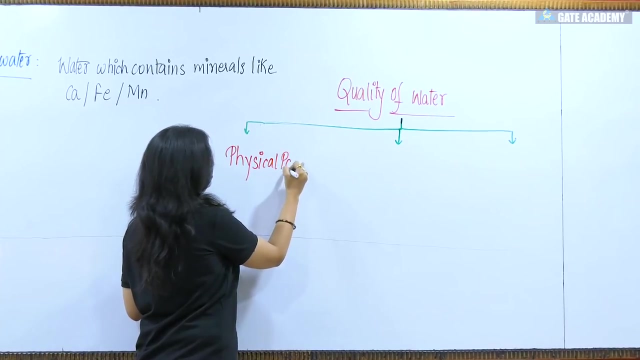 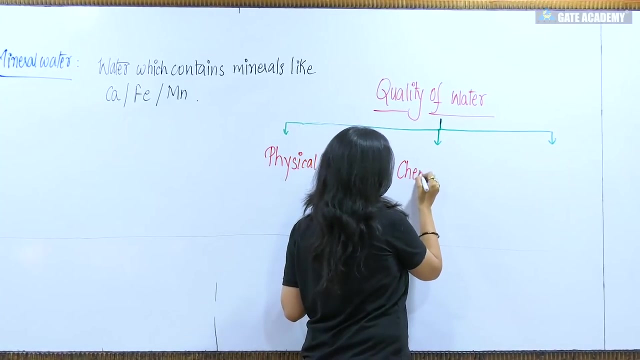 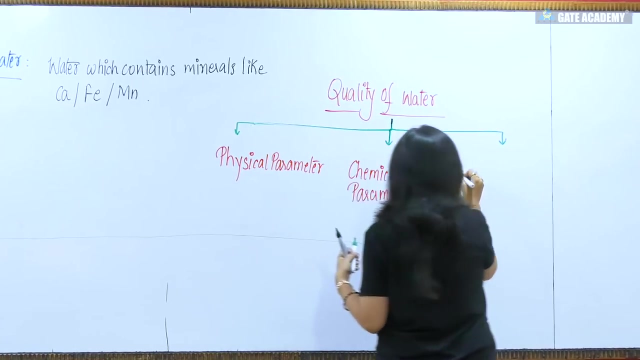 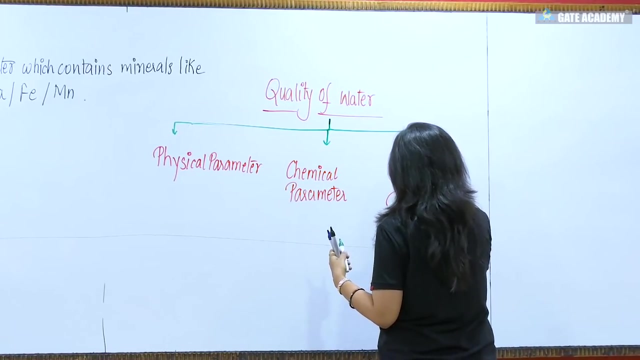 We divide water into three parameters. One is the physical parameter- Physical parameter. Second is the chemical parameter And the last one is our biological parameter. Biological parameters: Now, we will study each one broadly, Like when we study about physical parameters. 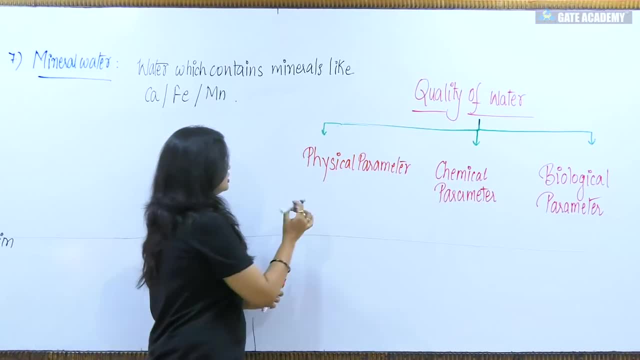 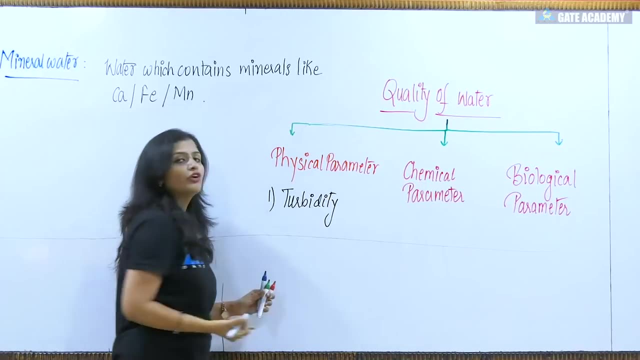 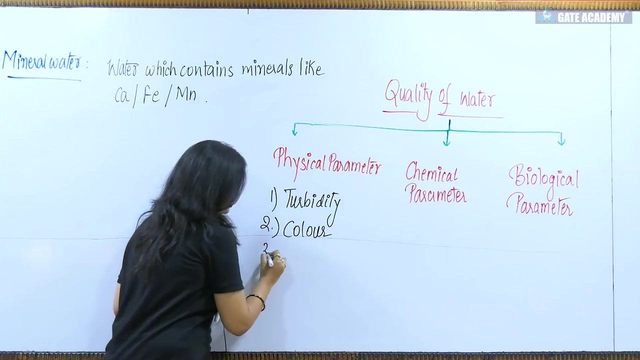 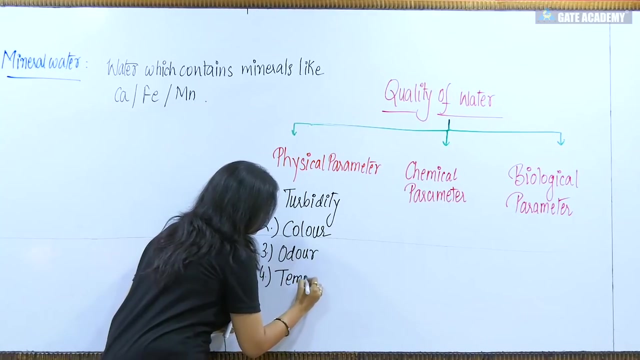 So what are we going to study in physical parameters? First we will be studying turbidity. After this we will be studying how much turbidity there is in water, Then color, Third is odour, Fourth is temperature And the last one is the conductivity. 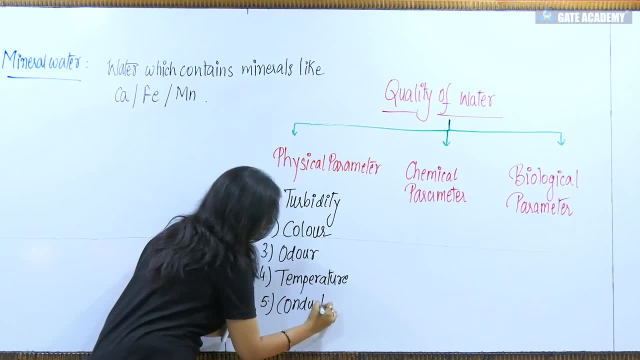 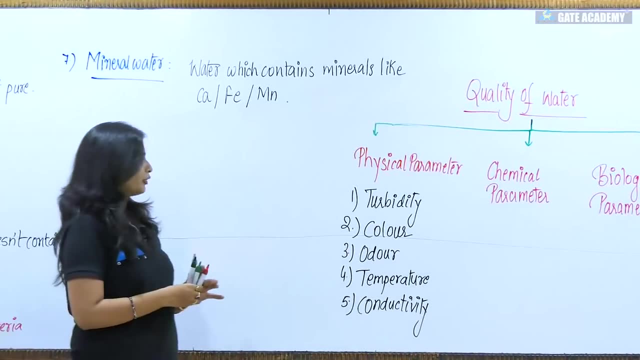 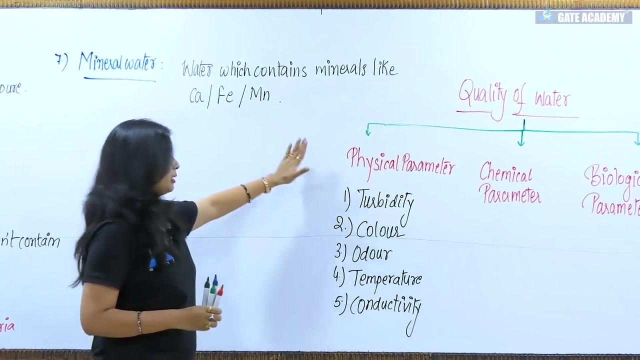 All these are the physical parameters of water About which we will study. well, Fine, So now we have done broad categorization of physical, chemical, biological. There are many parameters in chemical and biological as well, But we will see first physical parameters. 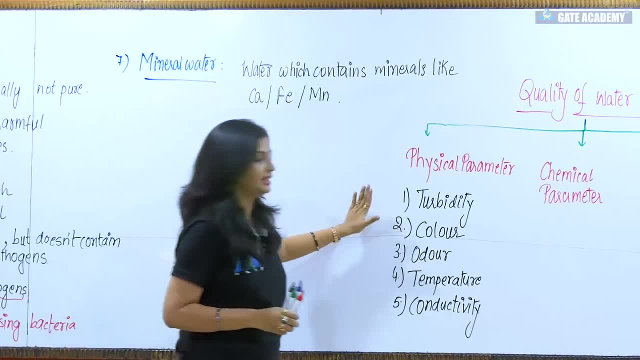 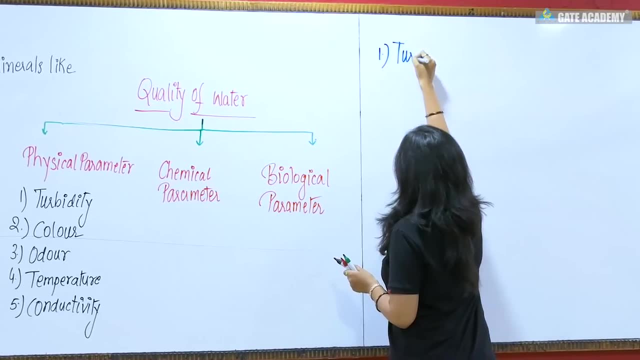 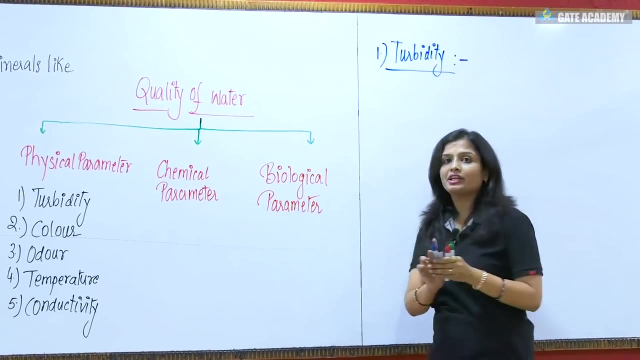 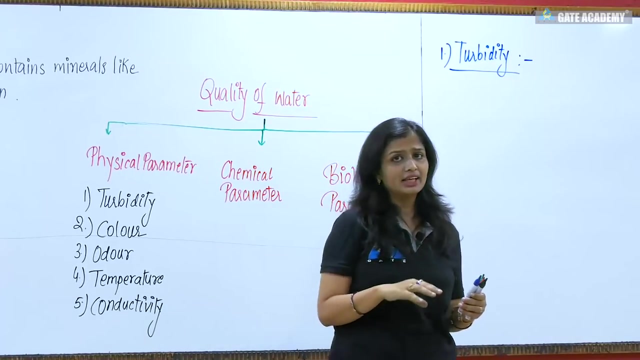 First of all, we will start with turbidity. So now moving to turbidity. Now you have seen the actual turbidity. if you assume that you have a glass of water, you put sand in it, then what are you seeing? that sand is generally not soluble in water. 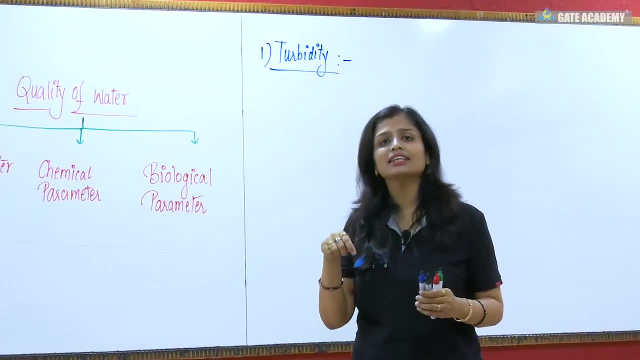 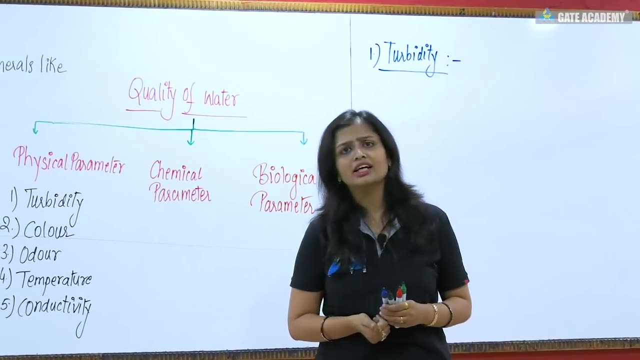 then it becomes sediment. then you, or if you stir it for a while, then you see that sandy deposits are formed in it. the water which is colorless, it looks slightly brown in color. then what do we call it? water is turbid. fine, then. turbidity is generally not harmful. 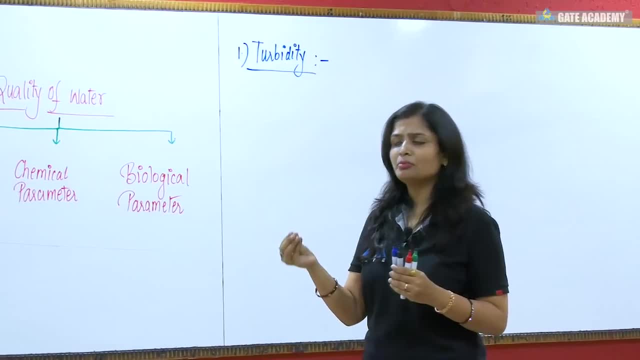 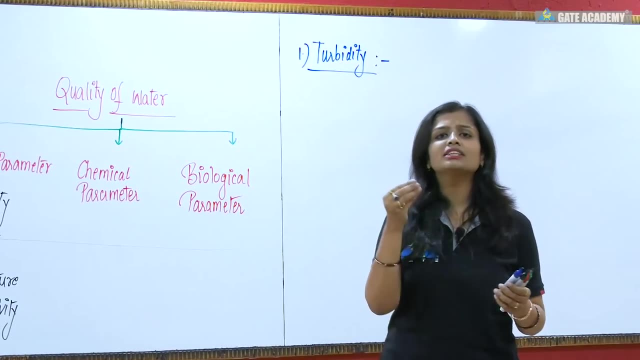 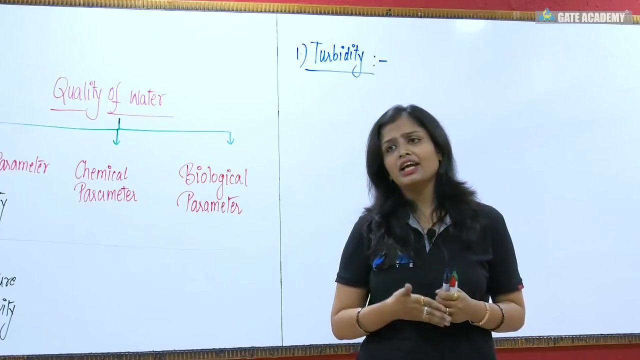 for our body. if turbidity is present in a certain amount, then it may not be harmful for our body. but can you drink that water if you, just for an example, you assume that if in a small amount of water any clay, particle or sand is present, if we digest that amount? 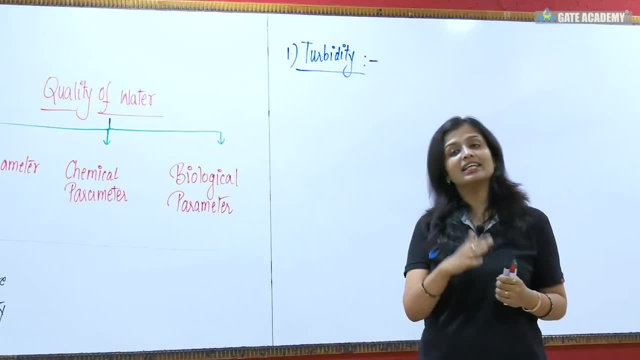 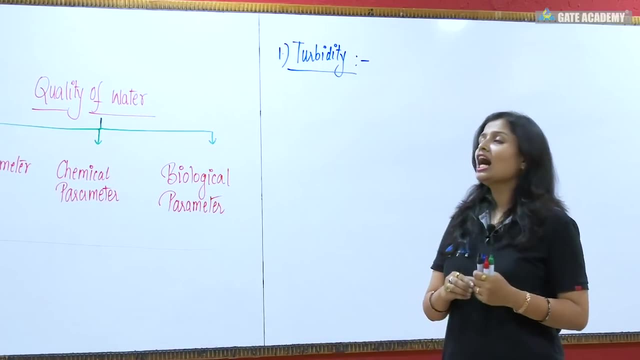 if we consume it, then it is not harmful for us, but still, can you drink it? no, it is not. you will not be able to drink that water because you can see that turbidity with your naked eyes. that is why we should know how to measure the turbidity, and we also have to know this. 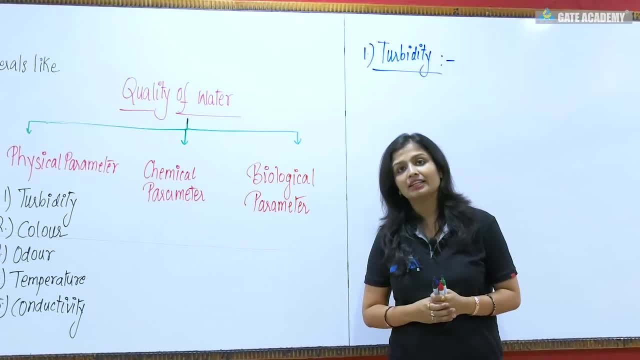 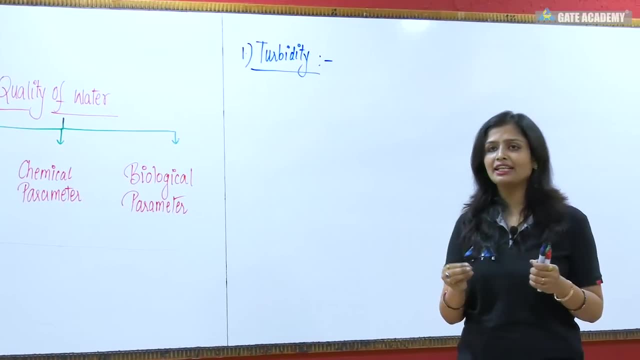 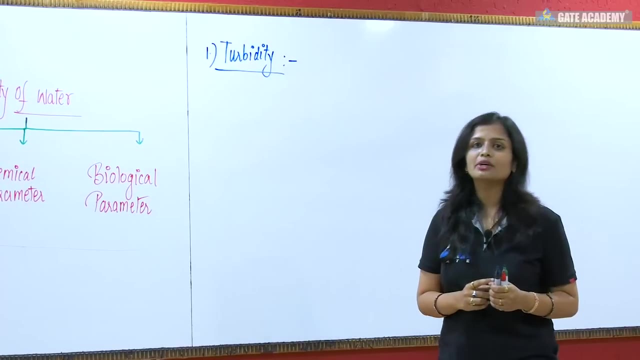 when we talk about the quality of water and all the parameters, then we should know everything because, as per the Indian standard, the Government of India has specified a certain permissible limit for drinking water and it is important for you to remember this permissible limit because it matches the following: 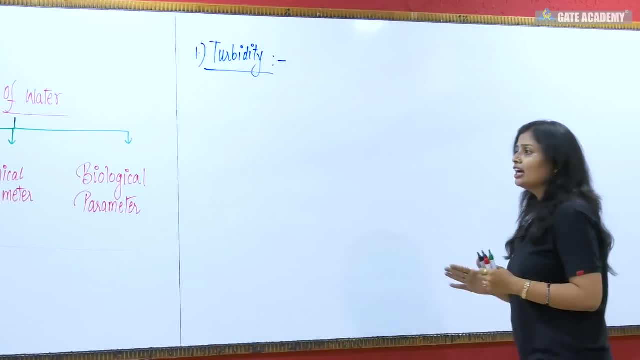 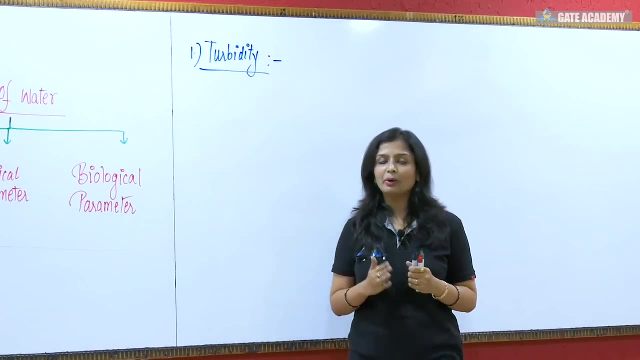 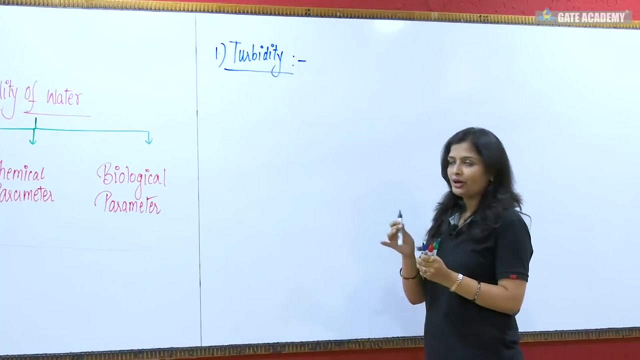 take the correct answers in one marks questions, fine, or because of someone? if? how to measure the turbidity? what are their units? they also ask questions on it, so it is very important for you to read it now. when we talk about turbidity, then I told you that water is turbid if there are many points of turbidity. 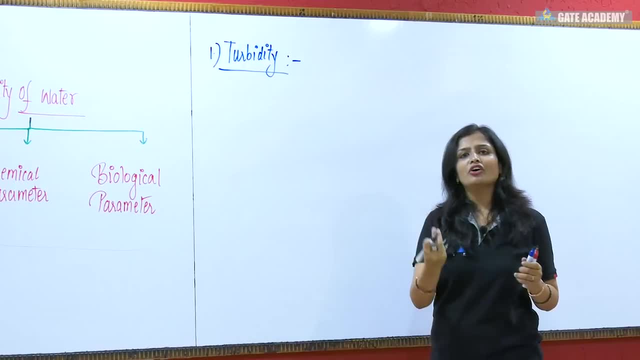 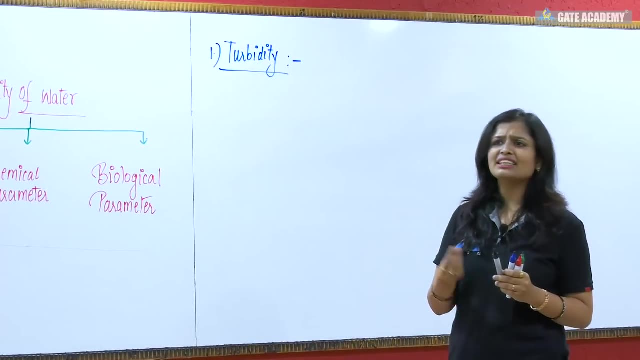 first of all, how do we know the turbidity, any unwanted substance that is present, if any vegetational matter is present, any impurities are present, of sand, rock water, then it is very important to know the turbidity of the water. because it is very important to know the turbidity. 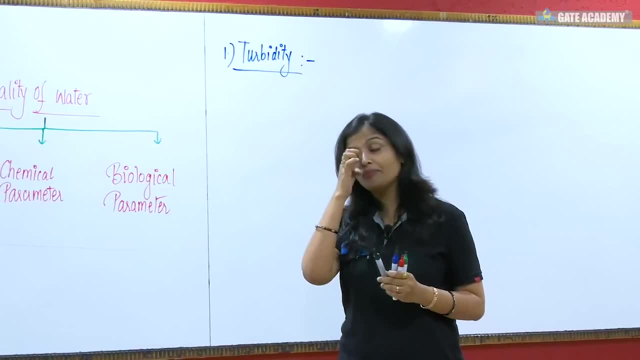 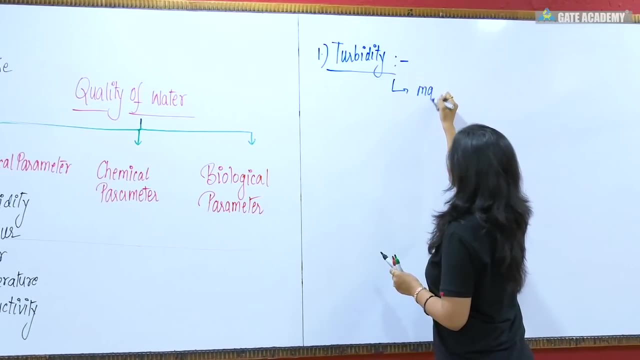 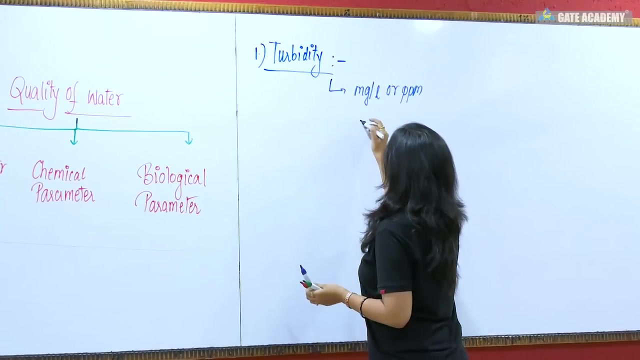 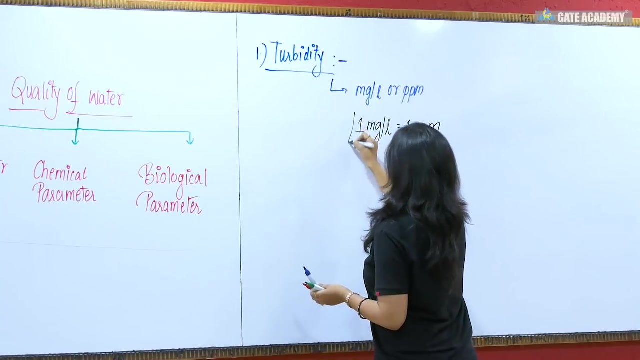 of sand, rock, dust, anything, so we say that water is turbid. apart from this, in which we measure the turbidity, we measure the turbidity on mg per litre or ppm. now remember one thing: that 1 mg per litre is equal to 1 ppm. fine, 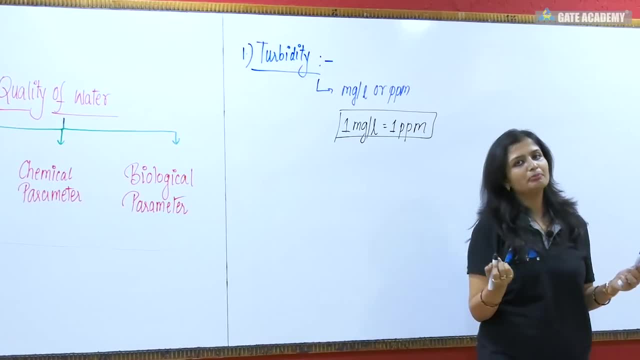 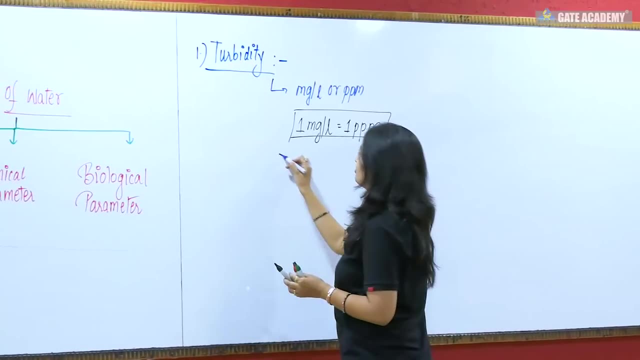 so if ppm is written somewhere, it means that it is mg per litre only. so we came to know one thing: that we measure the turbidity in mg per litre. if the turbidity is more than 5 mg per litre, then you can see it with the naked eye. 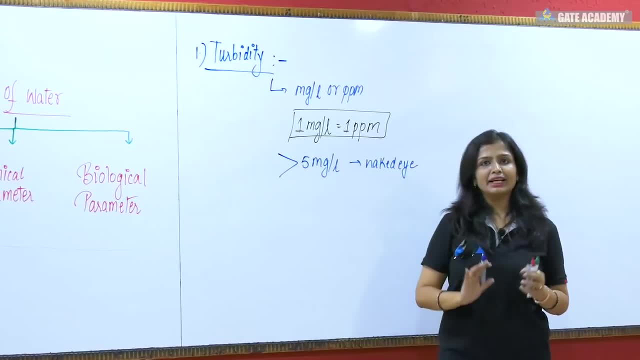 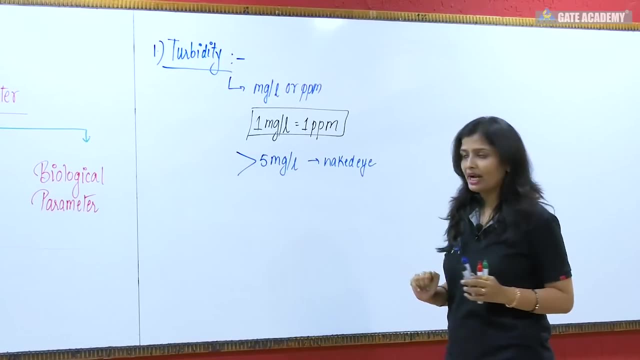 fine, you can see it with the naked eye. then after this one thing also comes that: how much is its permissible limit? how much turbidity is required to us? you should also know this. along with this, you should also know that how do we measure the turbidity? 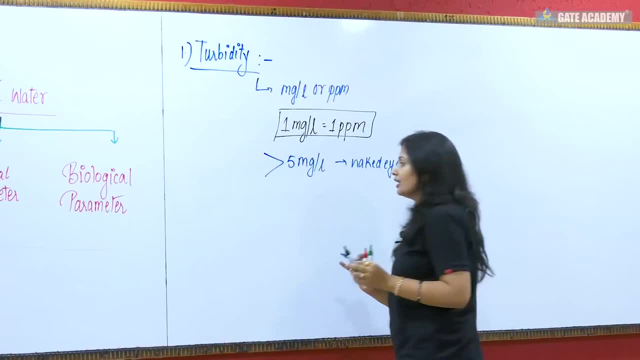 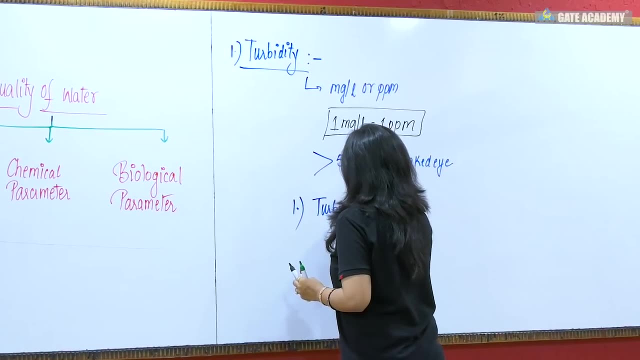 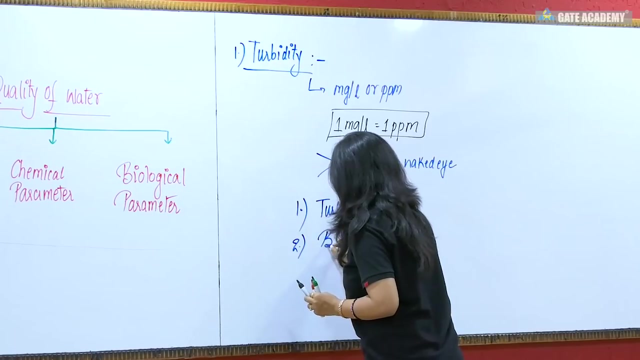 so to measure the turbidity we take 4 different types of instruments like: first, we take the turbidity meter. second, we take the Bayliss turbidity meter. here we call it the turbidity rod. we take the turbidity rod which we use in the field. 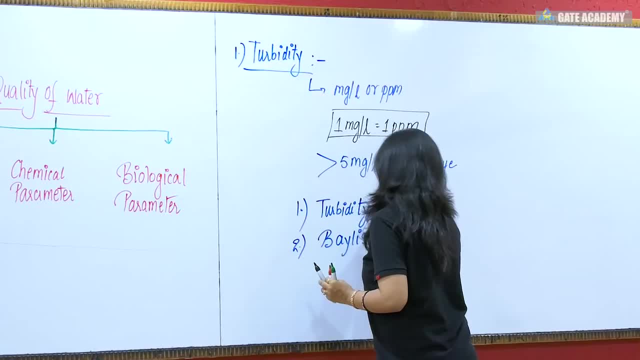 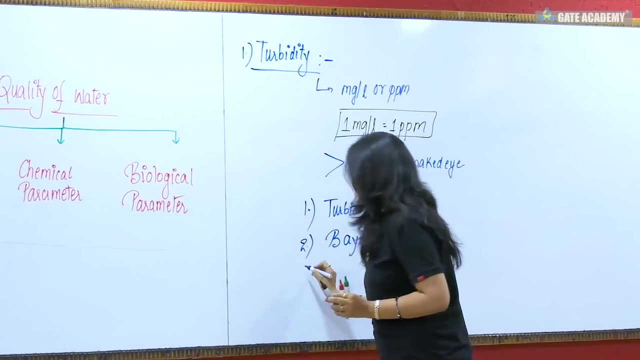 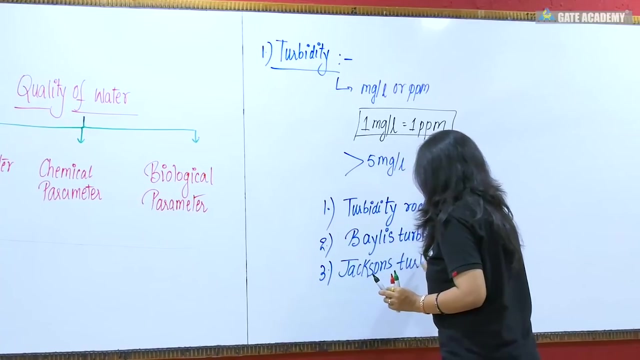 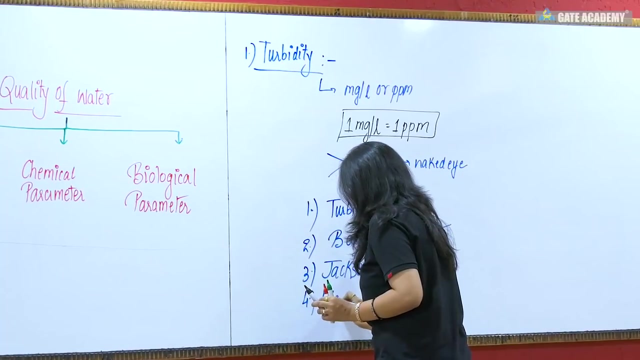 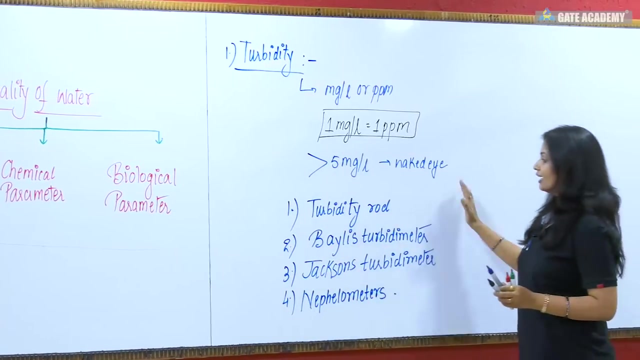 second is our Bayliss turbidity meter. third one is the Jackson's turbidity meter and the last one is the Nephelometric turbidity meter, or we can also call it Nephelometers. fine, so these are 4 different instruments with which you can measure the turbidity. 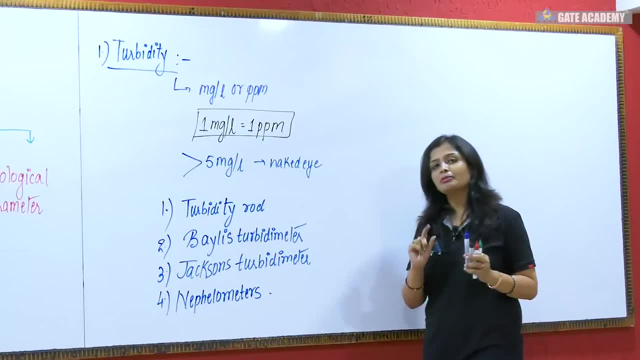 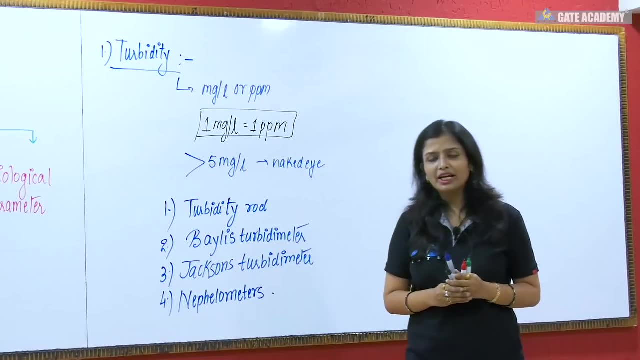 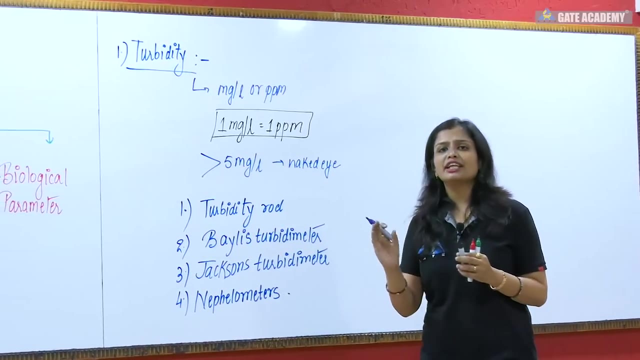 so first of all we talk about the turbidity rod. but before that let me tell you one thing generally: when we talk about the turbidity then we take the silica scale. silica scale means that if we talk about the silica scale then we say that how much mg of silica will be present in 1 litre? 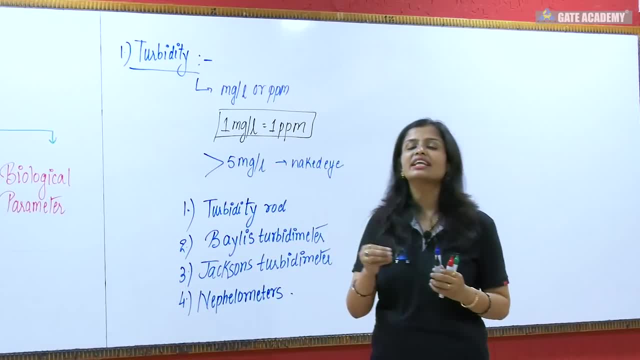 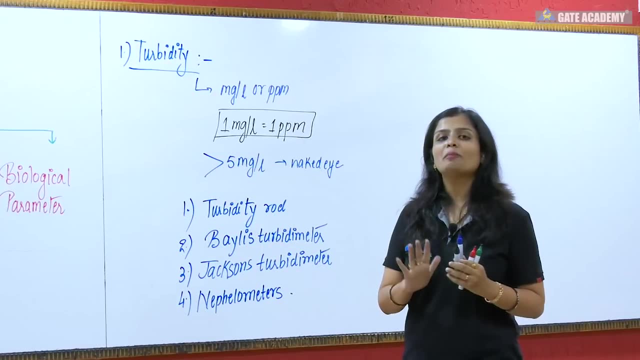 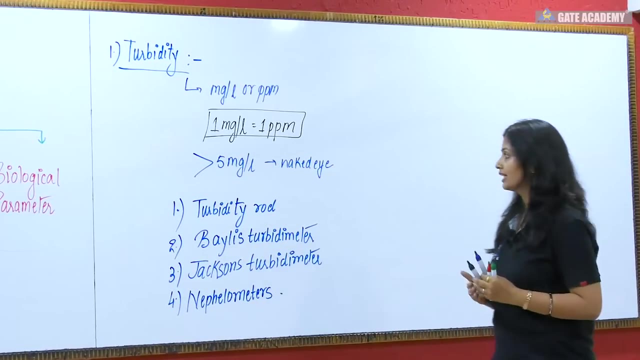 if you talk that there is 5 mg per litre turbidity in silica scale, so this means that the turbidity in the form of silica in 1 litre of water that 5 mg is present. fine, so we generally represent or term the turbidity in terms of the silica scale. 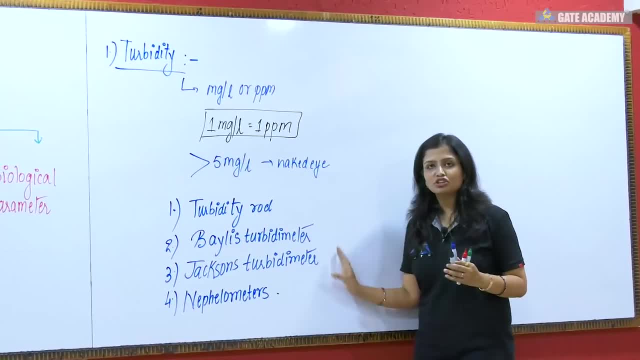 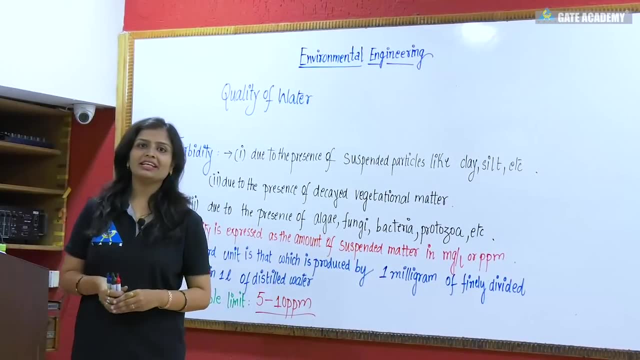 now we will talk about these 4 turbidity meters, or these 4 instruments with which we measure the turbidity. so first we will be dealing with the turbidity rod. now the points which I told you about the turbidity. quickly, just note it down. 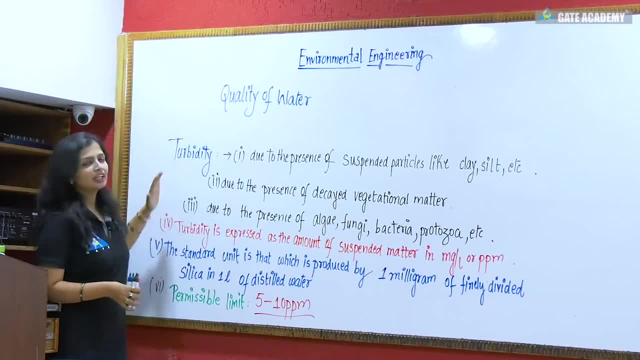 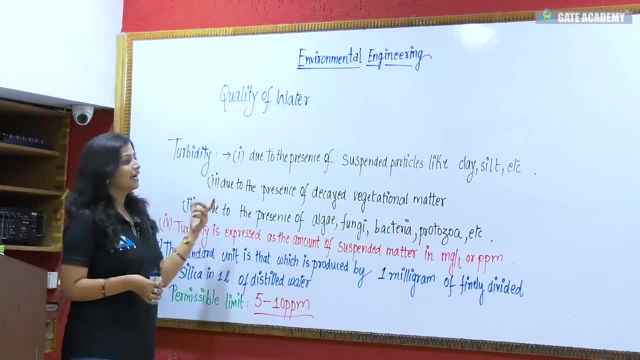 I will read it for you. that is first about the turbidity. why is the turbidity there? the turbidity is there due to the presence of suspended particles like clay, silt, etc. secondly, it is also due to the presence of decayed vegetational matter. 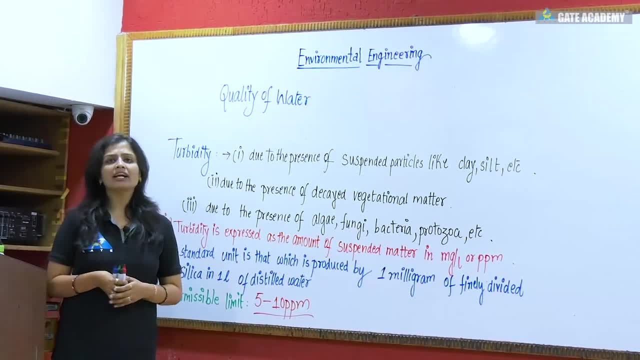 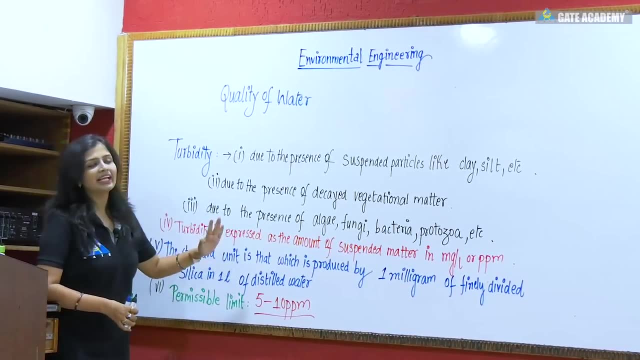 third, if any type of algae, fungi, bacteria is present in the water, then also a certain amount of turbidity is present. after that, if we talk about the turbidity express, then I told you turbidity amount of suspended matters which are present. 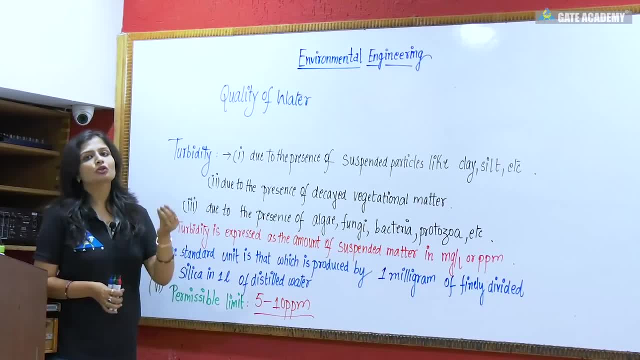 in mg per litre, and ppm means if 2 mg is present in 1 litre, then we will say that turbidity is 2 mg per litre. this is 2 ppm after that, if we talk about it, then in which we measure it. 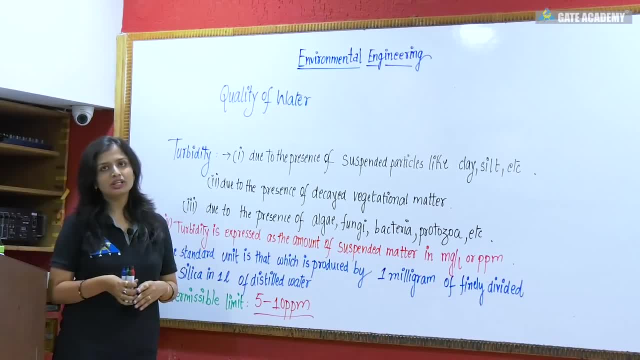 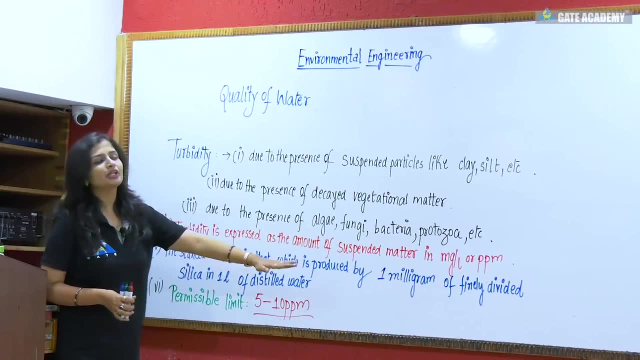 I told you, basically, we take a unit of silica. in terms of that, we take out the turbidity. so what is said here, the standard unit, is that which is produced by 1 mg of finely divided silica in 1 litre of distilled water. 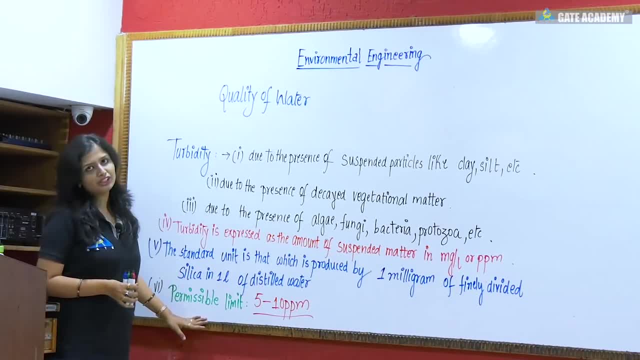 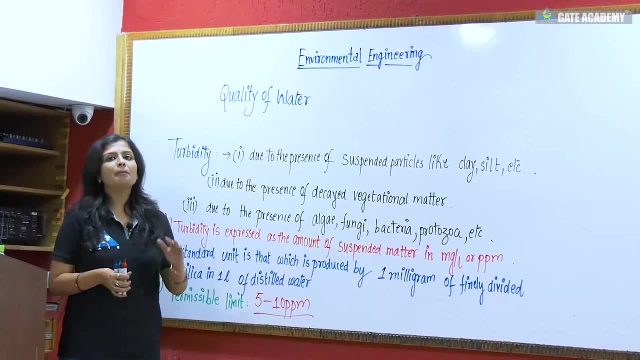 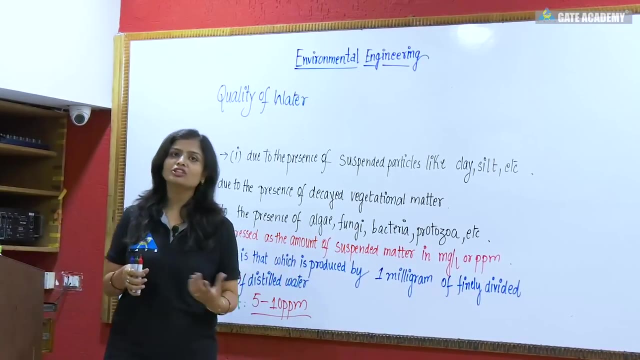 most important, we should know its permissible limit. so permissible limit of turbidity, we can say, is 5 to 10 ppm, means in 1 litre of water 5 to 10 mg of turbidity is allowed for drinking water because if we consume this much amount of turbid water in our body, 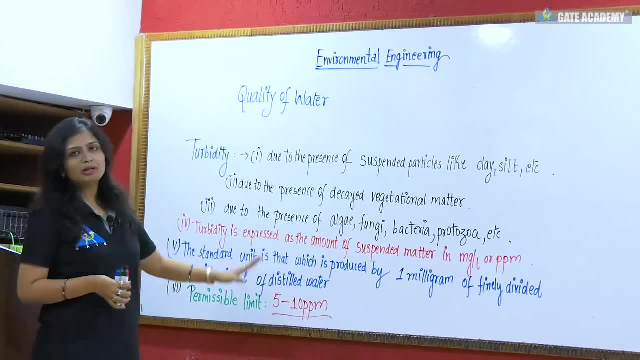 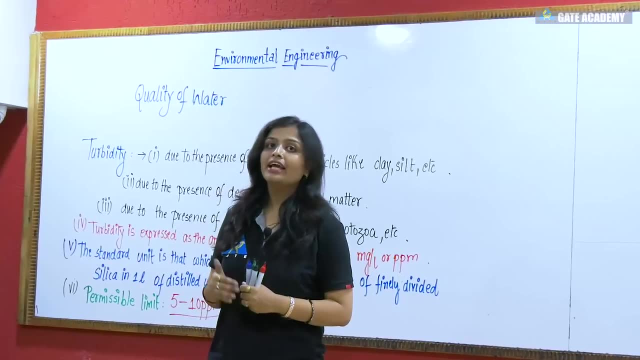 then it will not harm at all. fine, so we talked about the important points of turbidity. now what I told you? that we will study to measure 4 different types of turbidity, its instruments. so first we will deal in it. 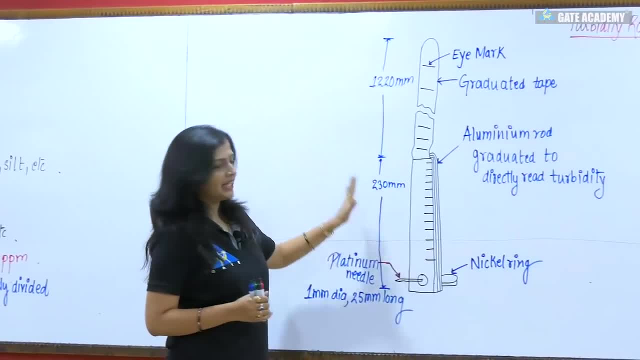 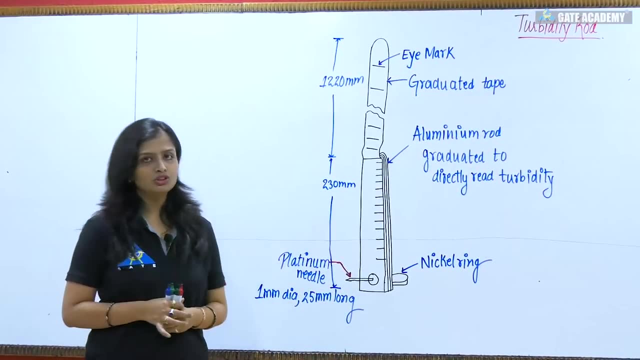 turbidity rod. so I have made this diagram for you of turbidity rod. I will tell you the procedure. you do not need to write the procedure, just the important points. you have to jot it down. first of all, where do we use the turbidity rod? 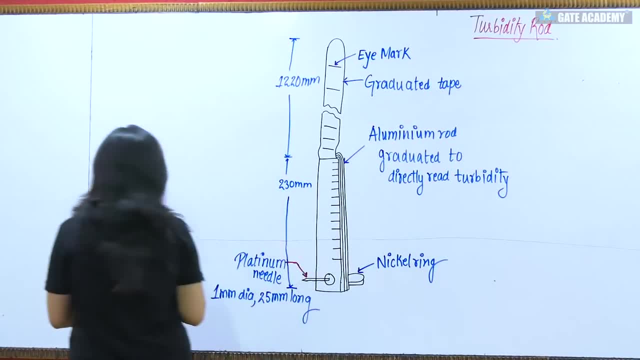 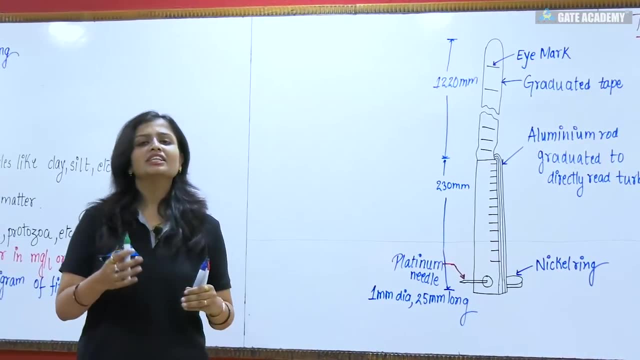 so we use the turbidity rod in the field, if you will be asked, like the Bayliss turbidity meter, the NFLO meter, the Jackson's turbidity meter. generally they are laboratory methods. but if we talk about the turbidity rod, 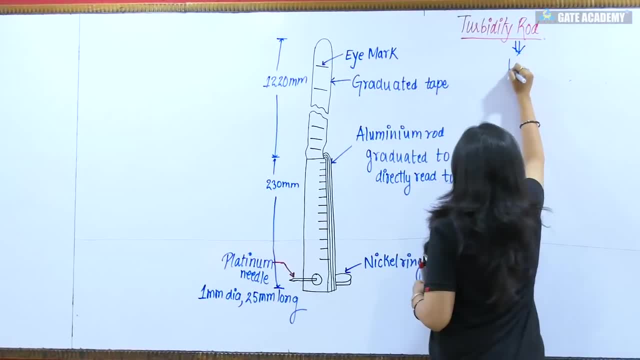 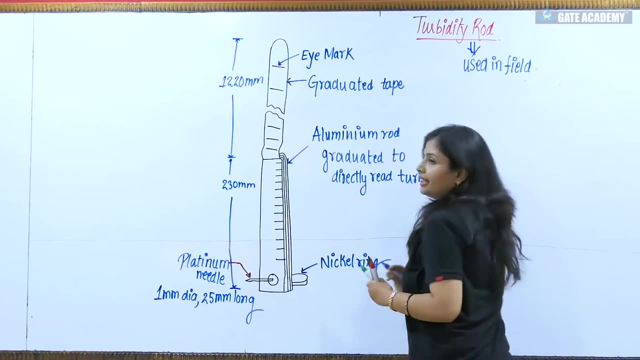 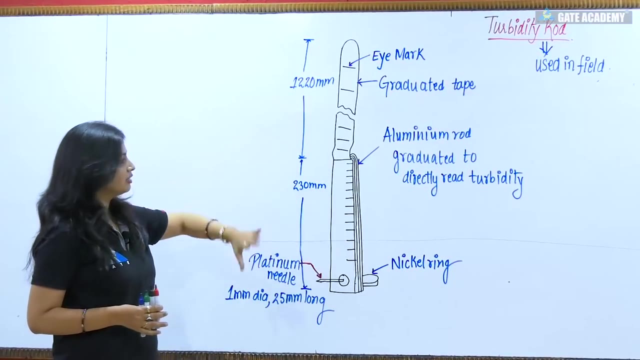 then we can write here used in field. fine, so we use the turbidity rod there now after this. this is the turbidity rod. first I will tell you what are the things in it. first, here is an eye mark. 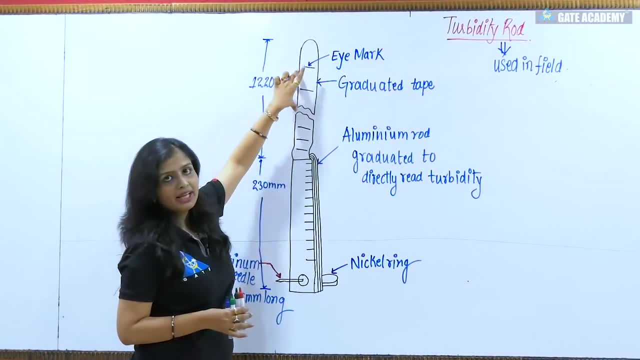 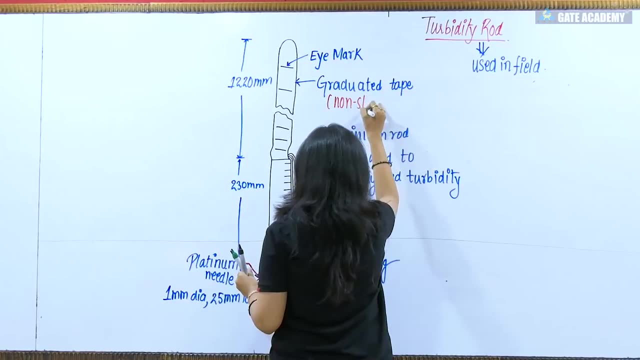 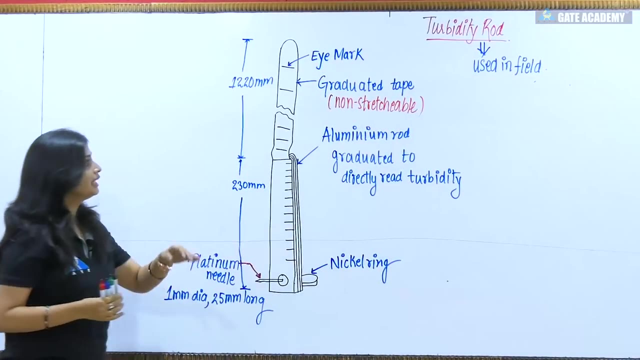 from where you can see graduated tape. this is non-stretchable means you cannot stretch it, so I will write here: non-stretchable, non-stretchable, fine, after this we will talk. this is an aluminum rod. 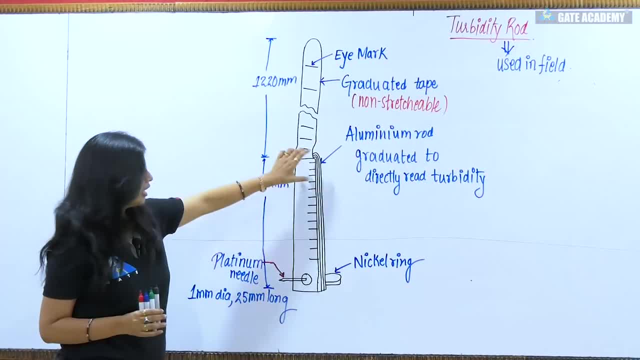 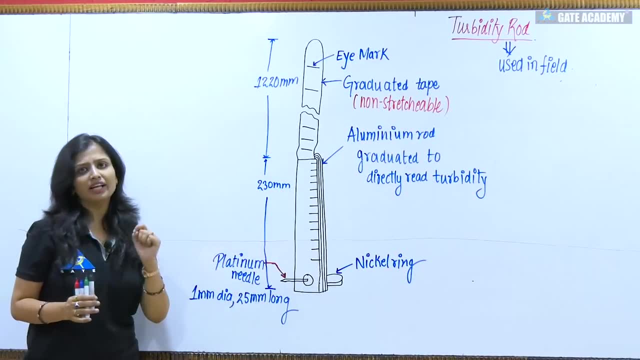 there are graduations made in it. different numberings and markings are given. after this, we have a nickel ring here. then there is a platinum needle whose die is of 1 mm and it is 25 mm long. that is 25 mm long. 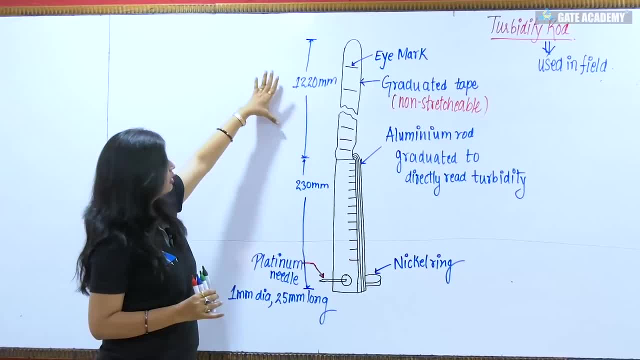 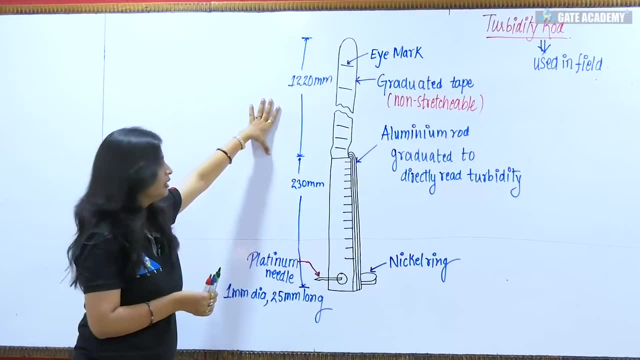 this is your portion of aluminum, which is your eye mark graduated tape. it is 1.220 meter or you can say 1220 mm. after that our portion is 230 mm where the inscriptions of the aluminum rod are given. 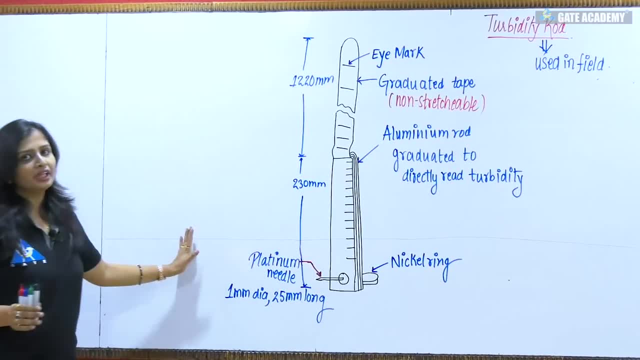 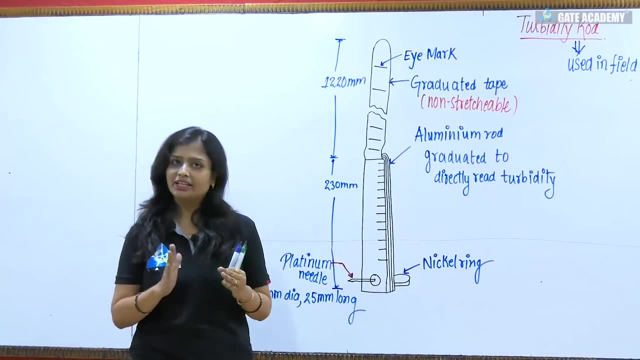 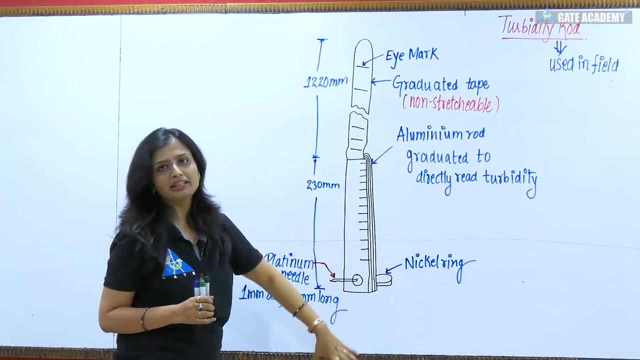 graduations are marked. now listen carefully. how does it proceed? how does it follow the mechanism? first of all, you have a water whose turbidity you have to check. what did you do? hold it and slowly you put it in that water. 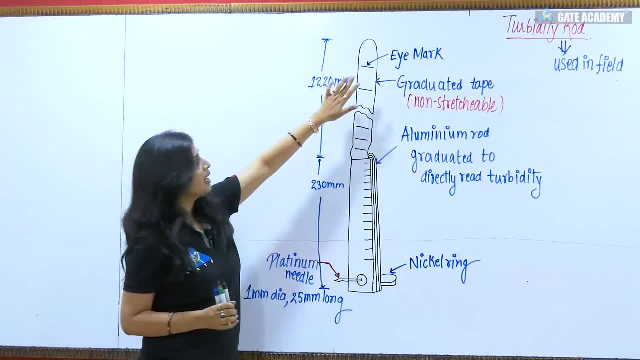 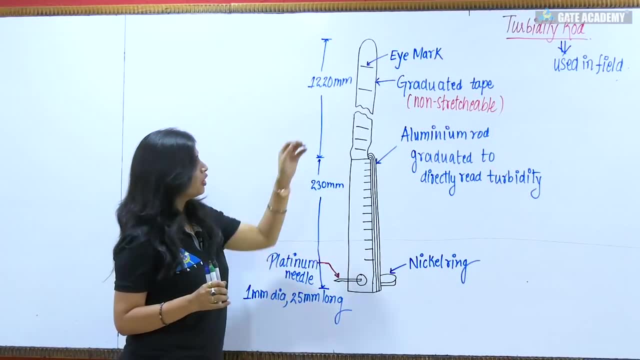 the turbidity of the water. you have to check. this is the eye mark here you will place your eye. then what will happen? you slowly, slowly. you have to see this platinum needle with your eye marks. you have to see this platinum needle slowly. 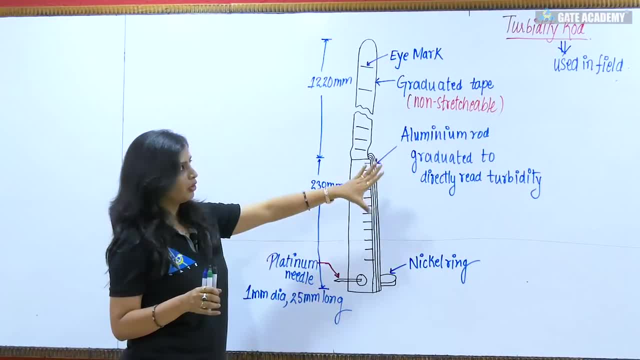 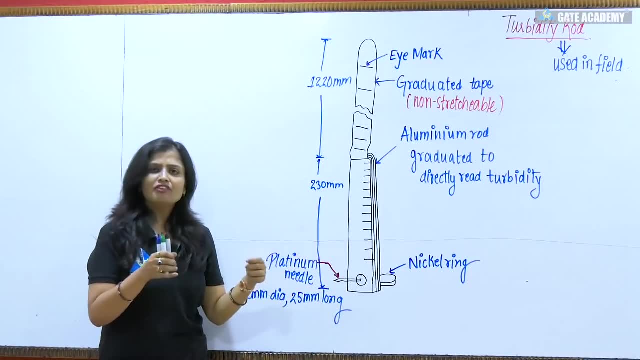 you have to put it slowly in that water, the aluminum rod, this turbidity rod, and you have to see with your eye marks that this platinum needle should be visible to you. then slowly, if the platinum needle is visible to you, 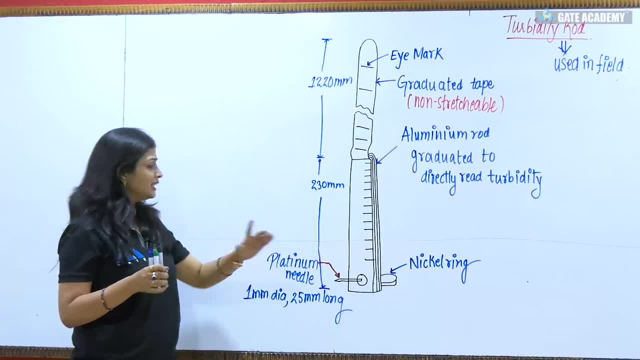 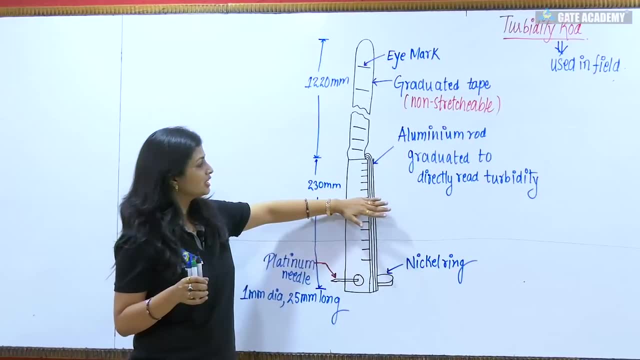 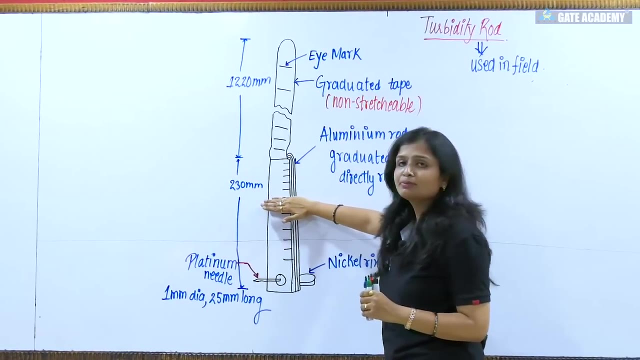 you lower it more in the water, then lower it more at the moment you stop seeing this platinum needle at that moment. here the water surface, just for an example, suppose you reached here, you put it in the water. here you stop seeing the platinum needle in this position. 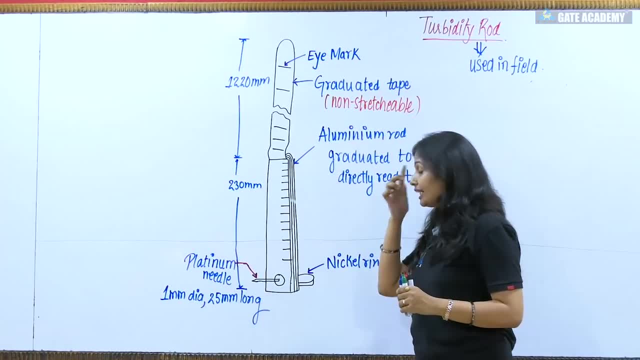 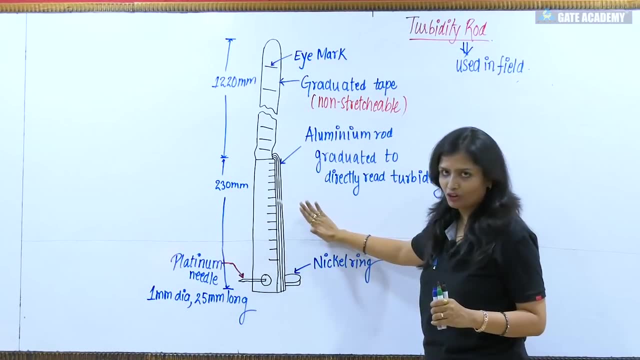 ok, then note the reading of the amount here. it will tell you directly that this much mg per liter of turbidity in the form of silica is present in the water. ok, once again, I am telling you what you have to do. 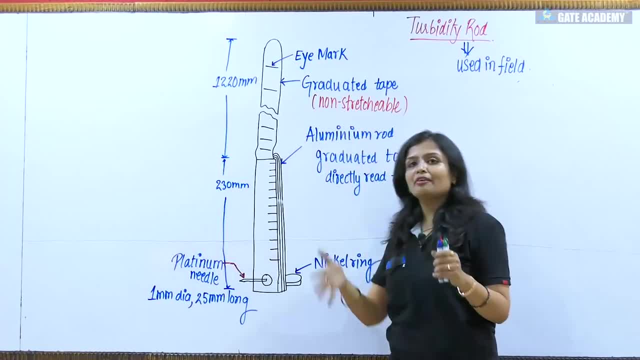 you have to take this turbidity rod, a beaker of water or a liter of distilled water- sorry, a liter of raw water whose turbidity you have to remove. you have to lower it slowly. see the platinum needle with your eye marks. 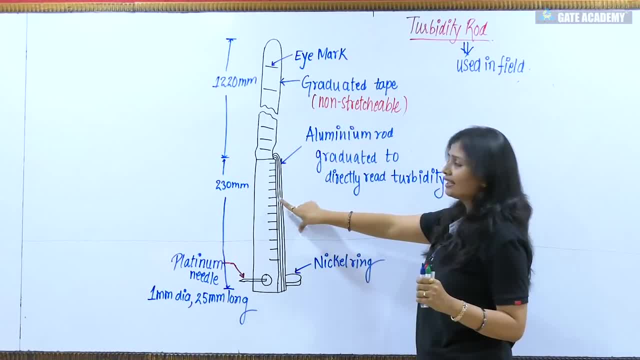 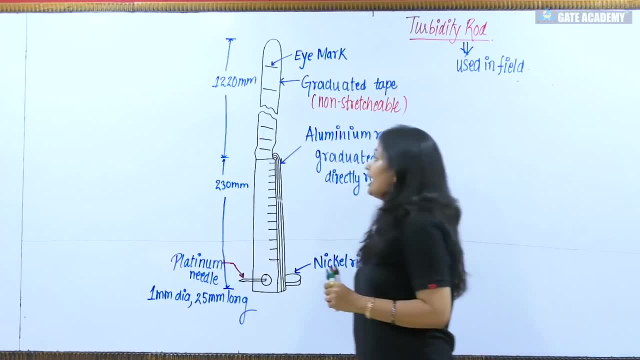 at the moment you do not see the platinum needle. at that moment you are reading directly the aluminum rod in which the graduations are given. you remove it. you will get the turbidity directly in this. you have to remember one thing: 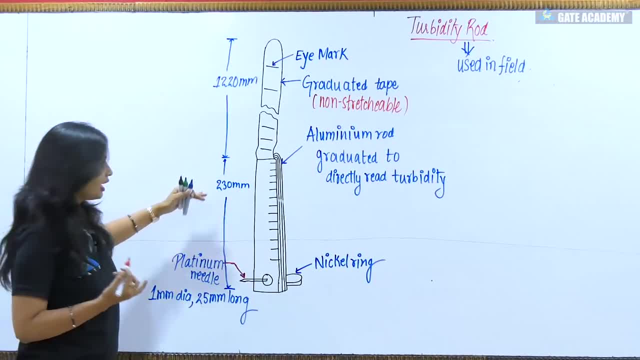 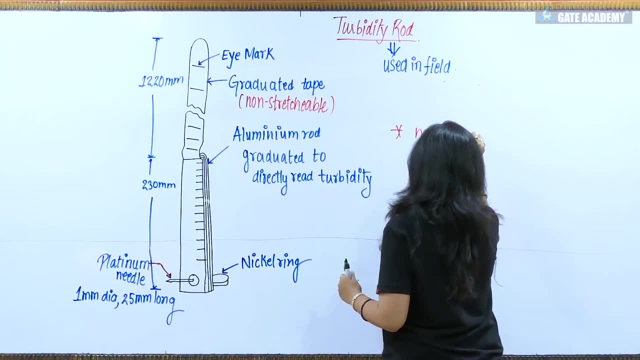 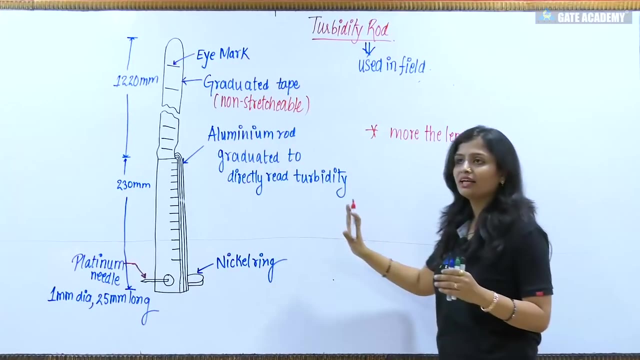 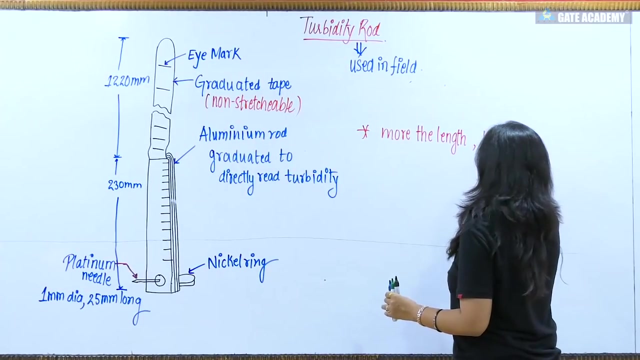 if its length, if its length is more, ok, more the length. if in more length, the more the length. after it goes it is getting the turbidity means you have penetrated more length in the water, then lesser the turbidity. 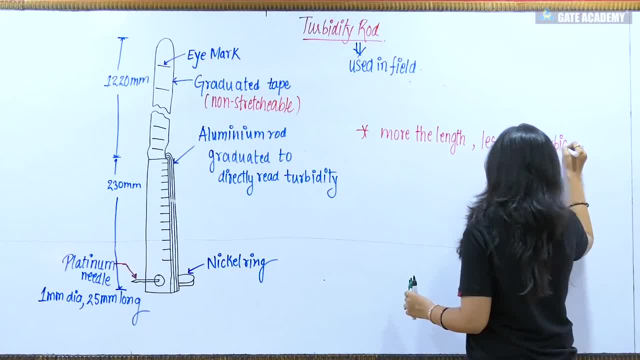 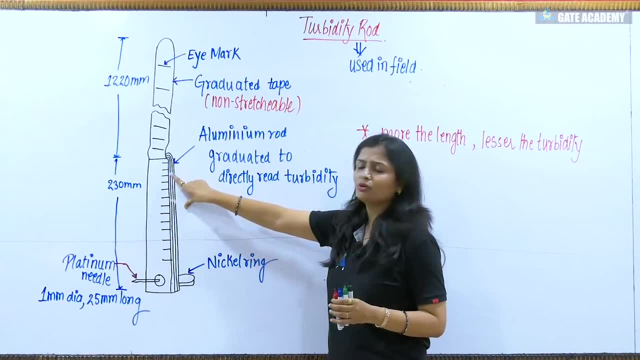 because you were seeing the platinum needle for a long time. if you immediately, immediately, put it in the water and after 2 minutes or a little here, what happens to you? platinum needle gets stopped. it means the water is very much turbid. 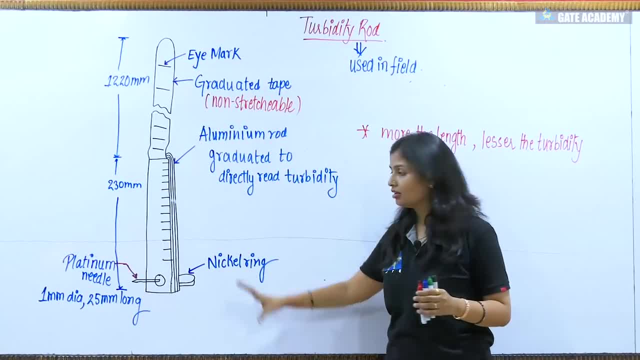 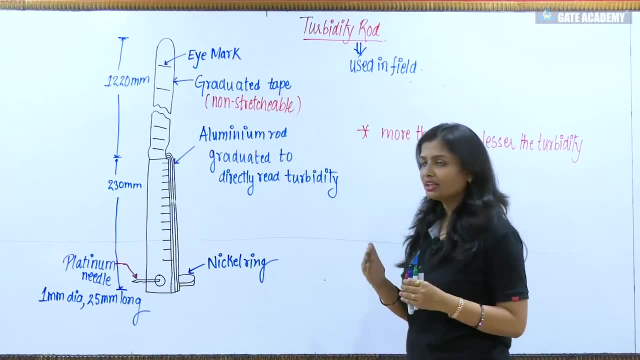 you saw the more length of the aluminum rod. you penetrated the aluminum rod more. after that, at a certain interval of time, you stopped seeing the platinum needle. this means the rod penetrated more length, so more the length, lesser the turbidity. 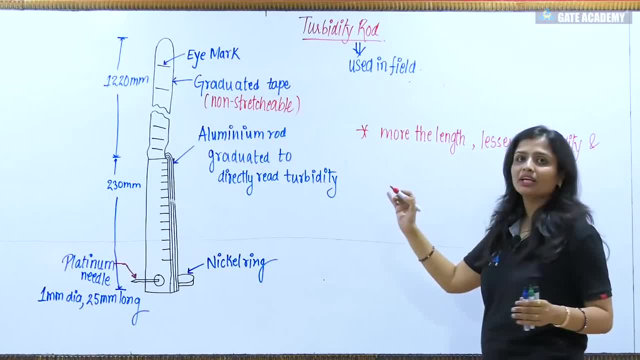 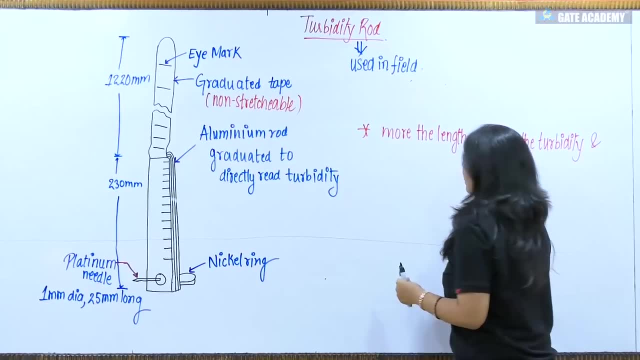 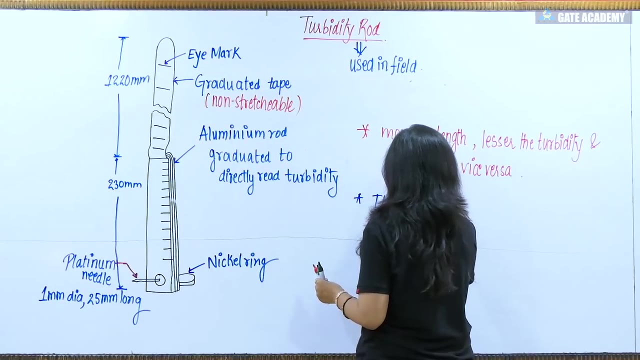 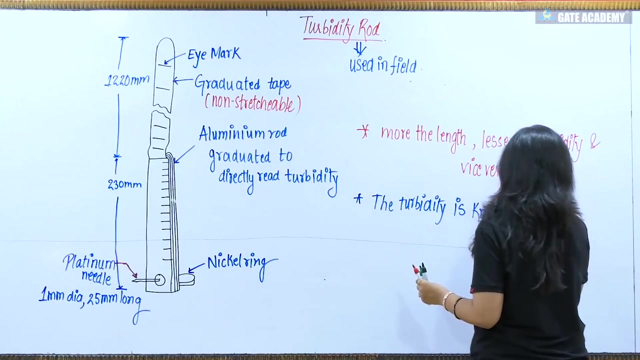 and vice versa. this means if the length is less, then the turbidity will be more, and vice versa. and we can also say that the turbidity is calculated, is known directly. how will we get directly? 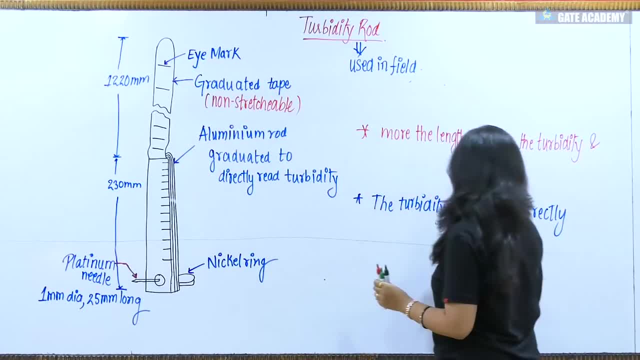 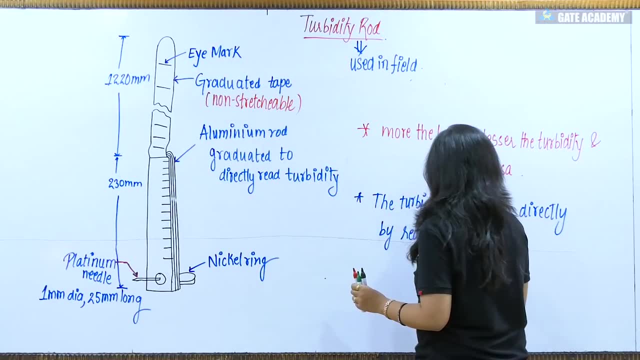 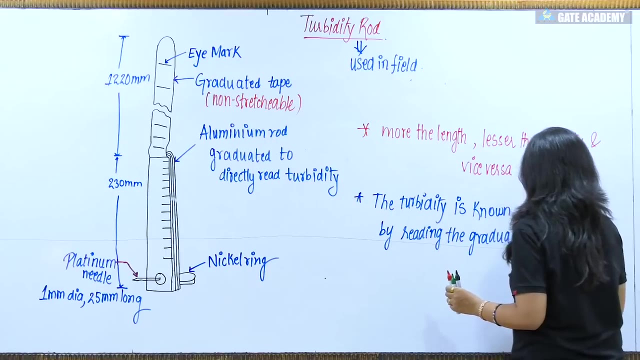 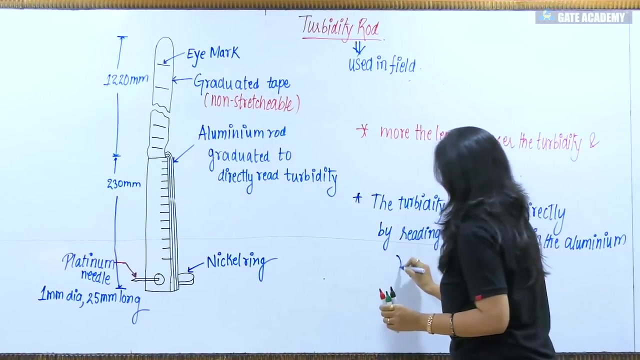 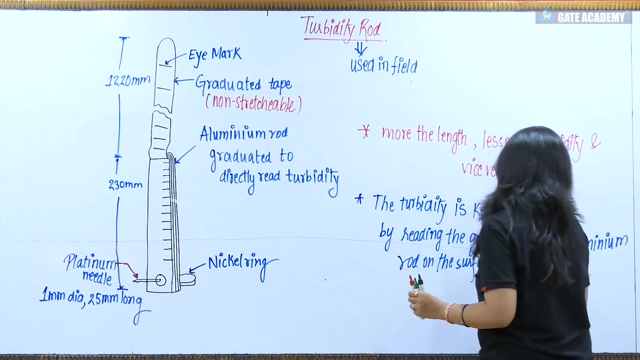 by knowing the graduations of in the water column. the turbidity is known directly by reading the graduation in the aluminum rod, in the aluminum rod on the surface of water column. in the surface of water column You can see how much reading is coming and you can tell directly how much amount of turbidity. 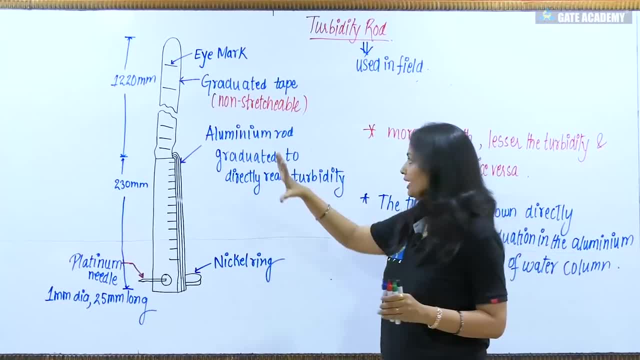 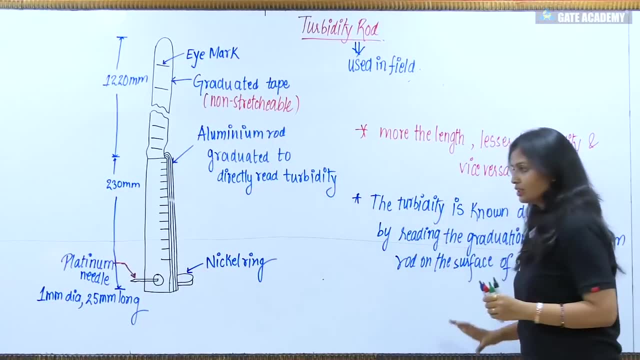 is present, Fine. So this was our turbidity meter. What are the uses in it? You have seen non-stretchable tape, aluminum rod, platinum needle, nickel ring. and what were its uses? Fine, We use the turbidity rod in the field. 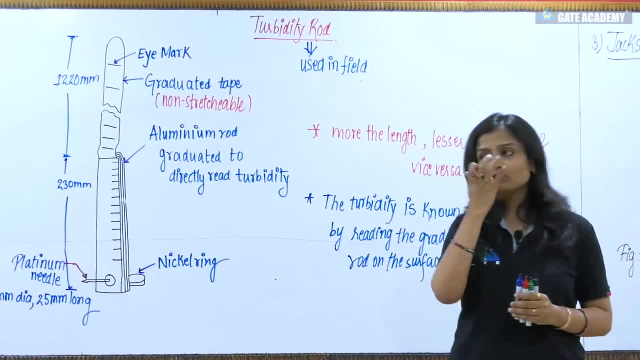 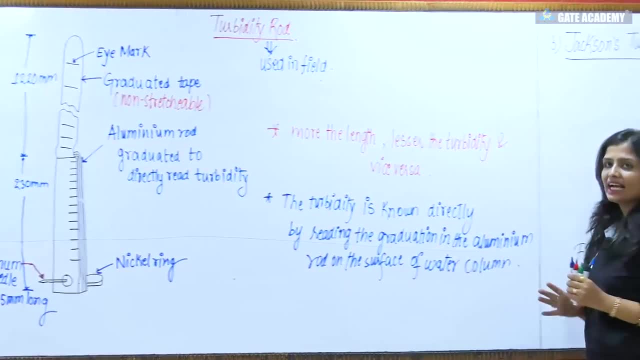 Now when we test the water sample in the laboratory, if the water sample of that area is the source of water, then is it good for consumption or not? In that we will first talk about Jackson's turbidity meter. We will study the Bellis turbidity meter after reading Jackson's turbidity meter, because 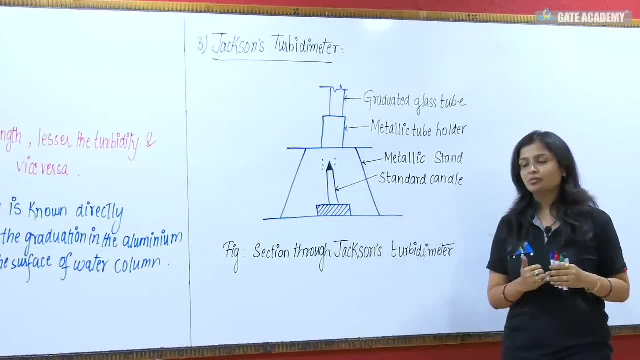 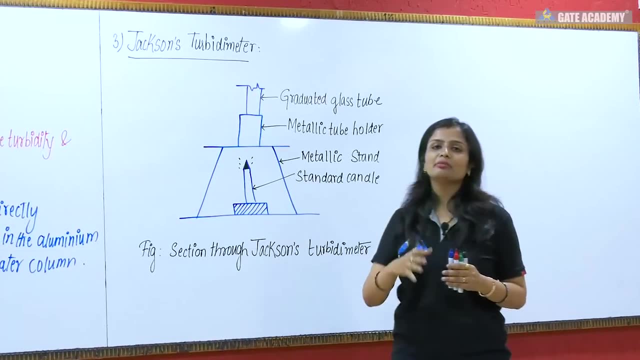 it is an advanced version after the Jackson's turbidity meter. So here I have made the Jackson's turbidity meter. There is a section of Jackson's turbidity meter. You can call it Jackson's turbidity meter, or you can also call it Jackson's candle turbidity. 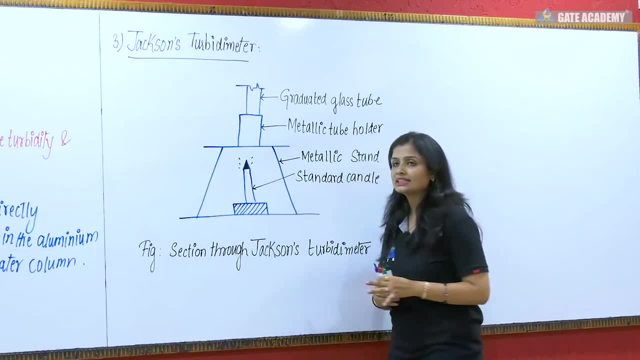 meter. This is a section. Its main procedure is this: What is this? I will tell you, But before that, you can see that this is a metallic tube holder, This is a graduated glass tube, This is a candle and this is a metallic stand. 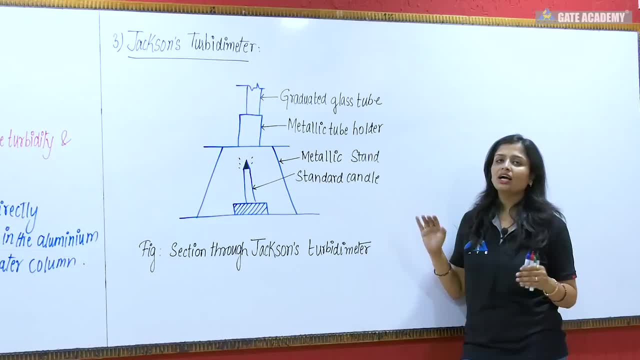 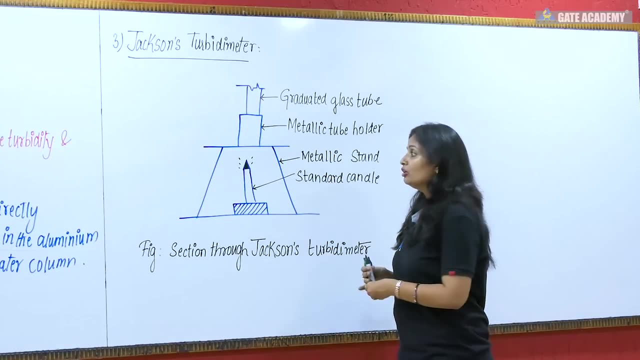 Now, basically, this principle of Jackson's turbidity. the principle of this turbidity is generally based on the principle of scattering of light or absorption of light. So what is the procedure of Jackson's turbidity? I will tell you this. 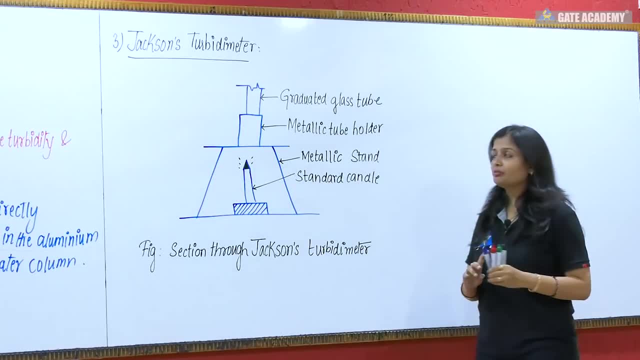 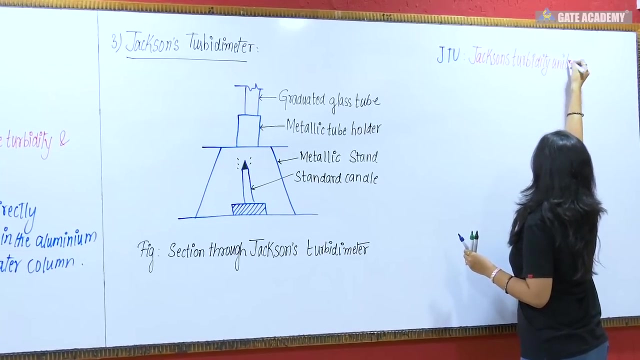 But before that you should be telling that Jackson's turbidity meter has a measurement meter. This is measured by JTU. The full form of JTU is Jackson's turbidity unit, Jackson's turbidity unit. And you should also know that the Jackson's turbidity meter measures the turbidity of 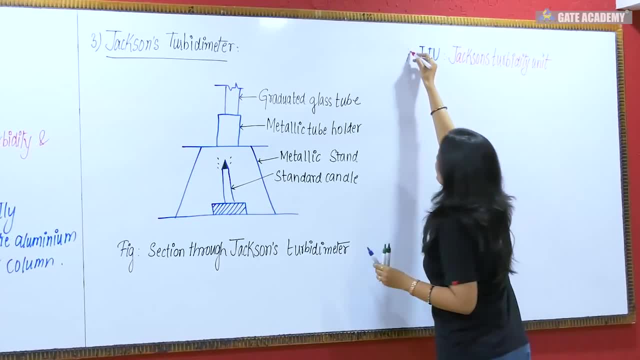 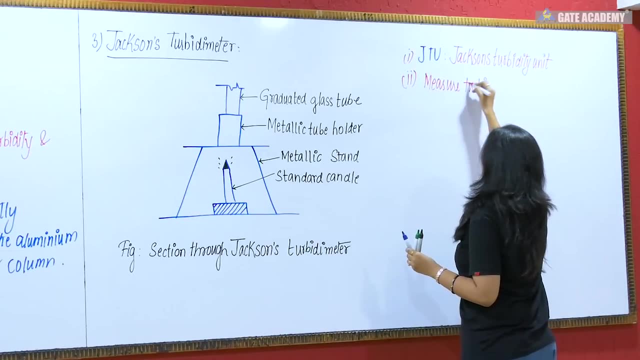 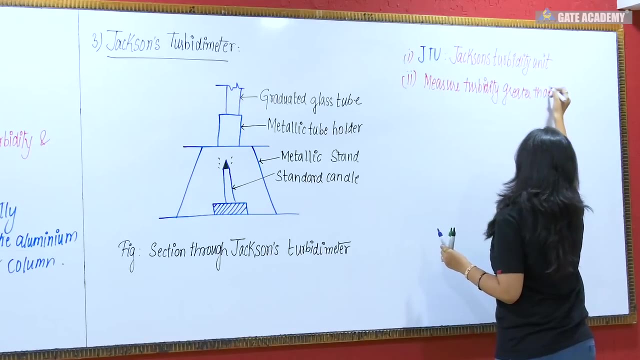 the candle. So this is the meter. This is the meter. This is the meter. So this meter gets Color. You can read this meter. This meter is 1 meter. this meter is 1.. This meter'sUCK can measure the turbidity greater than 25 mg per liter. 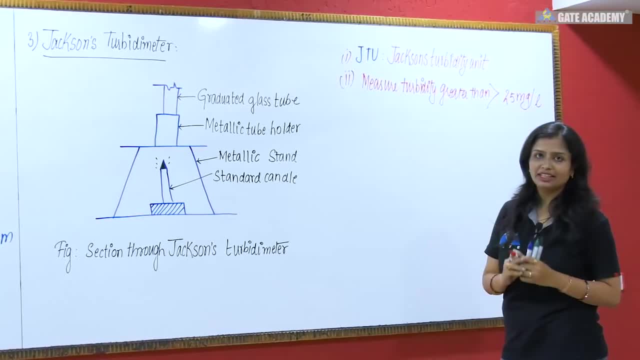 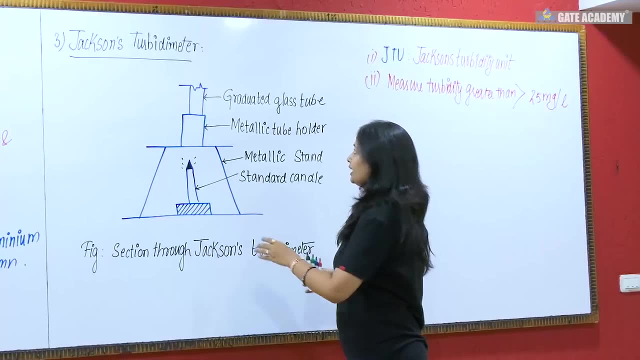 This can measure the turbidity from 25 mg to 1000 mg per liter. Now let's talk about its procedure. If we talk about its procedure, then you will see that this is a metallic tubed holder and this is graduated glass tube holder. 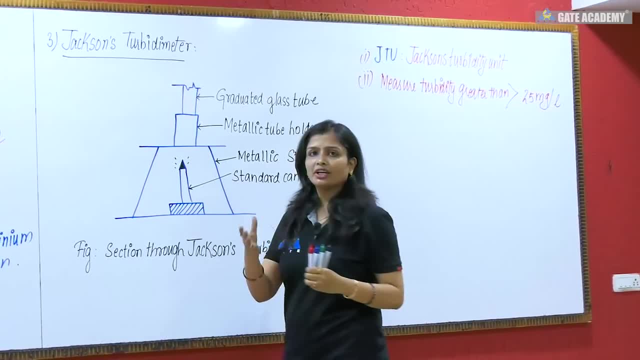 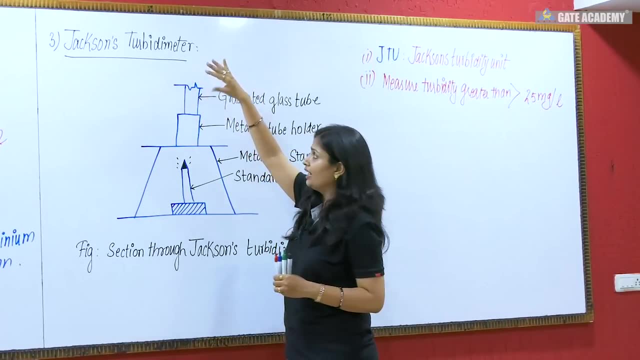 You have to test the amount of turbidity present in the water sample. You have started pouring the water slowly in it, And here a telescope is also provided generally, From which you can see in which position the flame of the candle is Initially. when you pour a little water, you will see the flame of the candle from below. 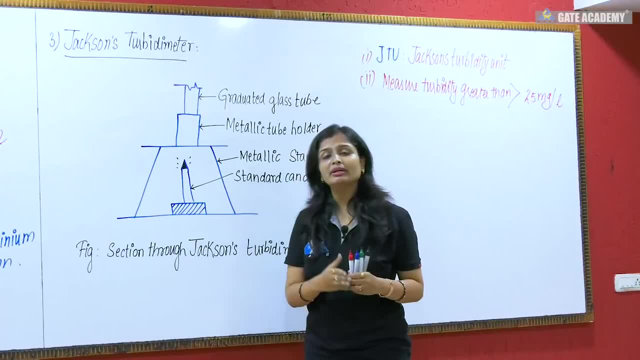 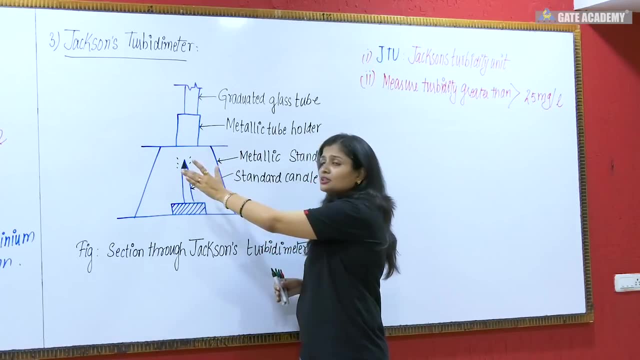 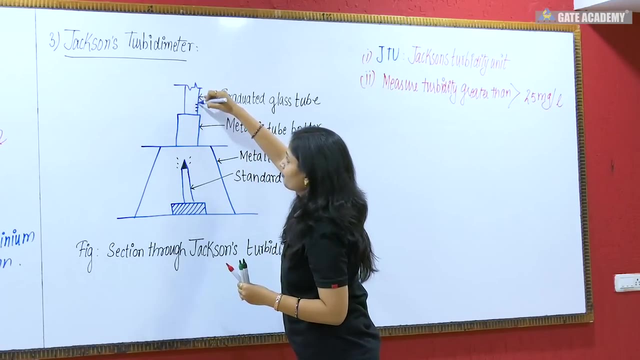 But when you pour water and if the turbidity is present in that water, So the flame of the candle or the law of the candle will stop appearing At the point at which it stops appearing. you also have graduated glass tubes. There is also a graduation mark in it. 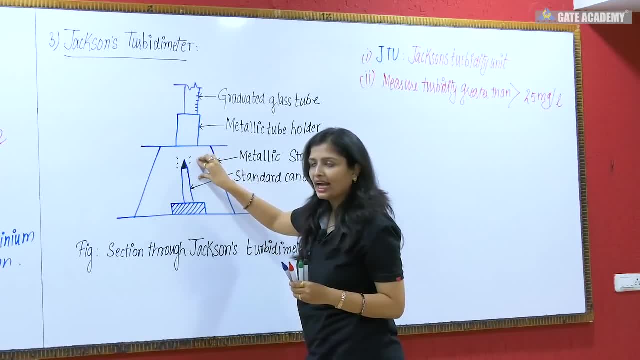 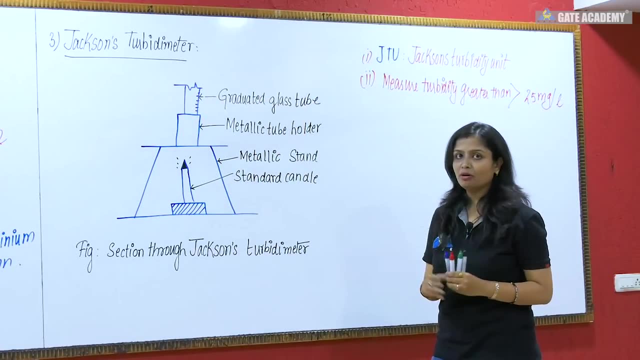 At the point at which you stop seeing the flame of the candle, you can note the reading directly from the graduated glass tube. at that point, That will be your turbidity. Now the thing is, if, after a long time, after a long time, 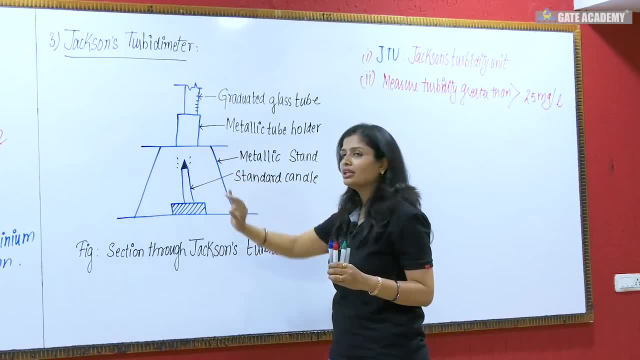 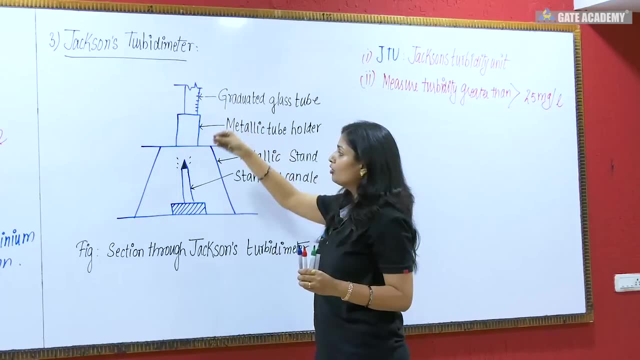 after graduation. if we stop seeing the candle flame, then it is good for us, Because if we pour a little water at a small level and we stop seeing the flame, it means that the water is very turbid. But if we pour a lot of water, 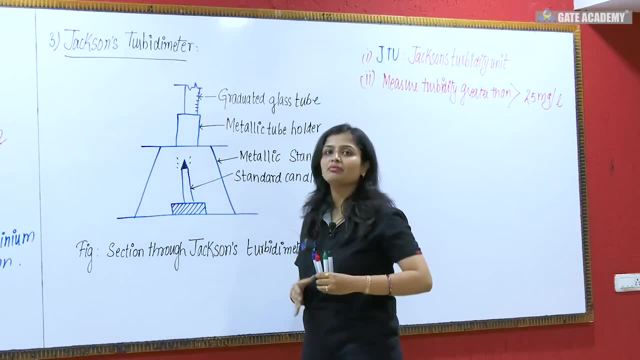 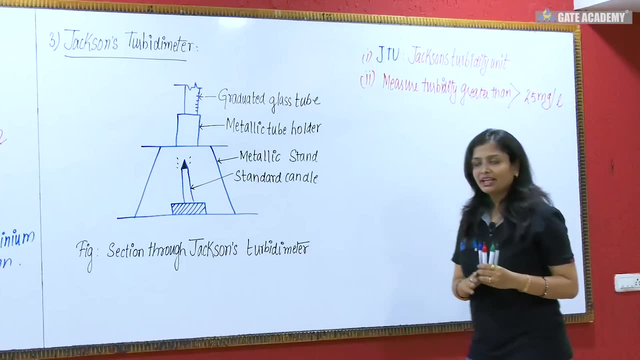 after an interval. if we stop seeing the candle flame, it means that the turbidity of the water is a little less Fine. But its drawback is that it has a turbidity of more than 25 mg per liter. It can tell the turbidity of more than 25 mg per liter. 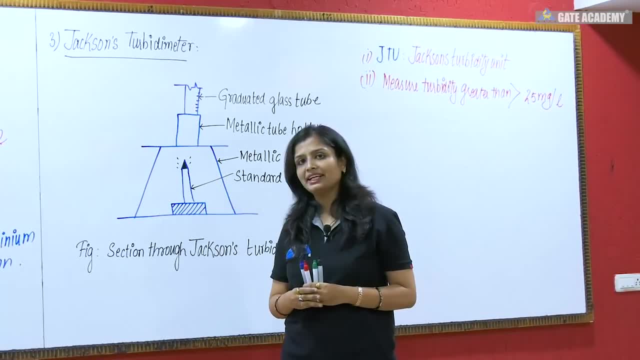 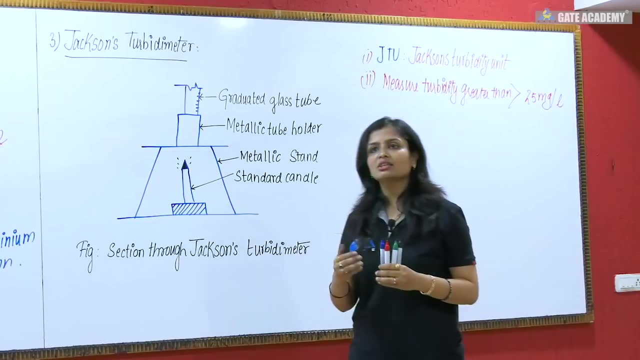 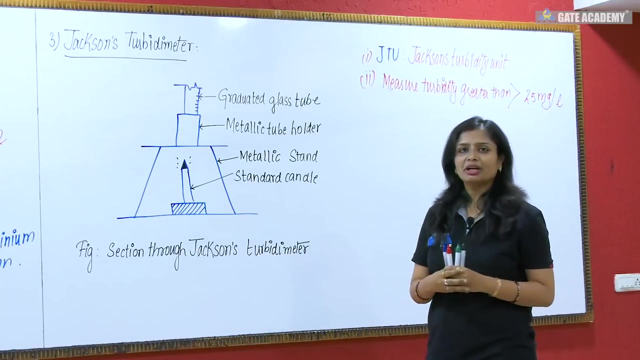 But we have read that for our body 5 to 10 mg per liter is required. So that's why we generally use Jackson's turbidity meter for water consumption. We have to detect how much turbidity we do not use Because it has a hindrance or drawback that it measures more than 25 mg per liter. 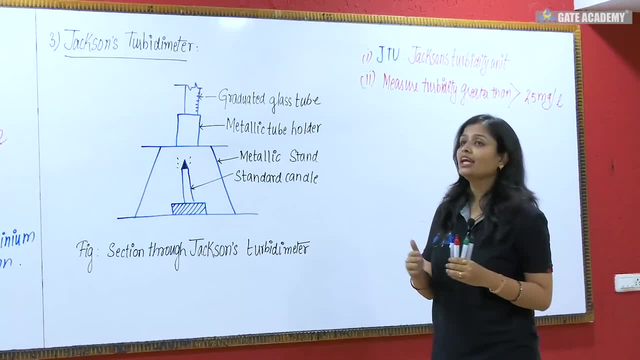 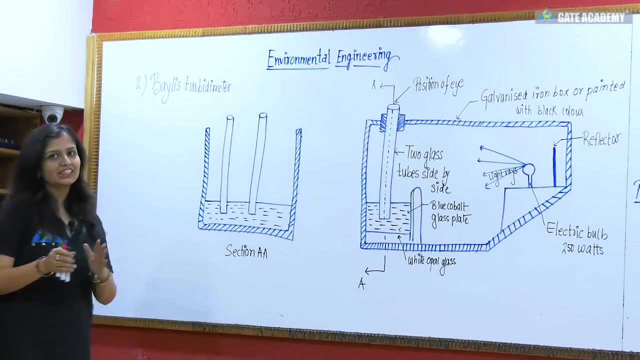 That's why we read an advanced version of Jackson's turbidity meter, That is, the Bayliss turbidity meter. Now we will be proceeding to Bayliss turbidity meter. Now, coming to the second one. initially we discussed the Jackson's turbidity meter. 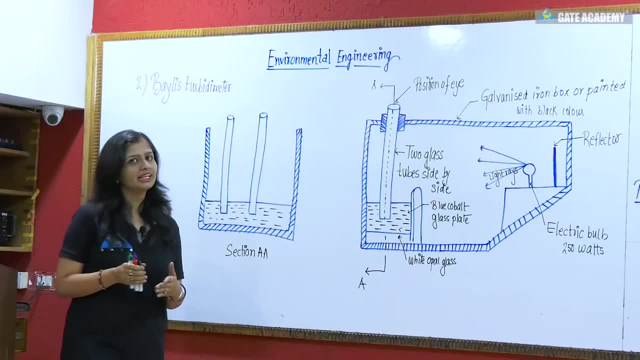 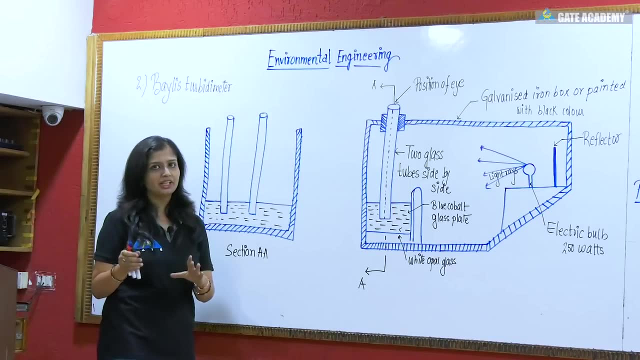 And I told you that the disadvantage is it can measure turbidity greater than 25 mg per liter, And we can also say 25 JTU. Both of them mean the same: JTU means Jackson's turbidity unit. Now, after that we will talk about Bayliss turbidity meter. 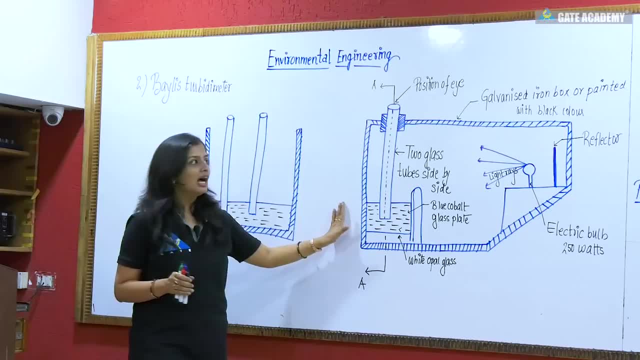 Here. I have taken a section of AAS and I have drawn it. You can see the Bayliss turbidity meter In this. this is the position of eye. These are two glass tubes side by side, Which is actually like this. 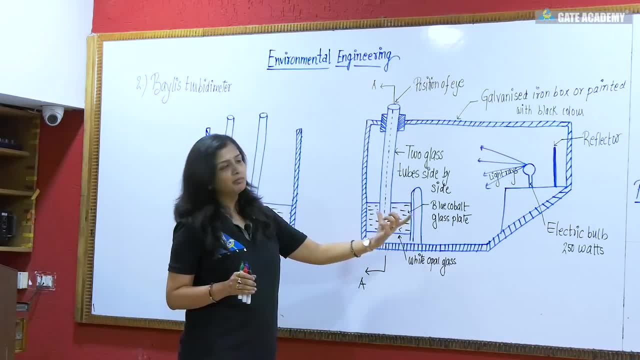 After this you have a white opal glass here. There is a blue cobalt glass plate. There is an electric bulb of 250 watts, There is a reflector and light rays, As you can see, which comes out of the electric bulb. 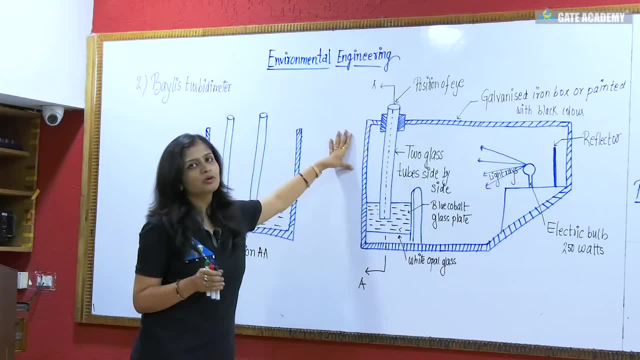 Now, with this, we have this galvanized iron box. The main reason to take a galvanized iron box is that generally there is corrosion in the iron, So we mix it with zinc and use it. So galvanized iron box, or painted with black color. 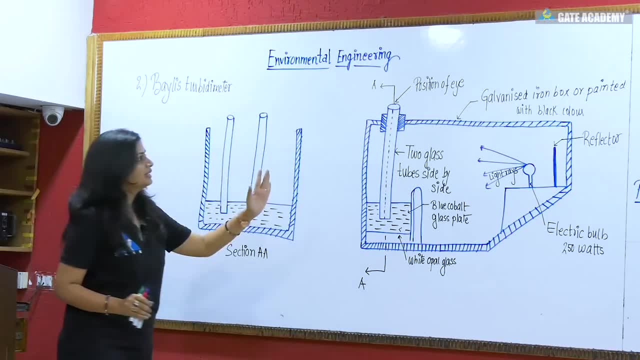 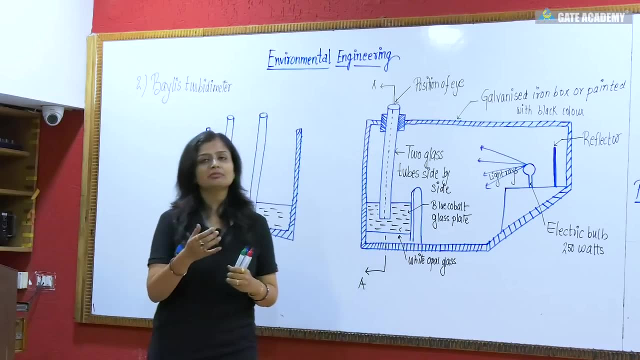 Or you can paint it with black color. Okay, So you will know what all things we use in Bayliss turbidity meter. Now it comes to how this procedure works. How do we measure the turbidity? So see what happens. You have two test tubes here. 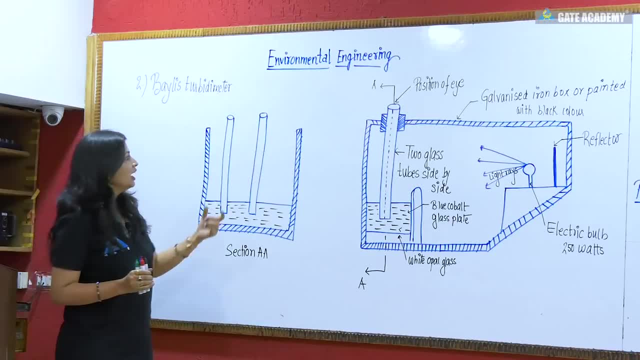 There are two samples. What will you do? in one sample, The one you have to detect is raw water, You fill it. And one, And in one sample, in one tube, the one whose turbidity you already know. take that. 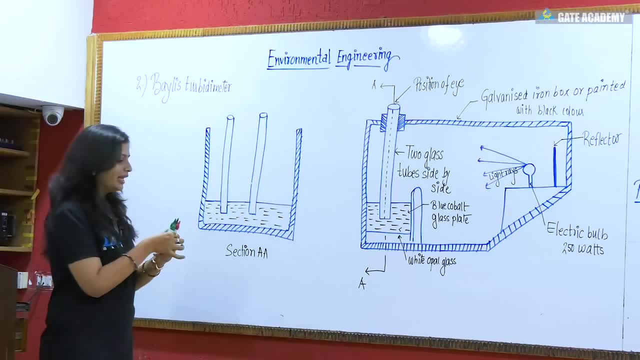 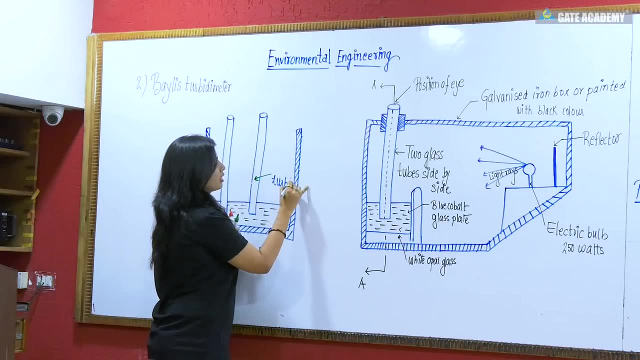 What did I say In one? in one tube we will take turbidity to be find out. Turbidity whose we have to find out? Turbidity of raw water sample- Okay, Whose turbidity we have to find out? 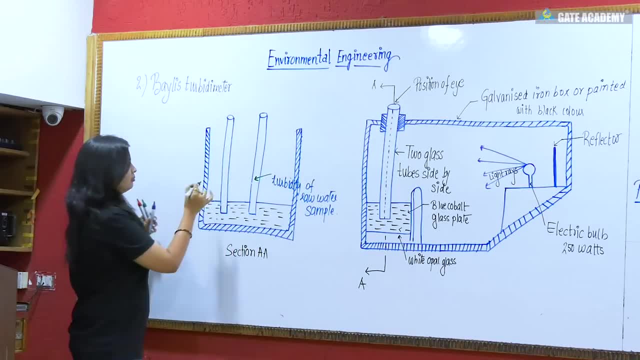 And in one we will take turbidity of known sample. Whose turbidity? we have to find out. Turbidity of known sample. Now, what we have to do in this? We have put these two, We have poured the water in the sample. 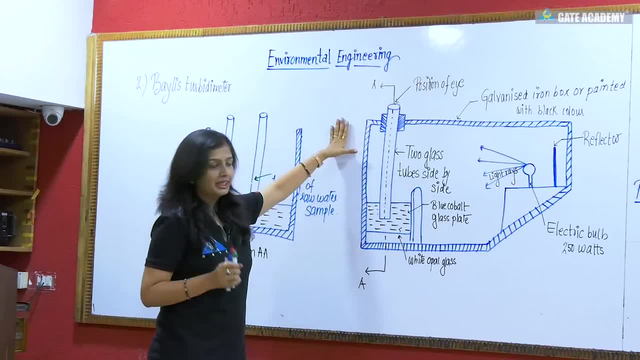 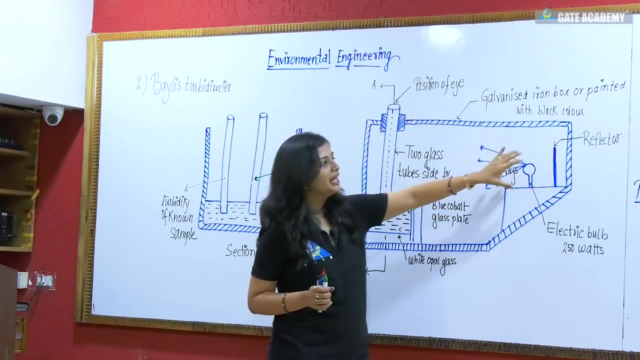 One whose we have to find out and one whose we have to find out: Turbidity. Now, what we have to do in this: You have to burn the electric bulb of 250 watts to pass the light rays And kept a reflector behind it. 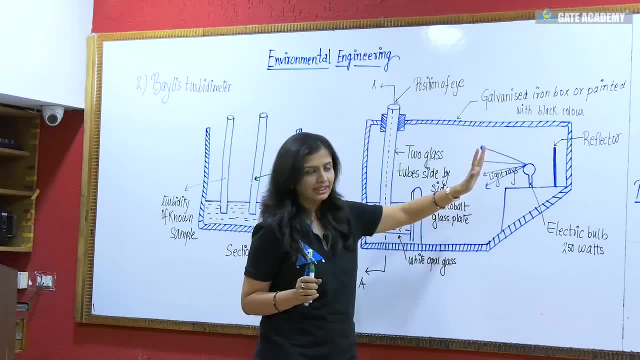 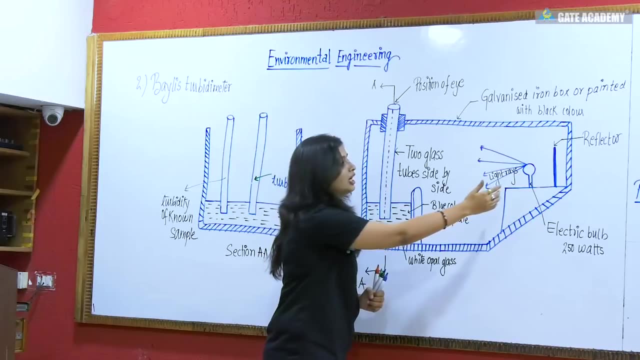 So that water, So that it can reflect the light Which is coming from the electric bulb. Then what it did- Electric bulb, not reflector. when it started the electric bulb, it reflected the light. When it reflects the light, then we have to see from our position of eye. 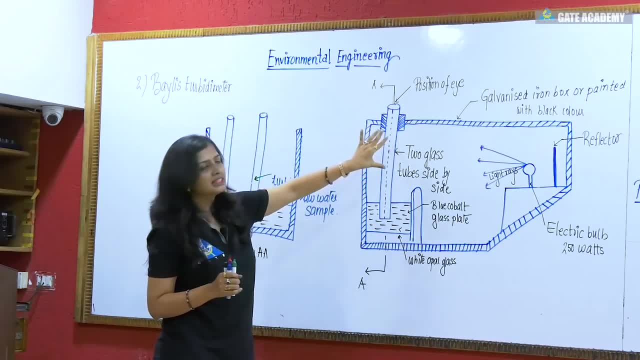 whose turbidity we knew its color and whose turbidity we have to find out its color. both should be same. In case the color of both is not same, then whose turbidity we knew of known sample. apart from that, we will bring another turbidity. 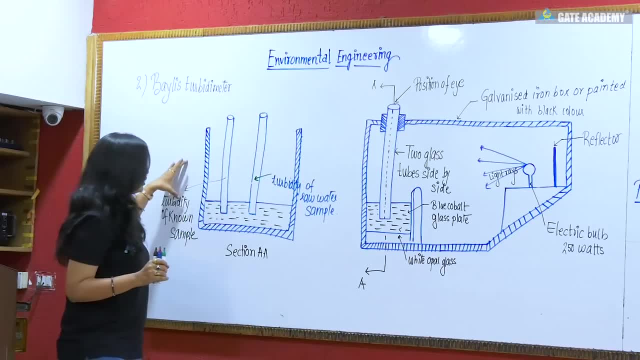 whose turbidity we know of. Because this turbidity, the turbidity of this raw water sample, these two did not match. Okay, So we will keep the raw water sample as it is, But we will bring the sample of another turbidity. 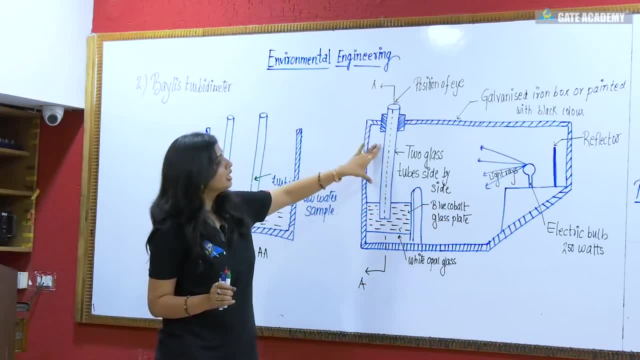 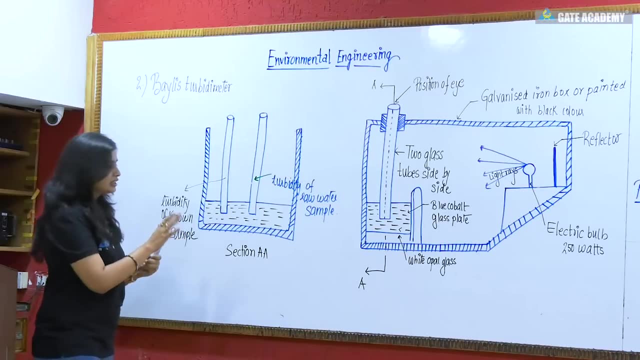 And then we will use the same process. We will do this till the time, till the time we do not get the same color of both. Fine, We use this principle- This is called Bayless Turbidity Meter- And this principle. 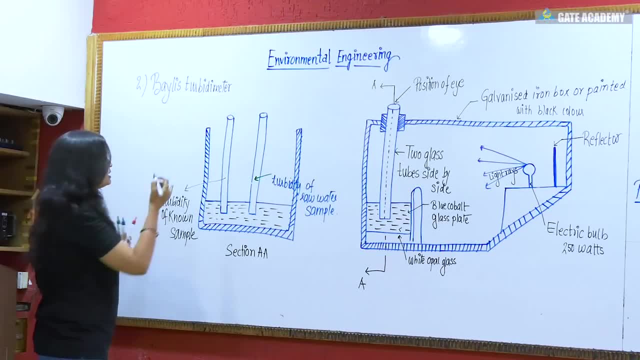 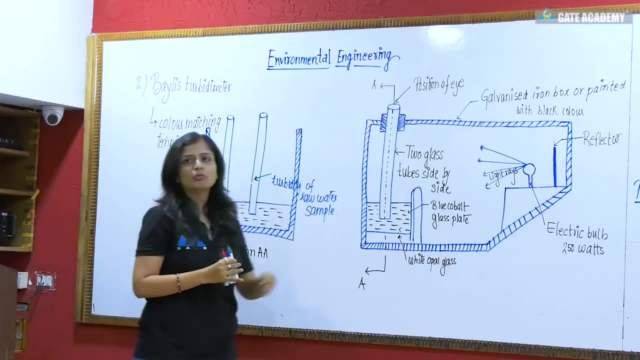 we use Bayless Turbidity Meter. If you ask yourself on which principle it works, then you should know we use it on color matching technique, Because you are seeing what you are doing every time. you have a blue cobalt glass plate here. 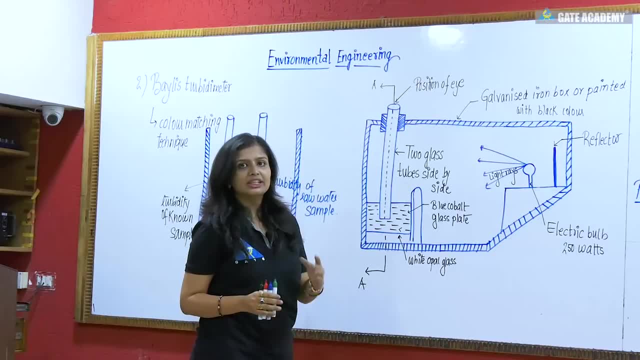 So when you pass the light rays then you should see blue color in both. If it is not visible, then you change the sample of the turbidity you knew, then see if the colors match or not. We used to do this procedure. 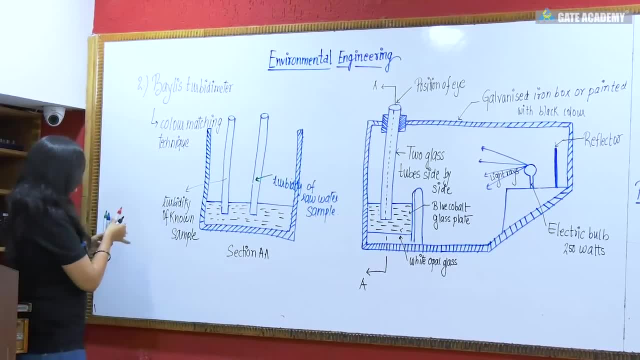 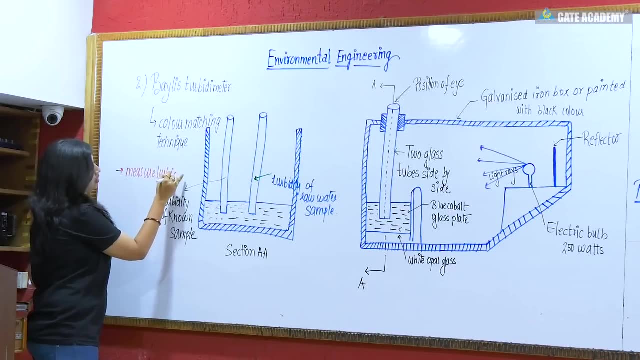 So that is why we are telling it it is based on color matching technique. Second thing: it can measure the turbidity up to 2 ppm Means. if there is any turbidity present up to 2 mg per liter, then Bayless Turbidity Meter can measure it efficiently. 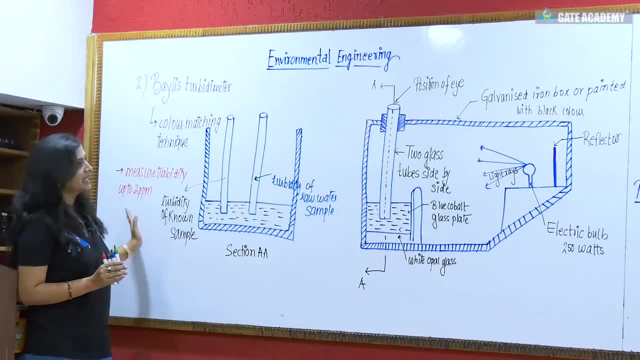 Fine. So these were the important things which you should know. If you just ask yourself about galvanized iron box or which turbidity meter is based on color matching technique, then you can say it is based on Bayless Turbidity Meter. 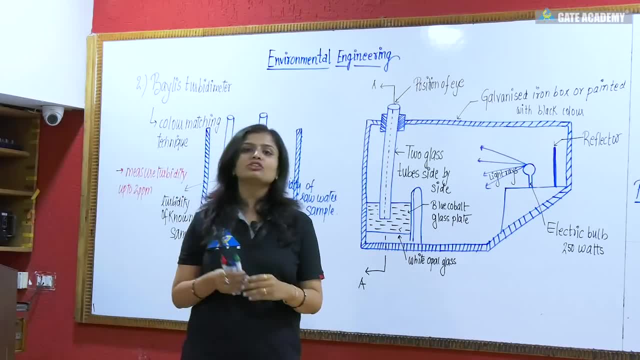 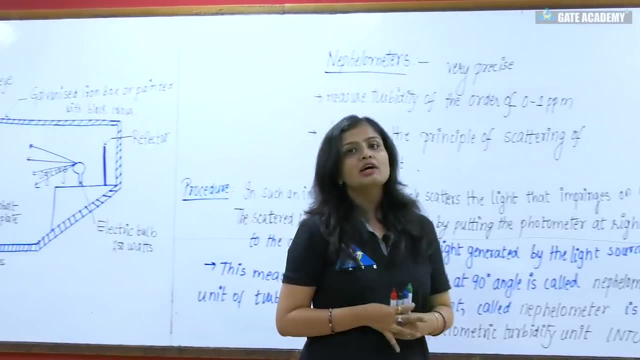 Fine, So this was our Bayless Turbidity Meter. After this, the most efficient which we generally use now is Nephelometers. I have written the important points of Nephelometers, But before that, let me tell you: 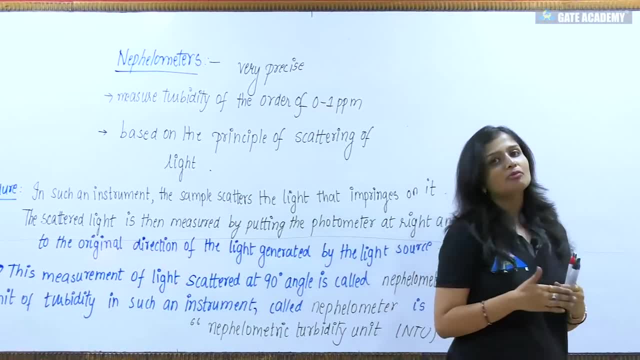 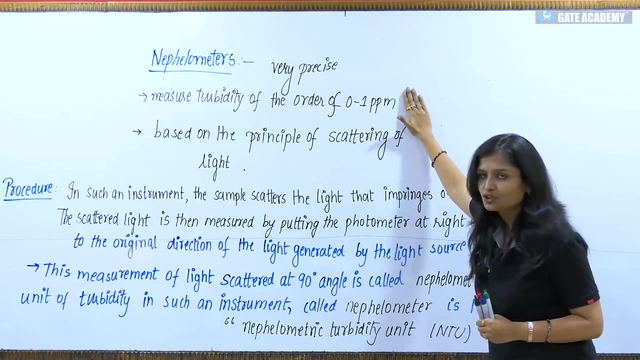 what are Nephelometers? Nephelometers, basically, we use it because its turbidity is 0 to 1 ppm Means it is a very precise instrument. After this, it is based on the principle of scattering of light. 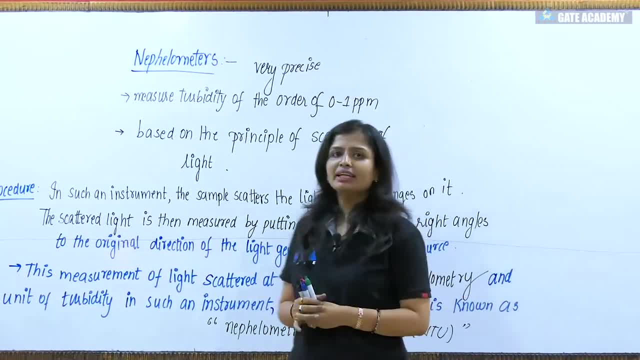 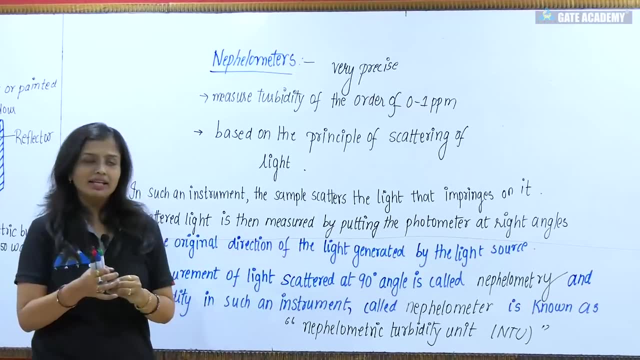 And if you see the procedure of this, what we do is you take a sample- I have written it here. you take a sample and it scatters the light which comes on it. Fine, Now, when it scatters the light, 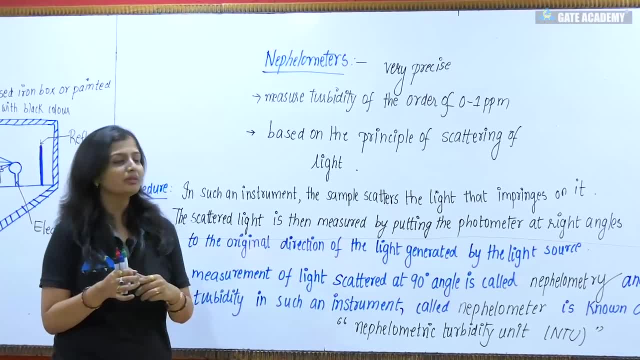 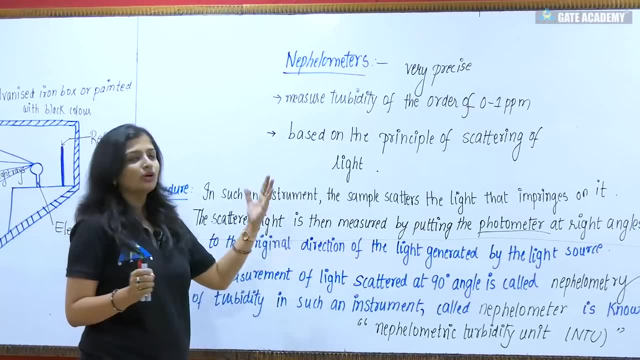 then we have to measure that scattered light. And how do we measure it? By putting the photometer at right angles. We keep the photometers at right angles and measure that the photometers are kept at right angles and measured to the original direction of the light. 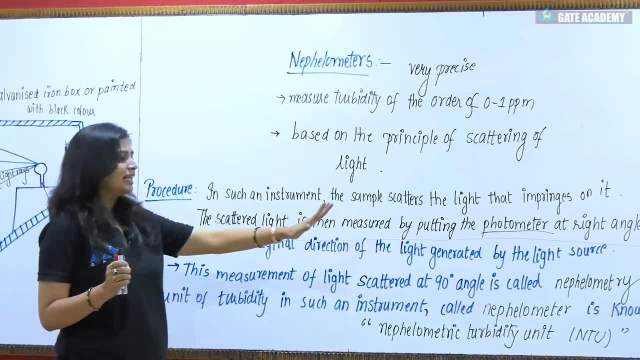 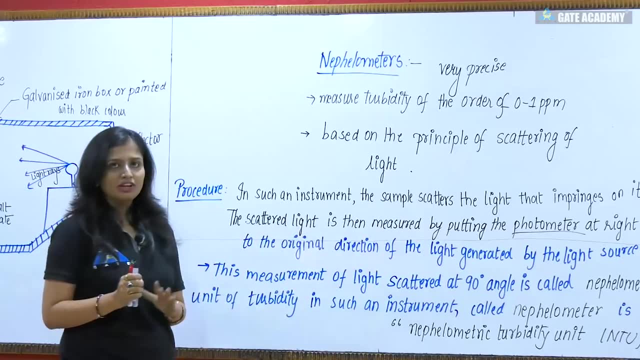 generated from the by the light source. Fine, After this, what happens When this instrument scatters the light at 90 degree angle? we call it Nephelometry. What is the instrument? Nephelometers And the unit in which we measure the turbidity. 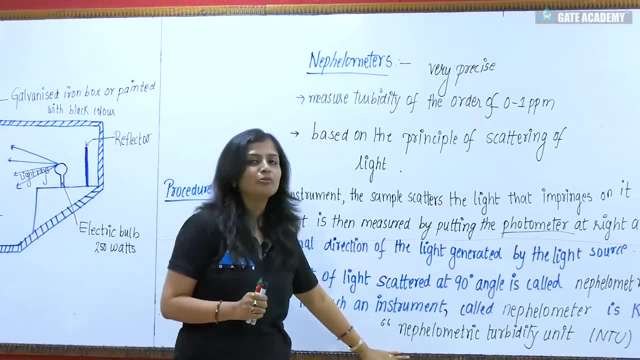 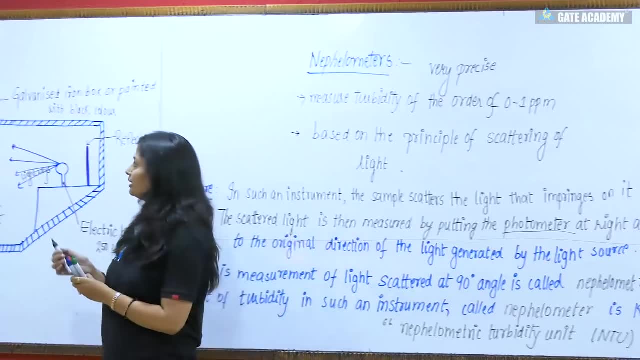 in the case of Nephelometers, it is called Nephelometric Turbidity Unit. You have to remember when we talk about Bayless Turbidity Meter, then we measure it. I will write it here: when we talk about Bayless Turbidity Meter, 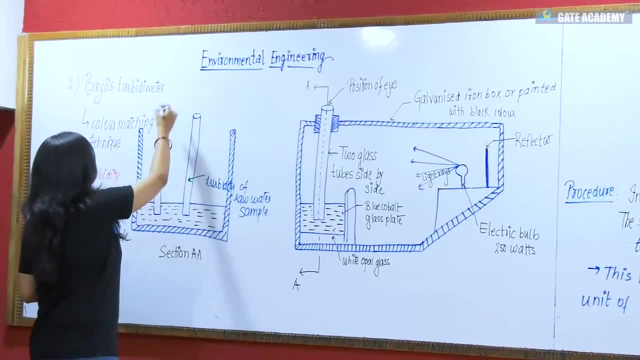 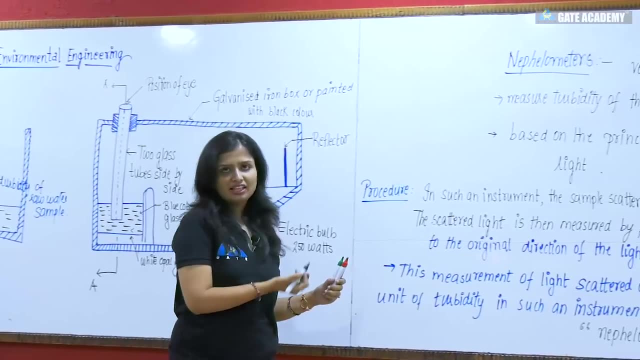 when we talk about Bayless Turbidity Meter then we measure it in BTU, In Bayless Turbidity Unit. But generally we use today's Nephelometers. so I have written here that the turbidity in such instruments 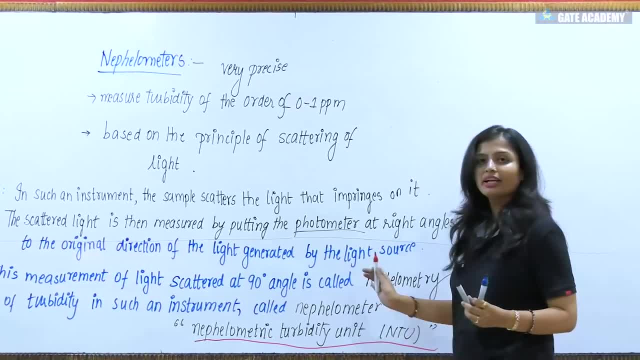 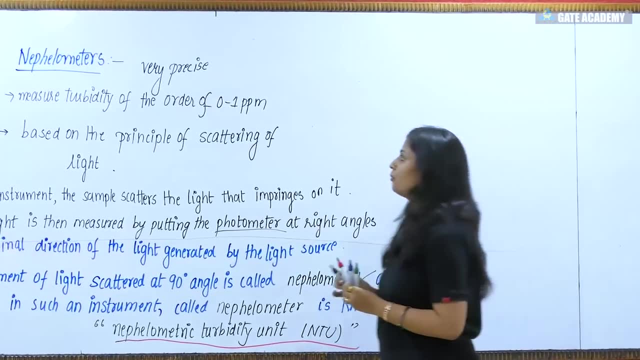 in Nephelometers. we measure it in Nephelometric Turbidity Unit, As we call it in short form, NTU. Fine, You just have to remember few things in it. It is important for you that we measure the turbidity from 0 to 1 ppm. 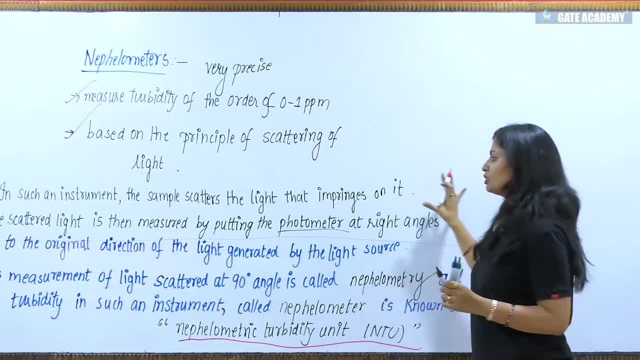 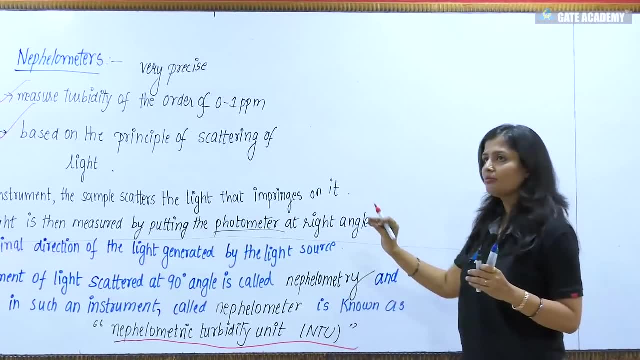 it is based on the principle of scattering of light. You will not be asked about this procedure, just for you to understand that it scatters the light which comes in its direction and we measure it by putting photometer in the direction of that light source. 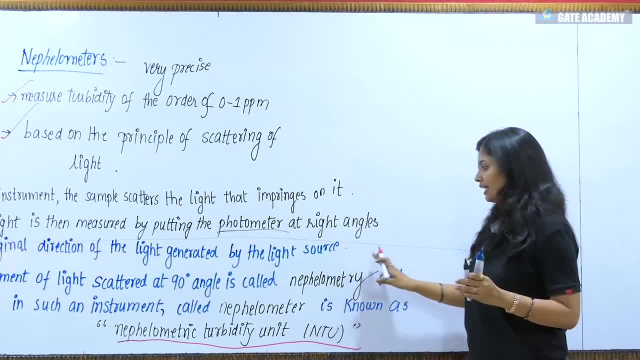 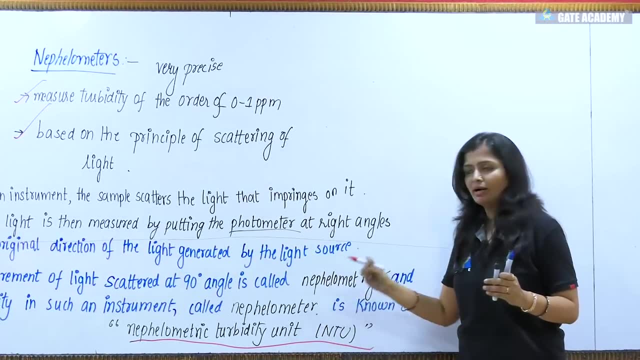 in the direction of the right angle, Fine, And after that it scatters at 90 degree. it is called Nephelometry, The instrument which is used, it is called Nephelometers. And what we measure? what are our values? 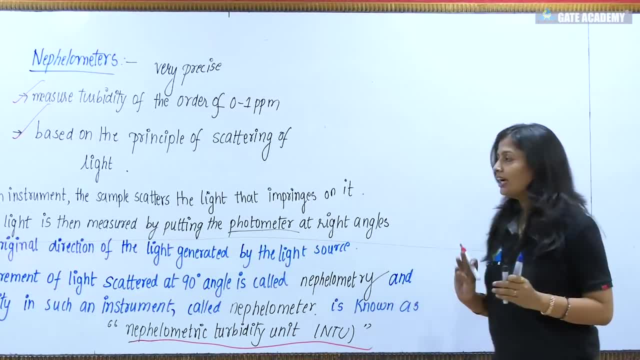 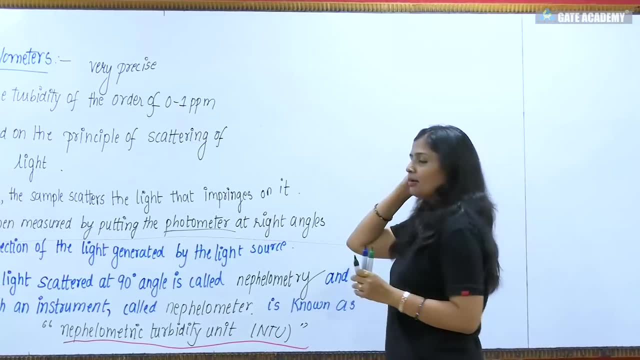 it is called Nephelometric Turbidity Unit. Fine, So now we know all this about Nephelometers. We use Nephelometers, But sometimes what happens is- I told you that generally when we use Turbidity- 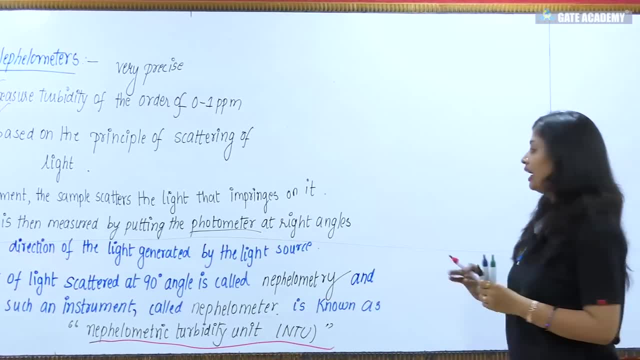 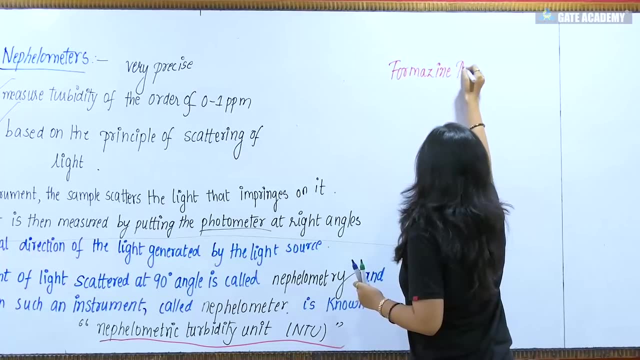 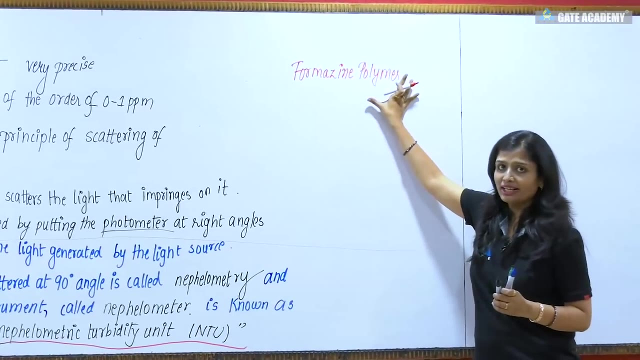 we use Silica as our benchmark. Yes, Silica is our standard solution, But sometimes if we take Formazine Polymer solution, if we take Formazine Polymer solution instead of Silica, we take Formazine Polymer. In that case, 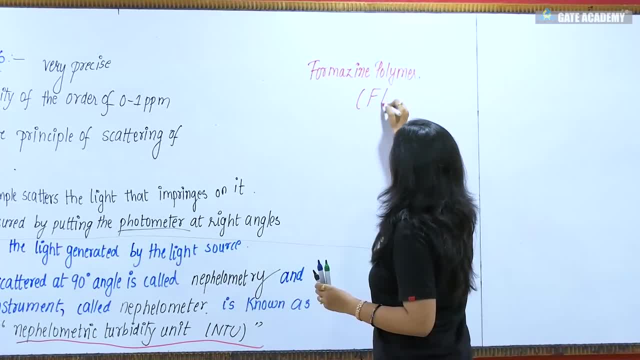 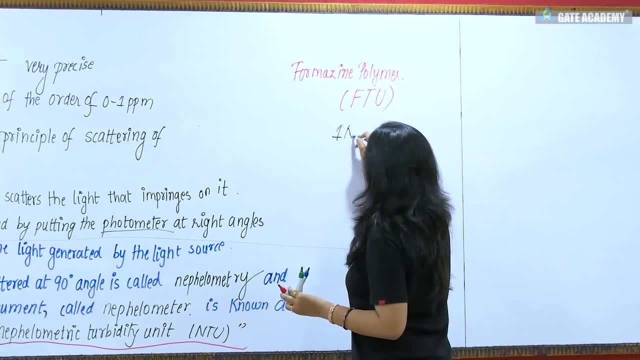 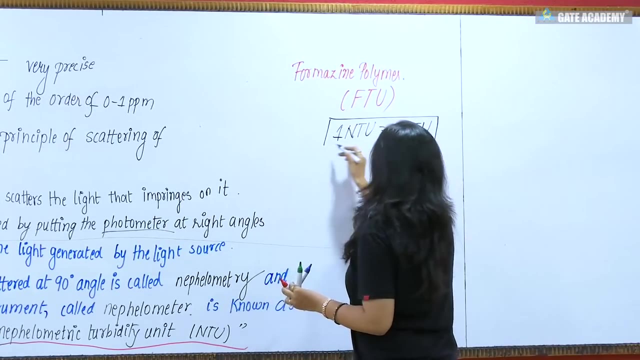 the Nephelometric Turbidity Unit. we can write it as Formazine Turbidity Unit. In this case, if you say 1 NTU or you say 1 FTU, Formazine Turbidity Unit, these two are the same. 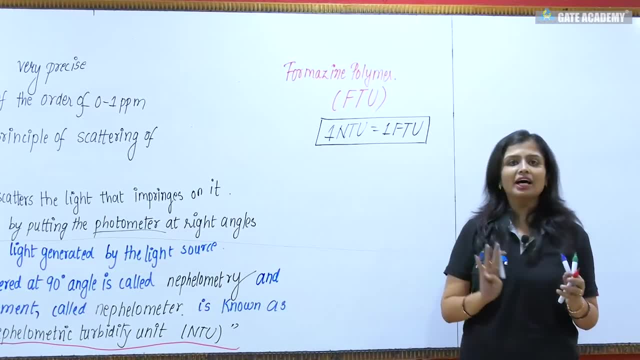 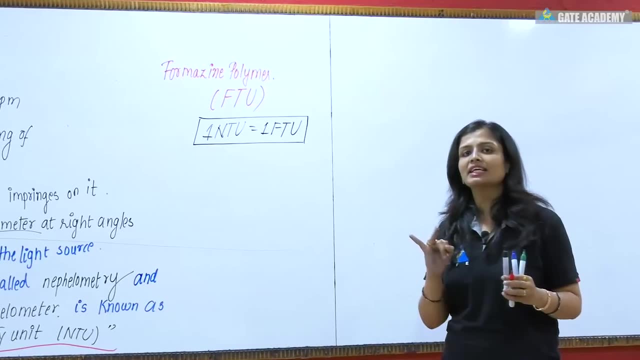 Fine, Did you understand? So these four types of instruments which we use, or the Turbidity meters which we use, which we use First, the Turbidity Rod which we measure in the field Jackson's Turbidity. 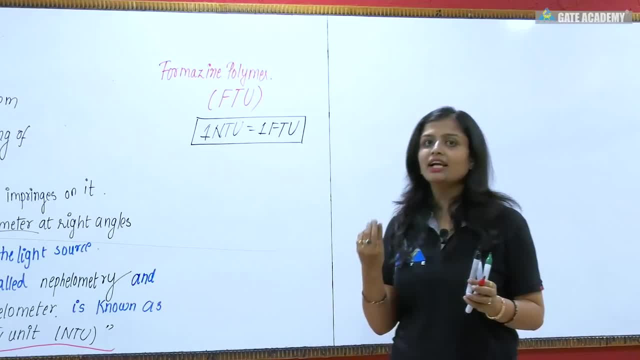 which measures the Turbidity of more than 25 mg per litre. Third Bayless Turbidity Meter which measures the Turbidity of up to 2 ppm. And the last is our Nephelometers, which can give us the Turbidity. 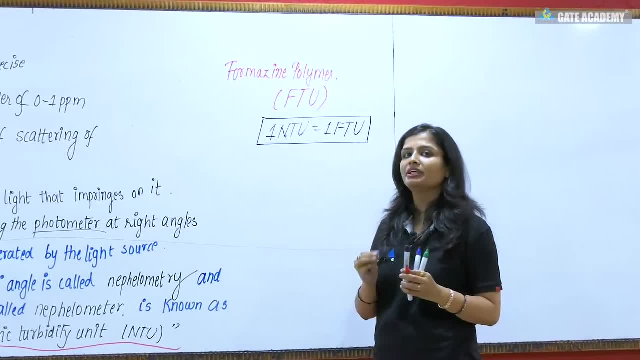 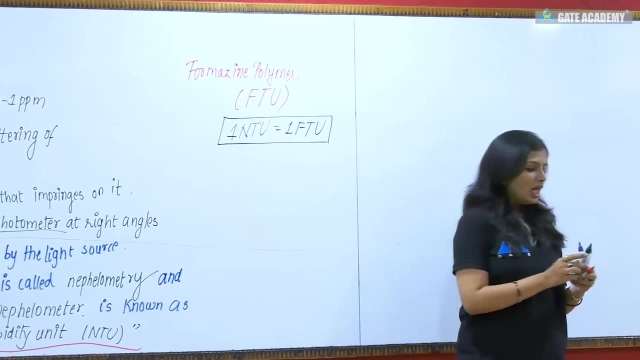 of up to 1 ppm. from 0 to 1 ppm It can tell us in the water sample. So we completed the Turbidity part, Now coming second to the colour Colour. So we have completed the Turbidity part. 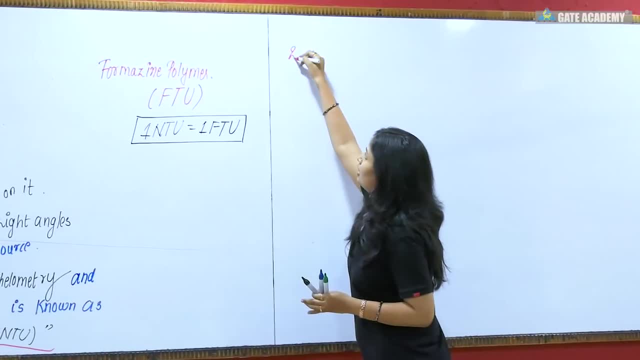 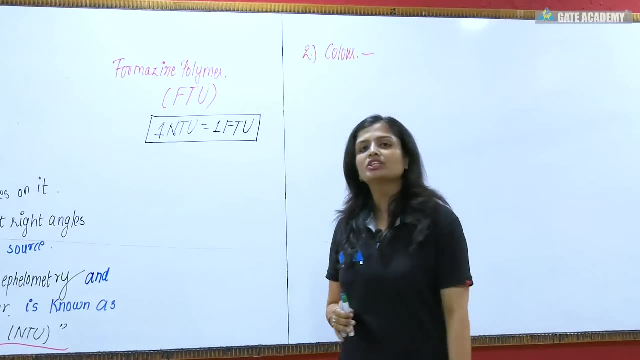 Now coming second to the colour Colour. Now you have water. generally, water itself is colourless. If you look at pure distilled water or chemical water, then what do you see? You cannot define any colour to the water. 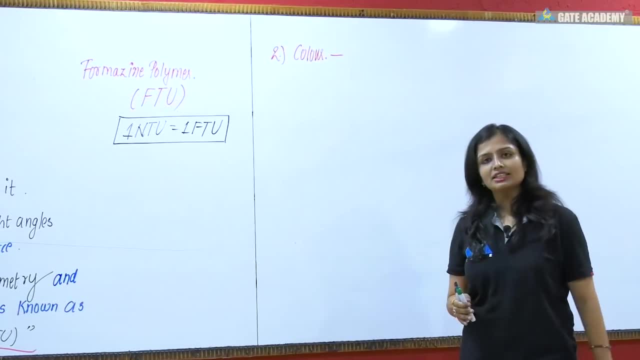 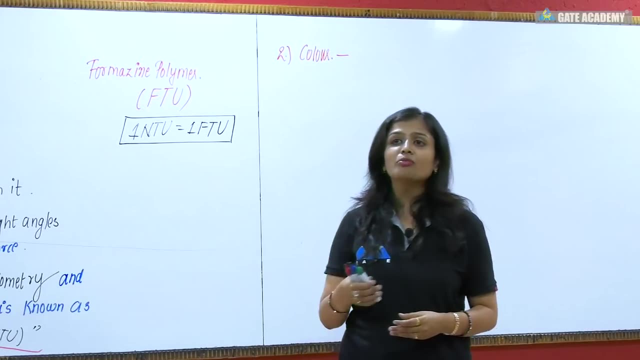 because we believe- and there is- that water is a colourless compound. But you know that if there is any alga or any vegetational matter, sometimes water starts to look colourful to us. We start seeing different colours in it. 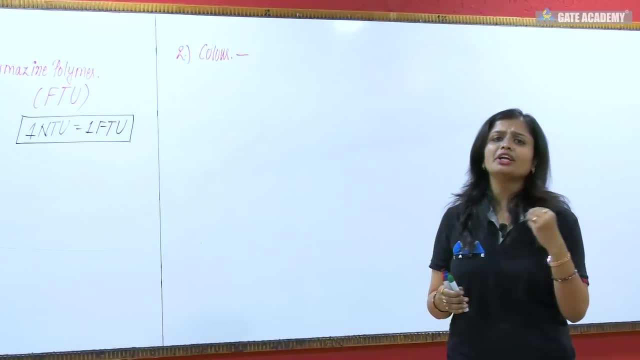 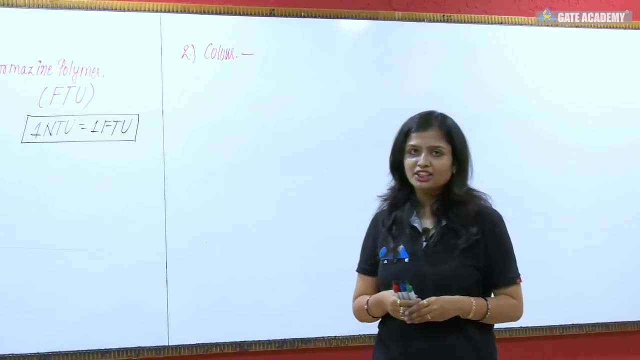 Why? Because water does not have colour, But decay or vegetational matter can also be present in it, Or due to any alga or plankton, the colour of water changes. Sometimes these things, if the water is colourful. 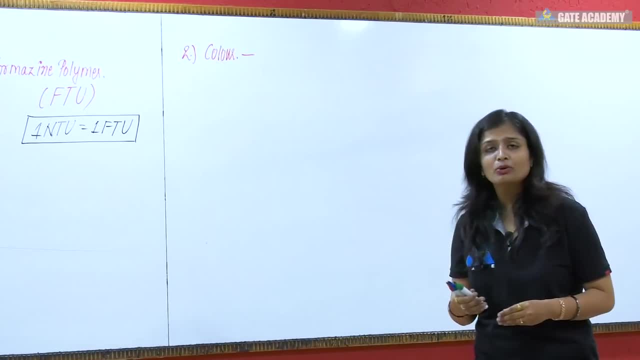 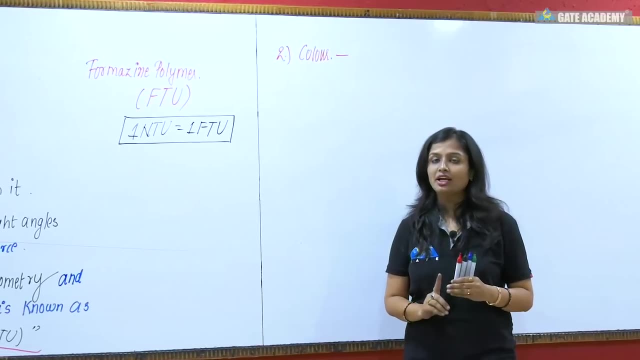 then it can be harmful for us. And even if it is not harmful, then also we cannot drink coloured water, Fine. That is why it is very important for us to measure colour too, First thing. Now it comes to: 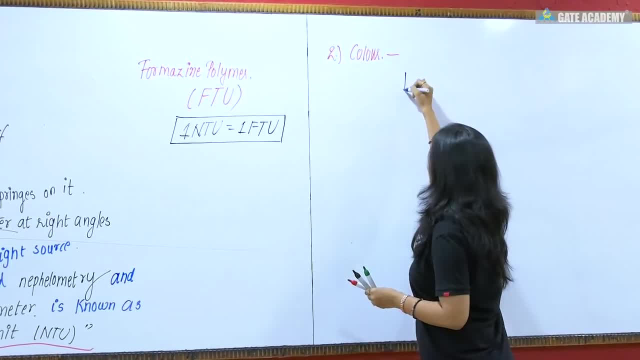 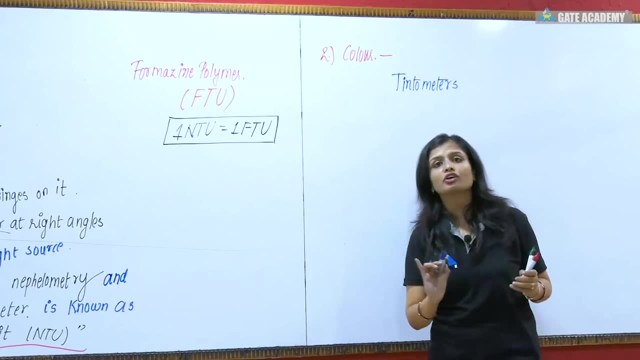 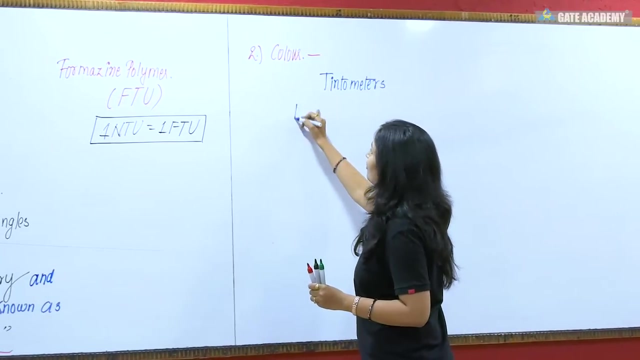 how to measure colour. We measure colour. This is called Tintometers, Through which we can measure colour. Fine Tintometers is an instrument through which we can measure colour. Apart from this, we also have a Nestle's tube. 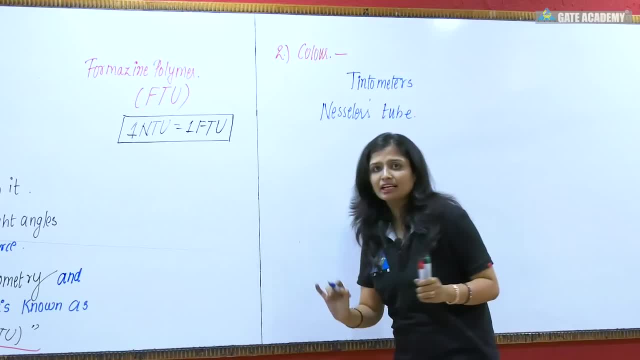 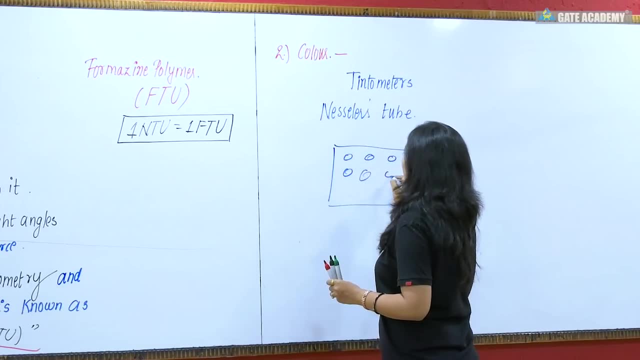 Nestle's tube. The main aim of this is that in this already different, there are many tubes here of different colours And they are given in different amounts. How much concentration is there Means if this colour is present? 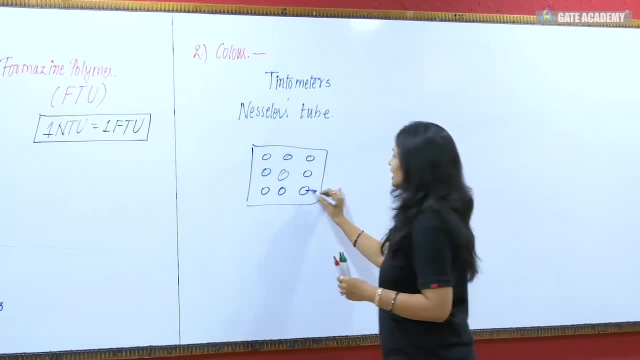 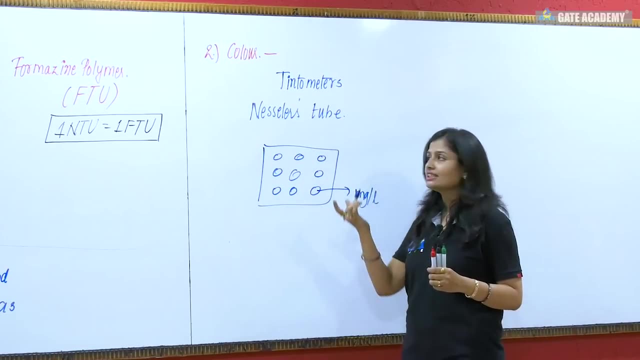 then, in what amount permissible limit is there? Everything is given to you Means: how much concentration is there in mg per litre? That? how much concentration of colour is there in water? You know this. This is called Nestle's tube, or. 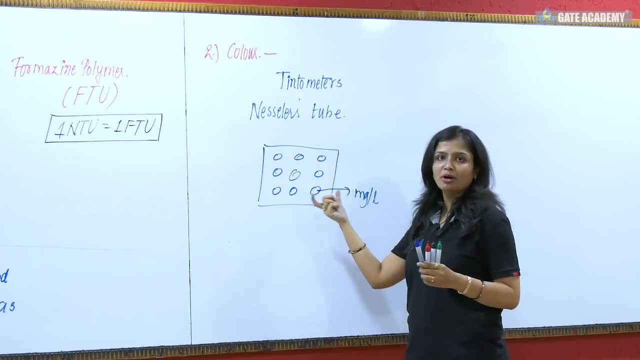 Nestle's tube. But this is the chart of Nestle's In which, in different colour amounts, how many colours are present in it that is given. So what you have to do is the raw water sample you have. 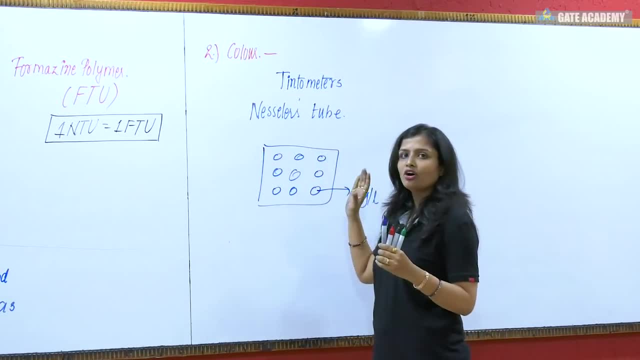 you from these in the Nestle's tube and in the Nestle's chart, the colour which is there, you match it. Your colour and the colour given in this chart will match. So you will know that how much amount of colour. 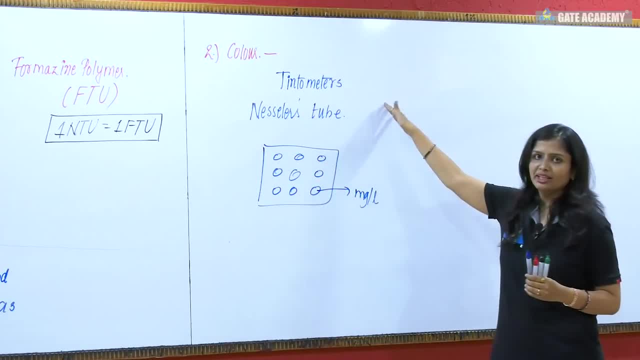 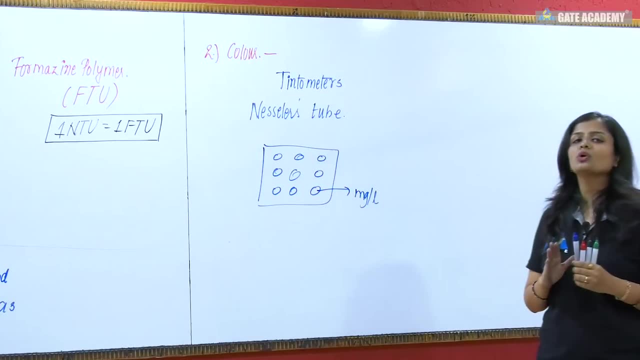 is present in your raw water sample, Or you can simply take out the colour from the tintometer. Now comes the permissible limit. So the permissible limit of colour. you are not allowed more than 20 ppm colour for drinking water. 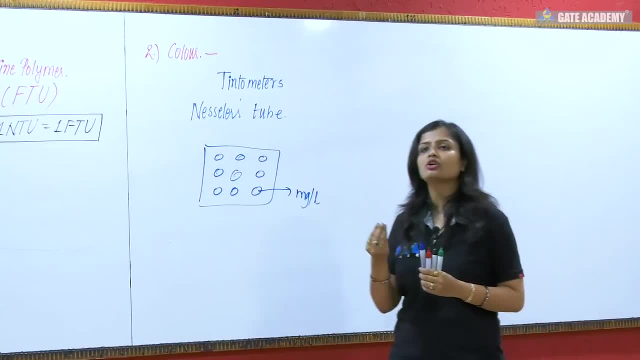 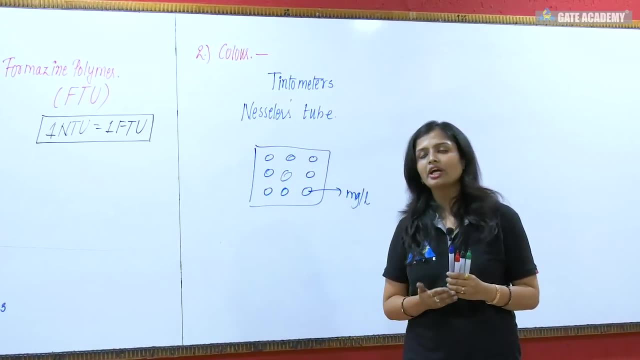 For a healthy human. if you want to consume water and it has coloured compounds, then in 1 litre of water at least 20, at most 20 mg of colour is allowed. You cannot use more colour than that, Fine. 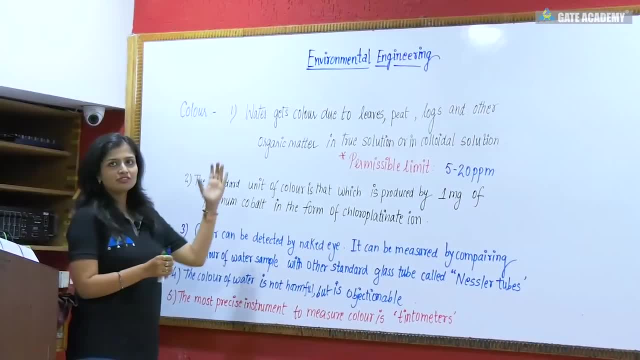 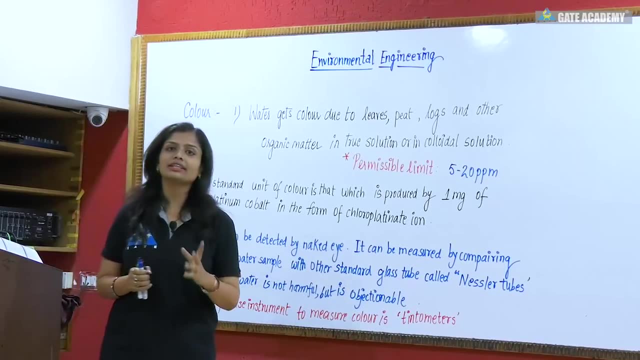 So I will write it down in the form of points. You can jot it down Now. I have jotted down the points which we discussed in the colour part. So colour water gets colour due to leaves, If leaves fall in a river. 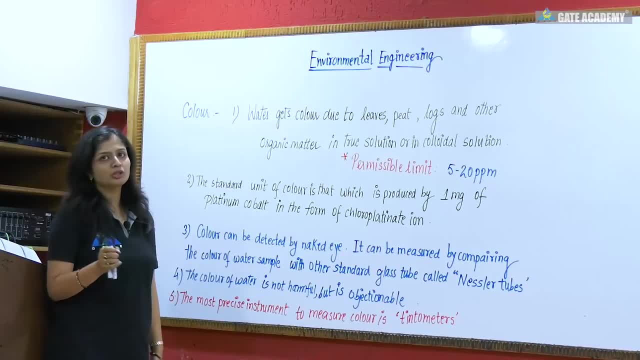 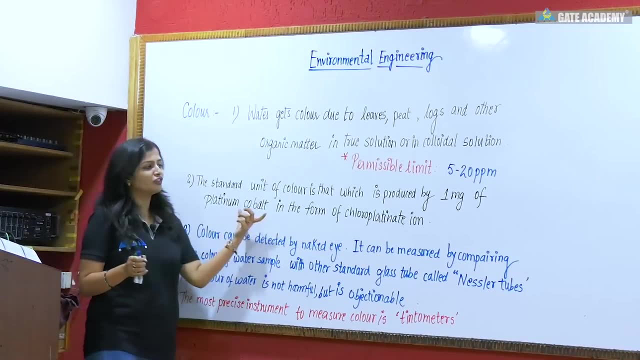 and other organic matter. water gets coloured in true solution or collider solution. Secondly, what is the standard unit of colour? It is that which is produced by 1 mg of platinum cobalt in the form of chloroplatinate ion. When we were talking. 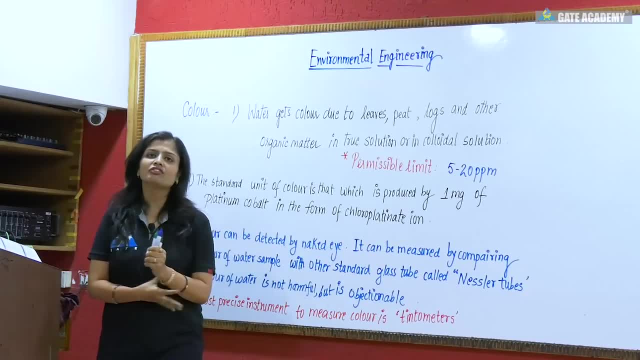 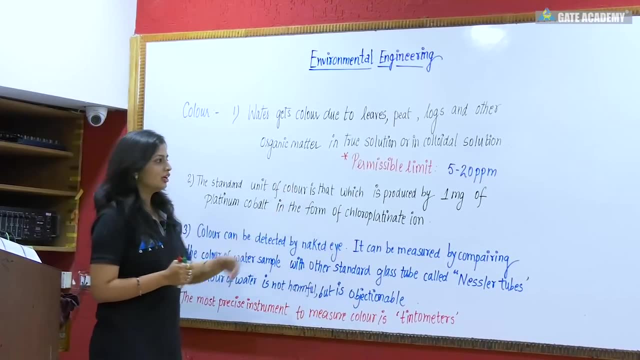 about turbidity, we were saying 1 mg silica. if it is in 1 litre of distilled water, then we call it 1 mg per litre of turbidity and 1 ppm of turbidity. Similarly, our standard unit here is 1 mg of platinum. 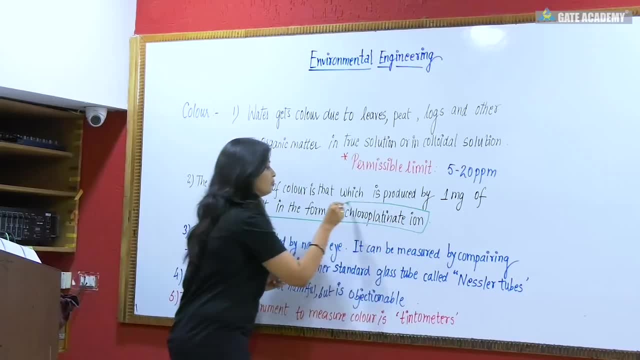 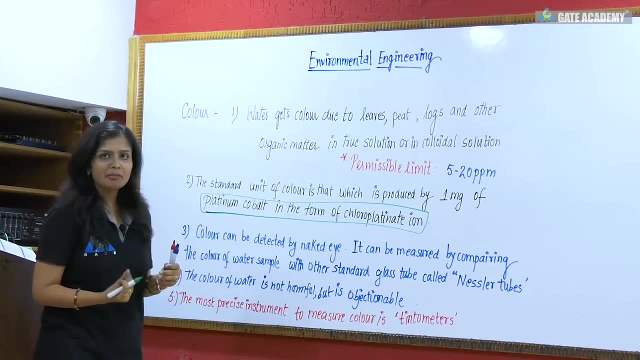 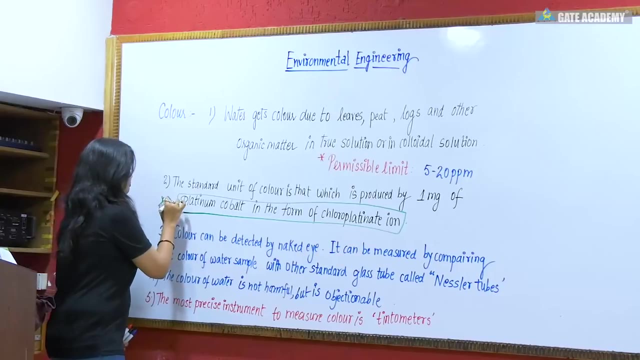 cobalt in the form of chloroplatinate ion. You have to remember this because it has been asked in the previous gate. Fine, the colour is measured in which scale? So you know platinum cobalt scale in the form of chloroplatinate ion. 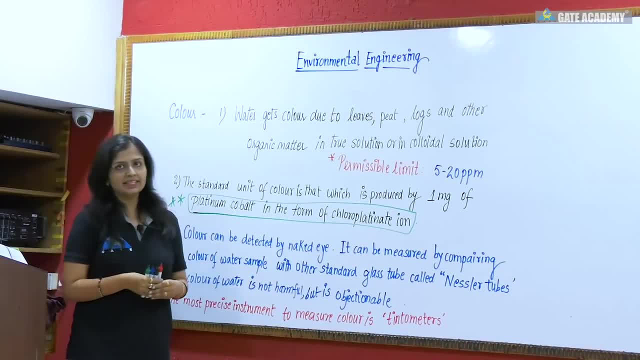 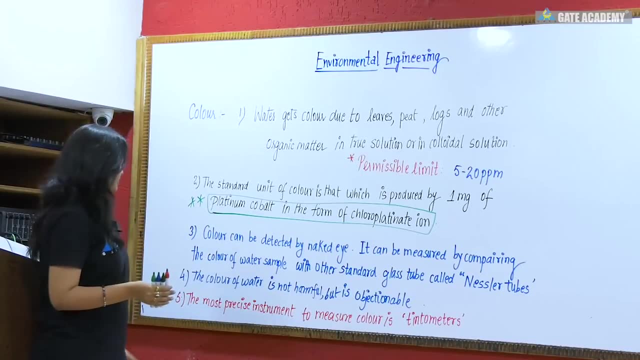 So this is important for you. Now we can see the colour with our eyes. We don't need any telescope for that. So what we do is I had told you that only I have written. colour can be detected by naked eye. 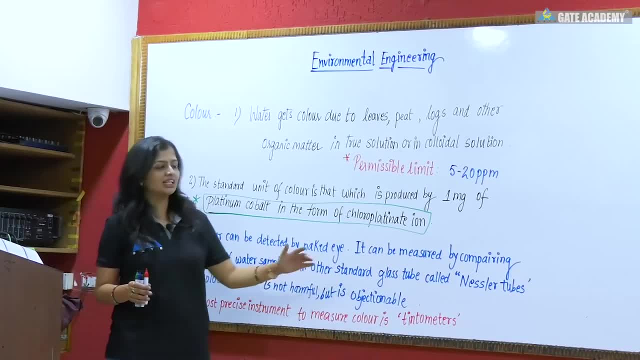 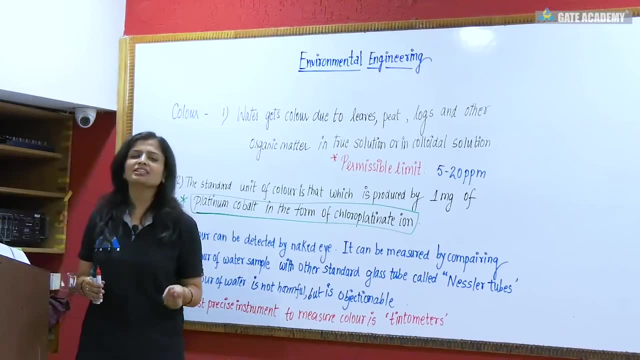 It can be measured by comparing the colour of water sample with other standard glass tubes called Nessler's tube. Now the fourth one is: colour of water is not harmful. We know that if it is present within permissible limit it is not harmful. But 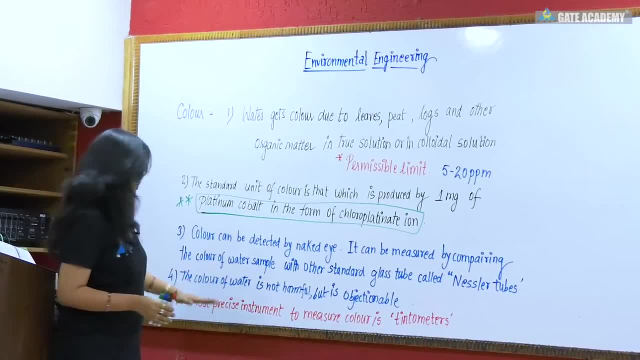 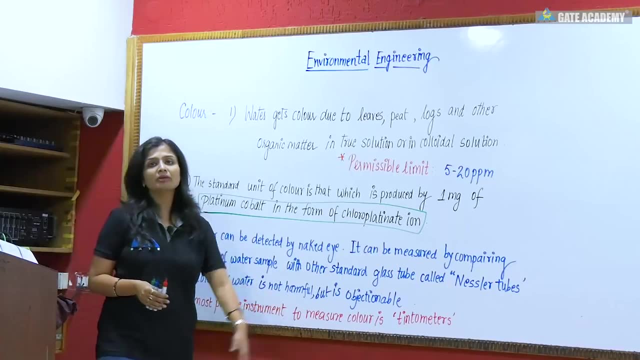 you know, if there is colour in your water, will you drink that water? No, you won't drink it. That's why it is objectionable. Last one is: nowadays we call it Tintometers. It can be asked in match the following: that in case of 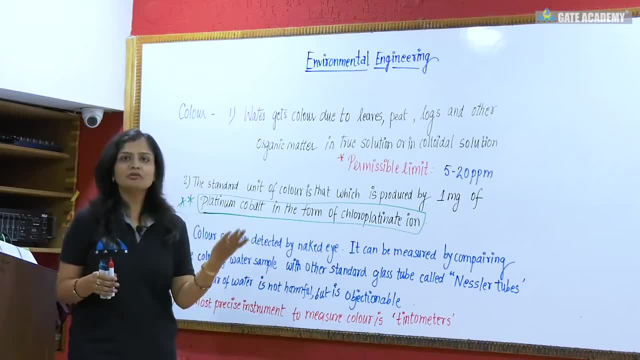 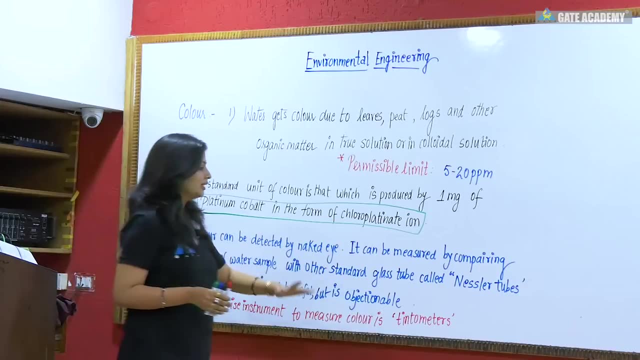 turbidity meters. it will write Baileys, buzz or nephelometers or Tintometers, And if we ask you in match the following, that with which we measure colours, then you should know that Tintometers is used to measure colour. Fine. 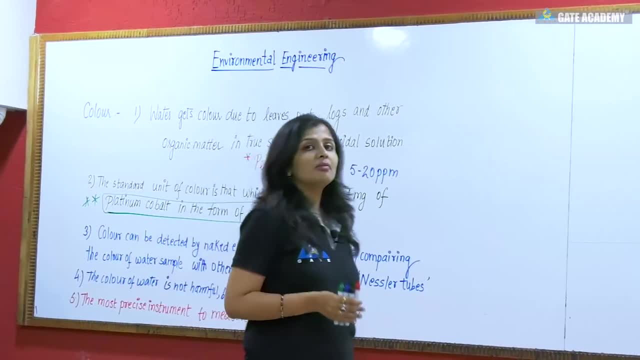 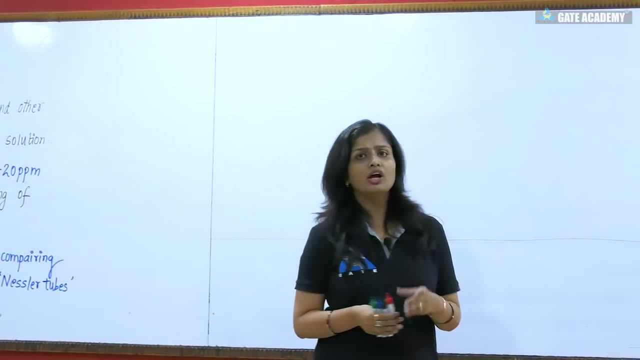 So this was our colour part. Now, if we talk about odour, Sometimes we say that taste is not good. taste is bitter or sour or whatever you want to say. Normally water is colourless. colour is present. Normally, water is tasteless. 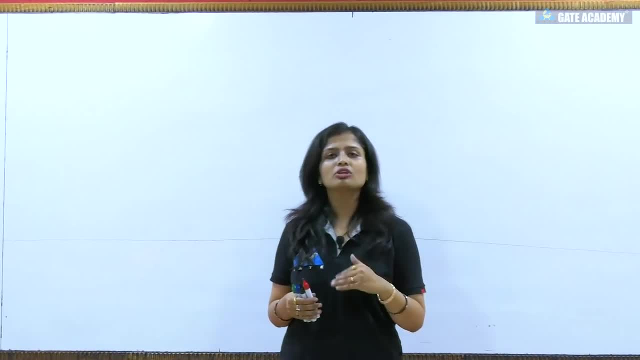 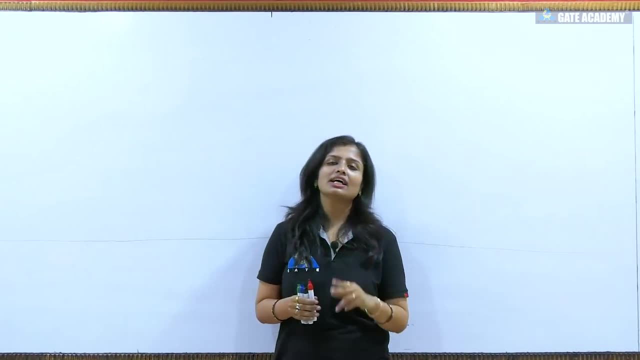 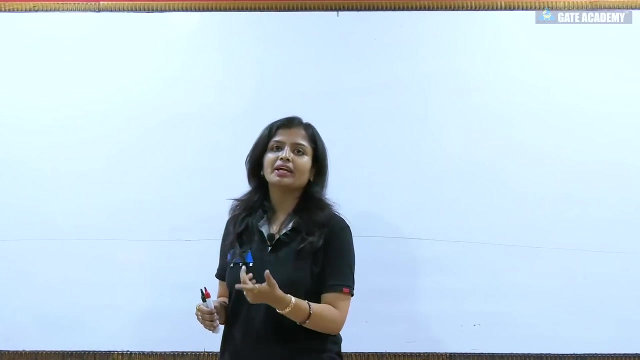 But if some kind of taste is present in water, then also we can't consume it. Fine, Sorry. So what happens is taste and odour. these two things are same Sometimes. if you smell from any water sample, normally if you drink that water. 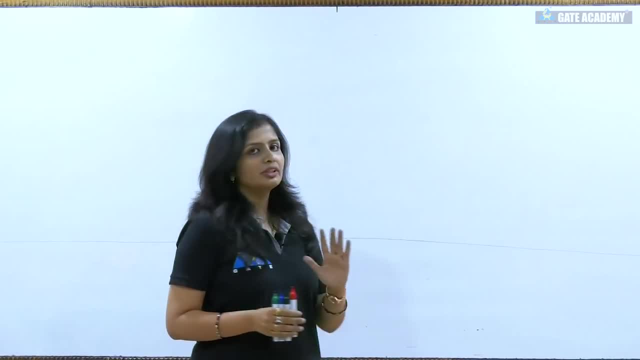 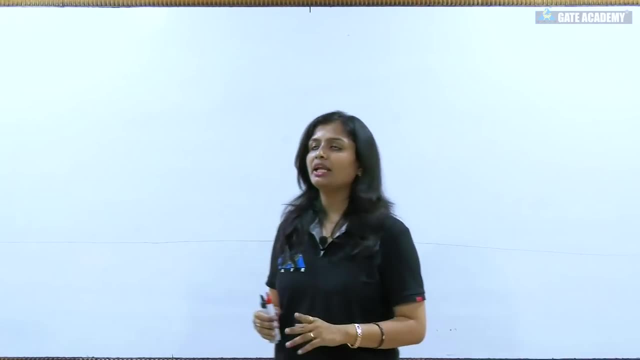 then there will be taste and odour. Fine, That's why we say that where there is odour problem, there is taste, and where there is taste problem, there is odour. Both are inseparable. That's why we can measure both together. 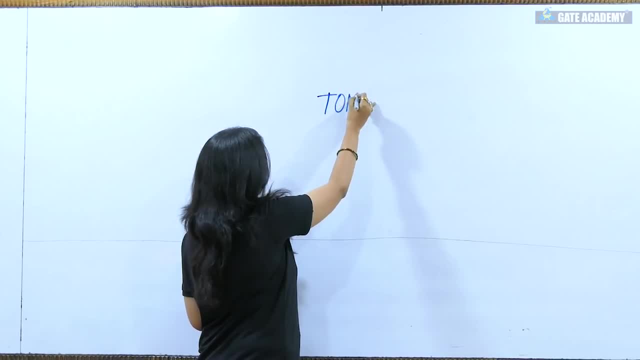 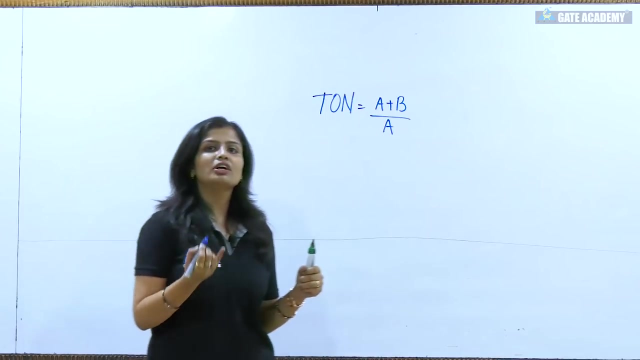 How We measure in the same unit, that is, Threshold Odour Number, which we call T O N in short form. Now, what is T O N? First of all, you should know its formula, if you can say A plus B, B, C and. 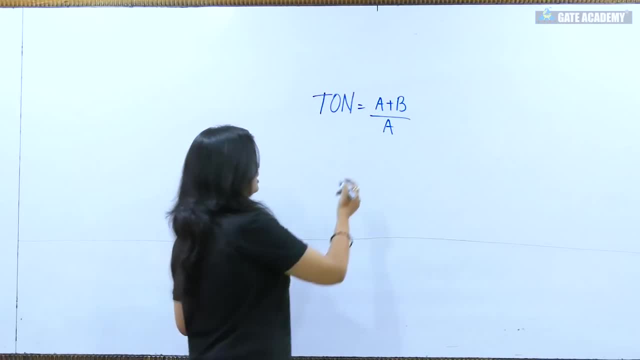 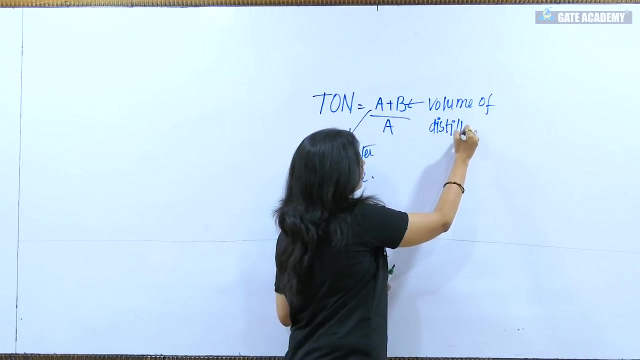 like this: it will be the volume of the water sample. You know from your water there is smell. you have taken that water. it is the raw water sample. Now you want that from that water the smell stop. So what will you do? 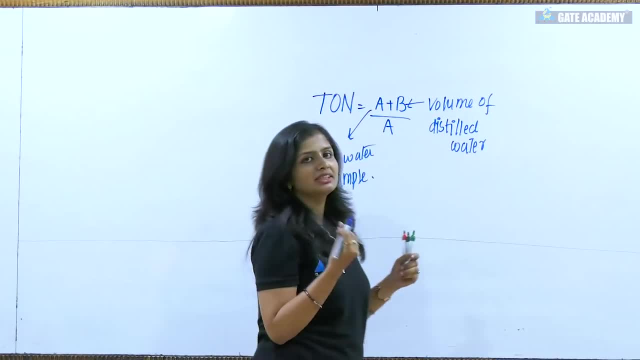 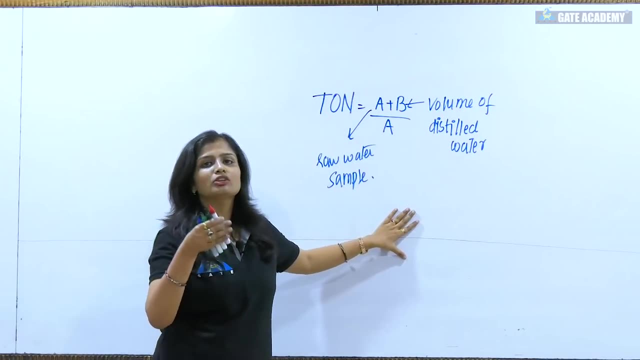 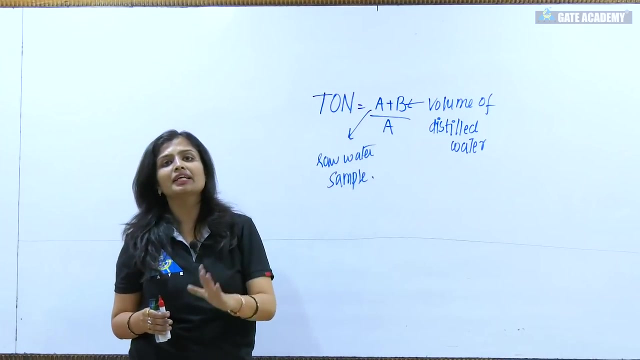 Take a distilled. Now understand its basic concept, that what is the threshold order number In threshold order number? first, you have a raw water sample from which either the smell is coming or the bad taste is there. Fine, you took the sample of that water. you will keep pouring distilled water in it until the smell or odor stops coming from it. 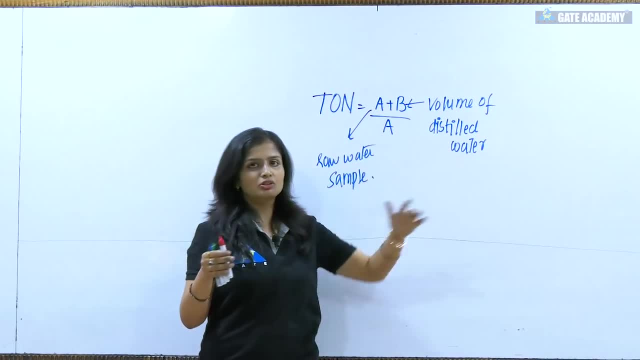 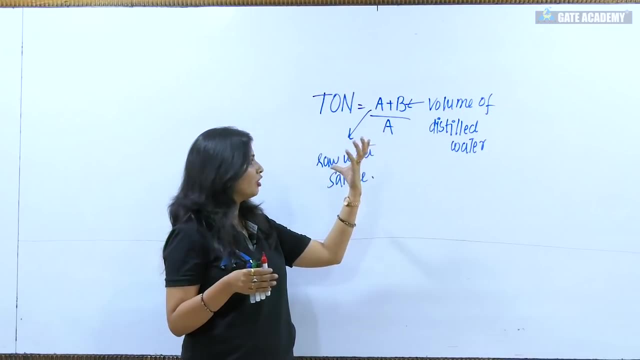 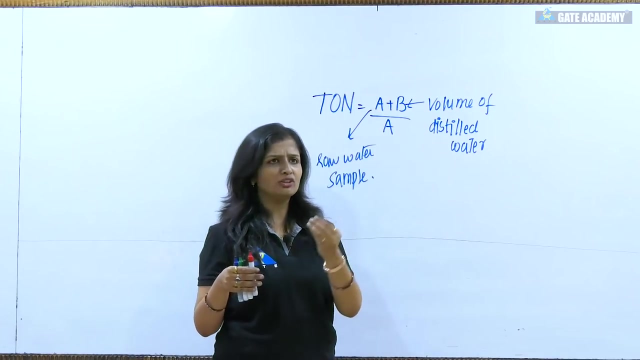 The moment when the smell is coming from the raw water sample or the taste is there. we can't detect the taste. The smell of the raw water sample is coming from the odor at that time, because you can smell it. If there is any hydrogen sulfide smell in it, it is very much the smell of hydrogen sulfide. 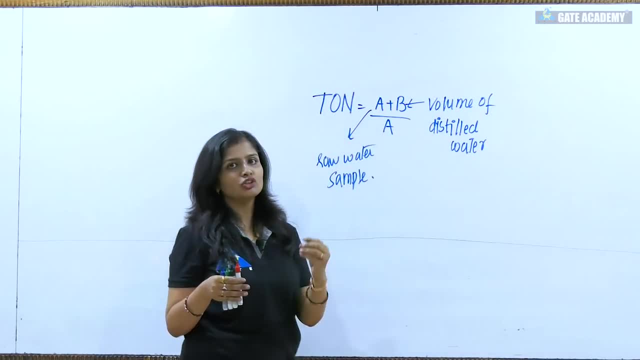 Generally the smell of the drain etc. smells the same if gases like hydrogen sulfide are present in it. So if you keep pouring distilled water in that water sample and at the moment you know if you have taken 1 liter of water in a beaker. 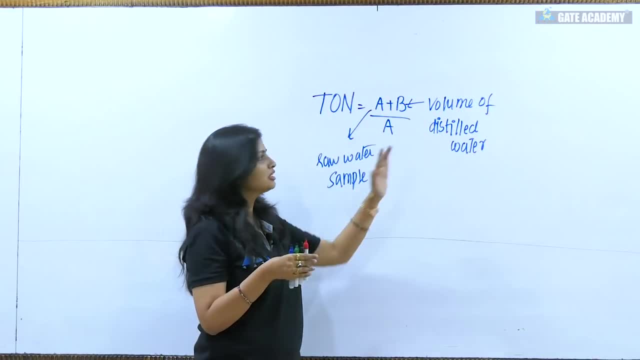 then you will be able to measure that, after pouring how much amount of water, the smell stopped, So you have put that amount of water. So you have put that amount of water. So you have put that amount of water When you put the water sample- initial raw water sample- in the beaker. 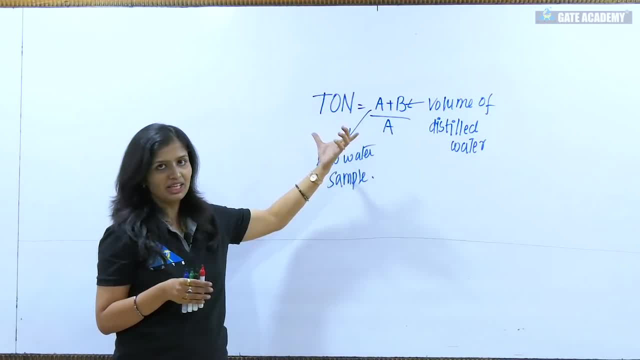 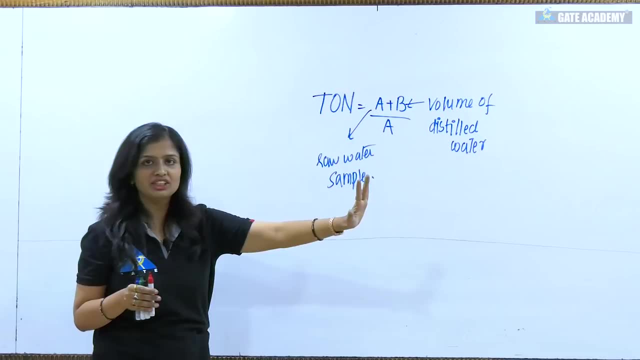 When you solve it, you will get the threshold order number. Fine, normally, as per Indian standards, the value of threshold order number should be 1 to 3.. Fine, it can ask you in 1 marks that you will get the raw water sample or will give the volume of distilled water. 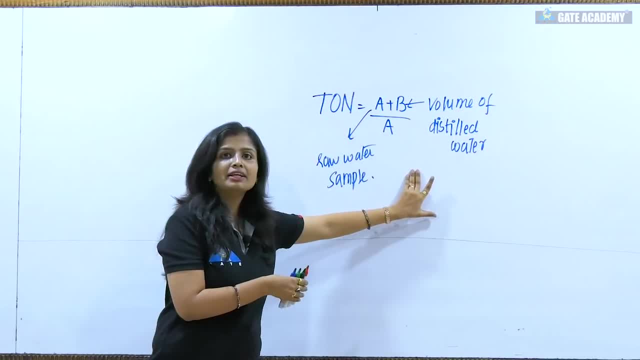 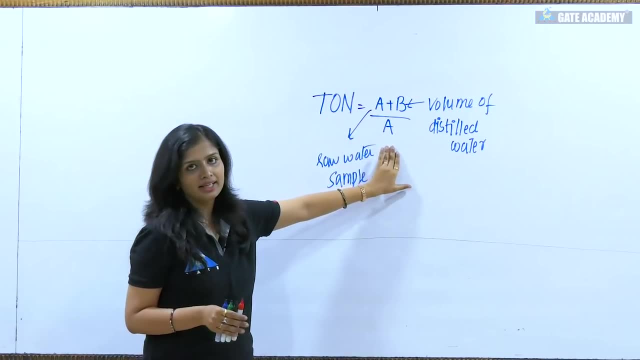 You will be confused that in the beaker do you want to write the raw water sample or the distilled water? So you always have to remember that the one who was smelling or whose odor problem you had. Fine, we have to write a plus b upon a only. 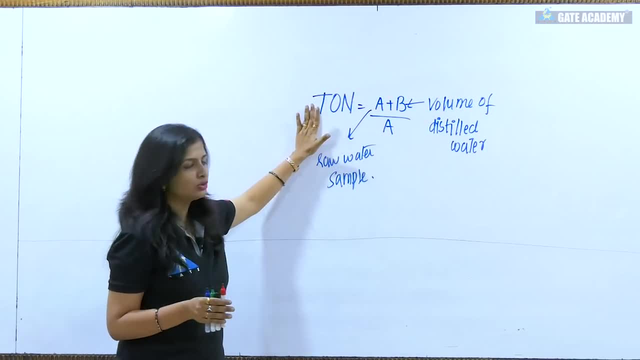 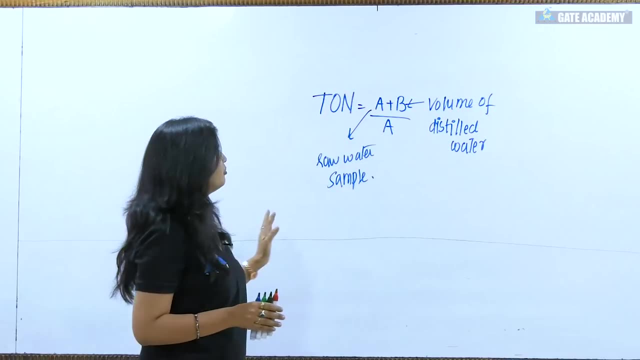 This is the part of confusion. This can be asked to you in one marks, And the permissible limit of the threshold number is 1 to 3.. And secondly, today we have an osmoscope instrument instead of the threshold order number. 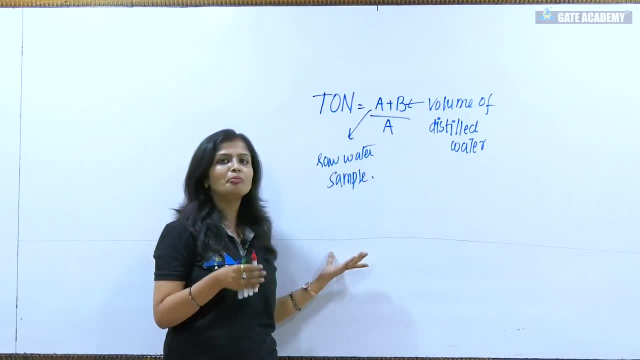 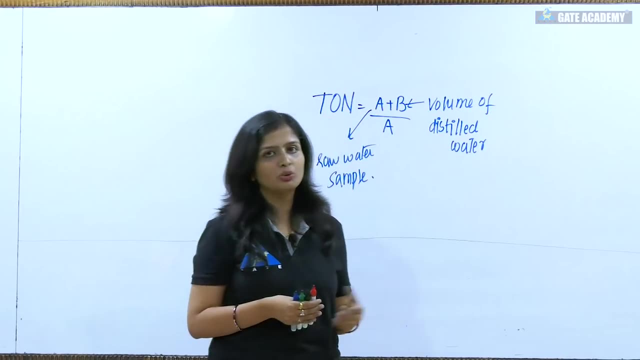 By which we can measure the threshold order number. Nowadays we do not need distilled water for the volume of the raw water sample. We can measure the taste and odour with the osmoscope instrument. Fine, so this was our complete odour and taste part. 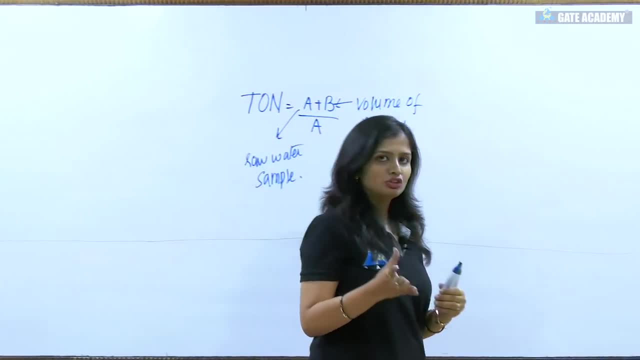 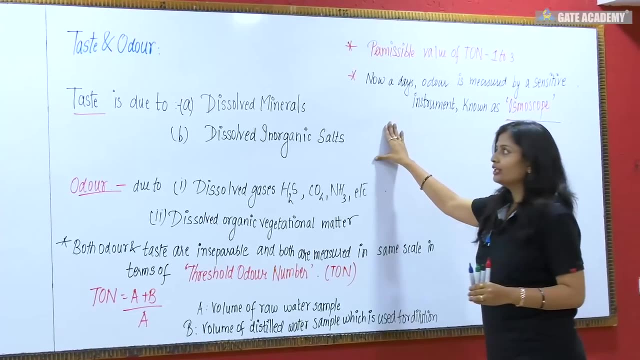 Now, whatever I have told you, you can quickly jot it down. That is why I have written it all down here in the whiteboard. That what all things you should know. If we talk about the taste, then why is the taste bad? 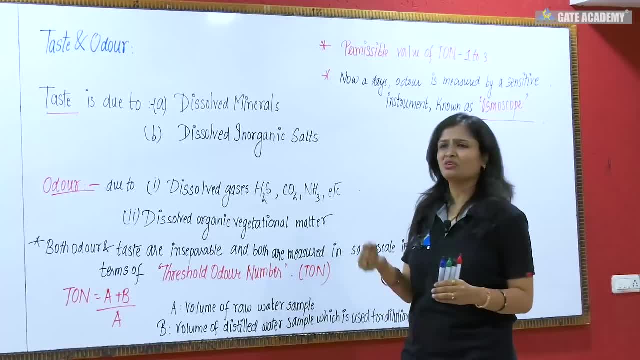 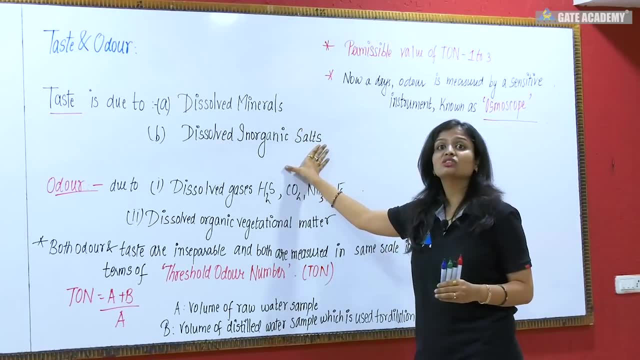 Sometimes we say that there is more chlorine in the water. It feels like it is chlorinated by drinking it. Chlorine seems to be chlorine. That means it has dissolved minerals in it. Sometimes inorganic salts are present in it. That is why we do not like the taste of water. 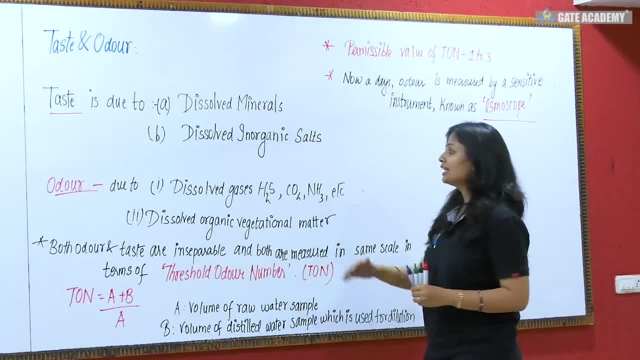 Okay. Similarly, let us talk about odour. Odour comes because of hydrogen sulphide gas is present, Or carbon dioxide gas is present, Methane is present, Ammonia is present, Any gas is present. It comes because of that. 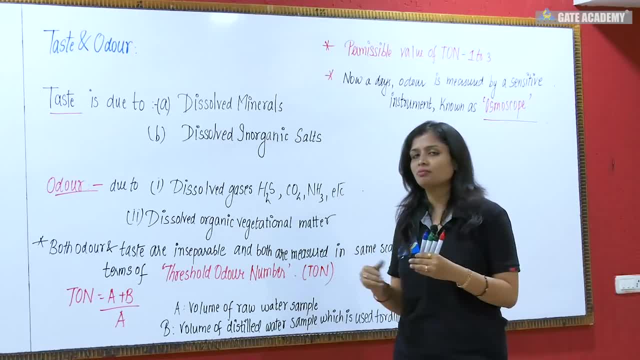 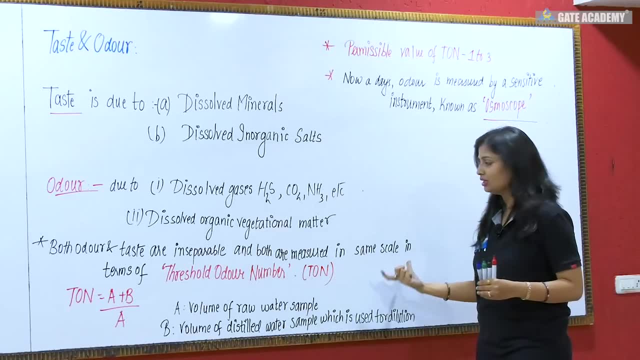 After that, even if there is any organic or vegetational matter in that water, then also we have odour problem. Now, whatever I told you here, both odour and taste are inseparable, And both are measured in same scale. In which scale? 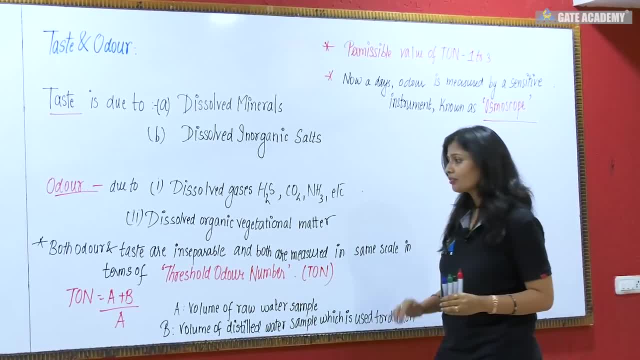 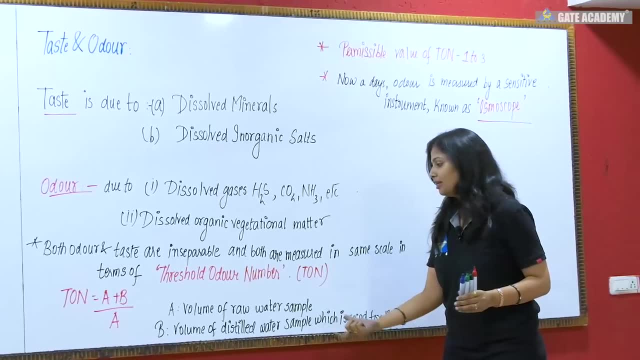 Threshold odour number, That is TOS. Now, what is this threshold odour number? A plus B upon A? Whatever, I told you: volume of raw water sample. What is B? Volume of distilled water sample, That is, for dilution. 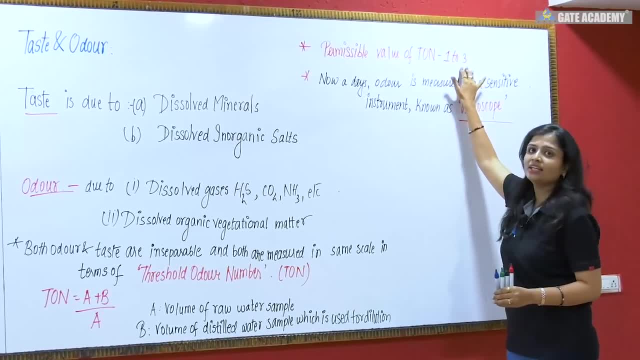 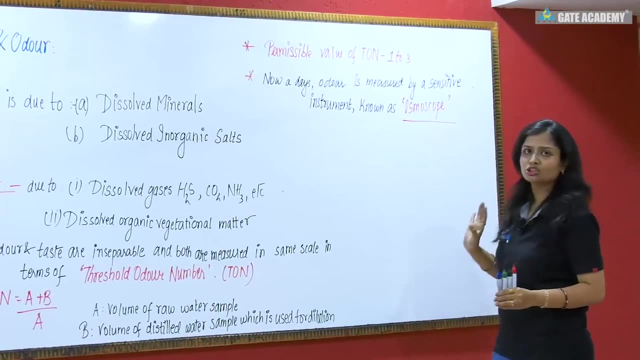 Fine, Now you know its permissible limit. The permissible limit of threshold odour number is 1,, 2,, 3.. And nowadays we measure odour with an instrument which we call osmoscope. Fine, So this was our taste and odour part. 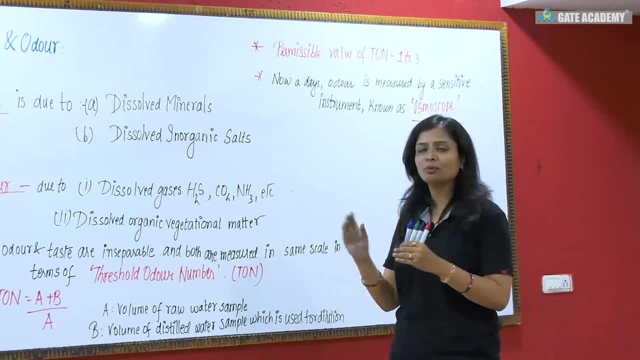 We talked about colour. In that we said: what is the permissible limit- 5 to 20 ppm. And when we talk about taste and odour, what we are saying here is: what is the threshold? odour number 1 to 3.. 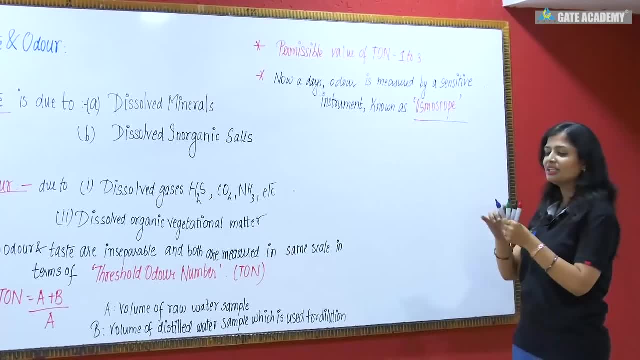 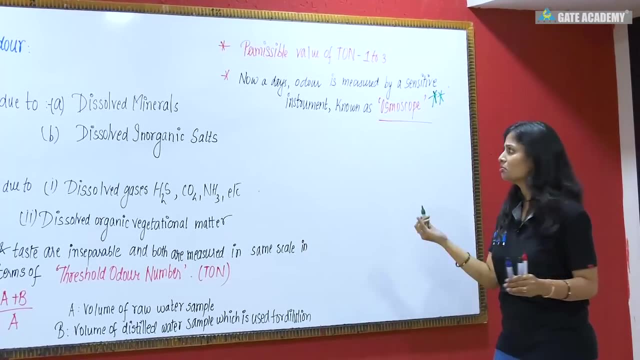 So you have to remember these permissible limits too, And along with that you have to remember these instruments too, Because in Maths, the Following it can ask you. this Osmoscope will give you tintometers, nephelometers, and it will ask you. 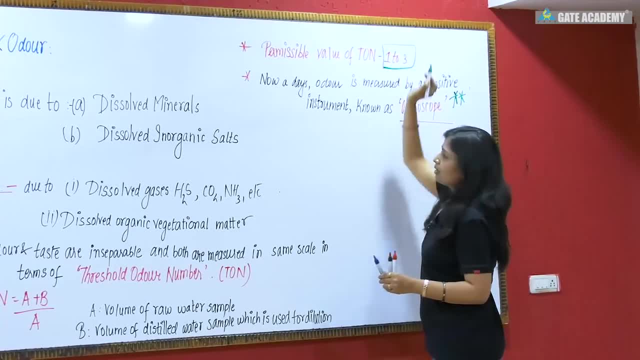 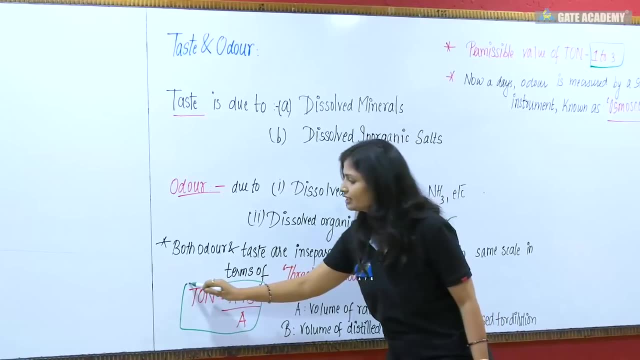 Fine, And you should also know the permissible limit of threshold odour number And, along with that, the formula of threshold odour number. If it will give you raw water sample and distilled water And it will ask you the threshold odour number, 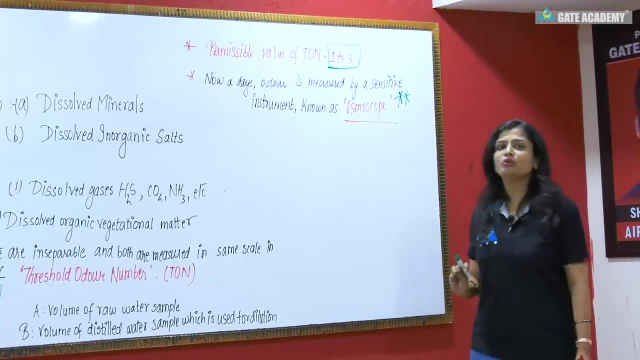 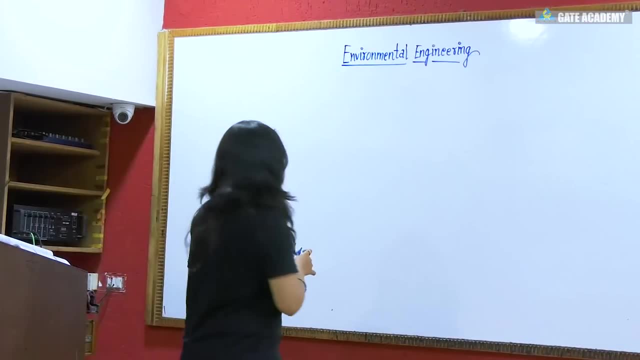 So you should also know this too Fine. Now we will be moving to the temperature part. Now coming to the temperature part, We discussed the turbidity, We discussed colour, odour. Now the temperature of water. When we talk about temperature, 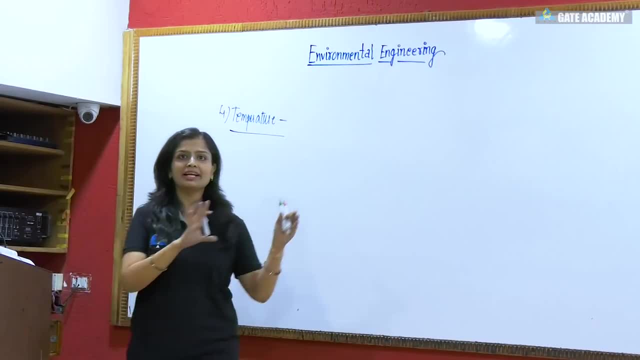 So the temperature First. you guys understand, I will be writing all the points for you So that you can jot down and make your notes. Firstly, when we talk about temperature, So the temperature, The supply of water should be maintained. 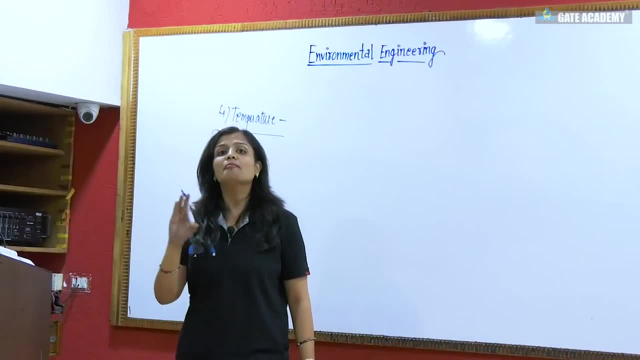 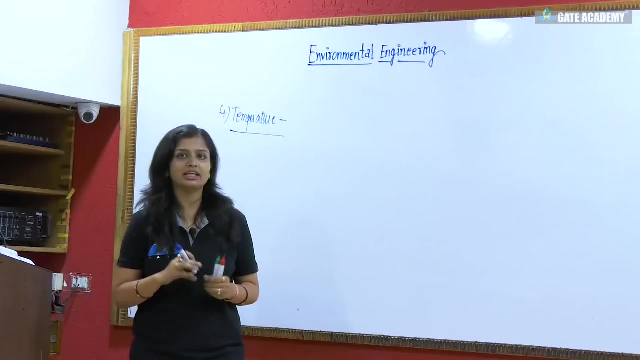 It should be maintained from 10 to 20 degrees Celsius. If the temperature of water is more than maximum 25 degrees Celsius, Then it becomes objectionable for us. So 10 to 20 degrees Celsius is an ideal temperature. That means the water should flow in that temperature. 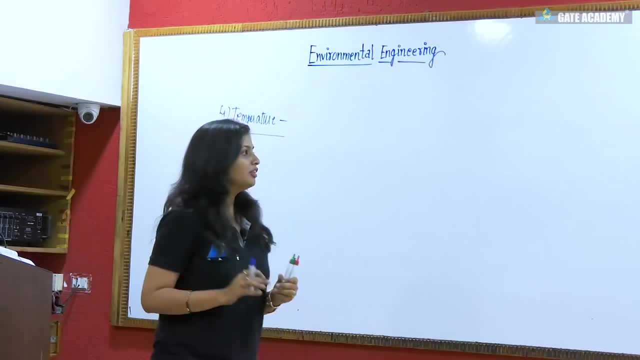 Or the water should be supplied in that amount of temperature. First point. Secondly: how do we measure the water temperature? We measure it with normal thermometer. So here also we will measure the water temperature with thermometer. But if there are water bodies of large surface, 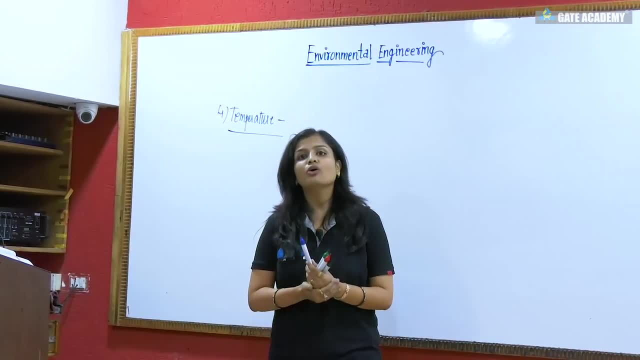 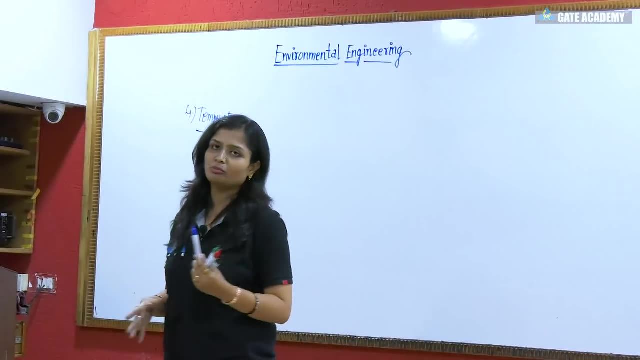 Whose temperature we are not able to measure with thermometer. In that case, we use broken capillary thermometer. This is the type of thermometer which we use In case of large surface water bodies To measure their temperature. Fine, Apart from this, why temperature is important for us. 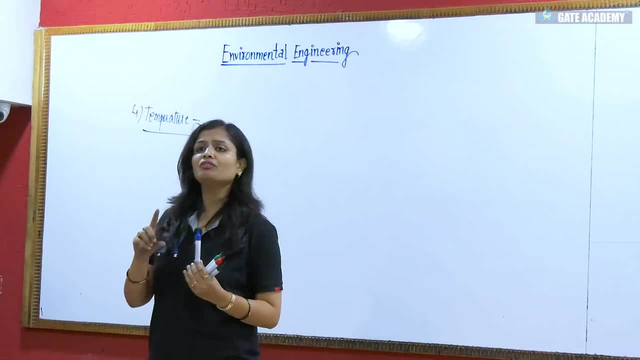 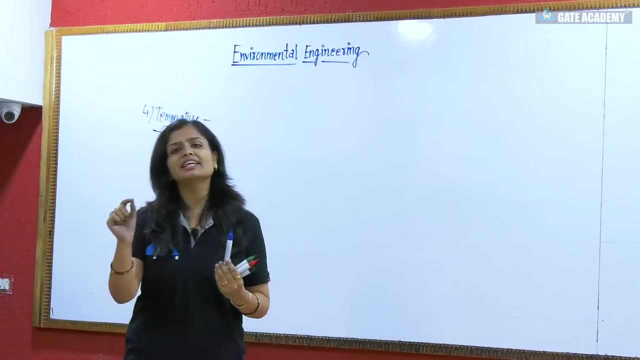 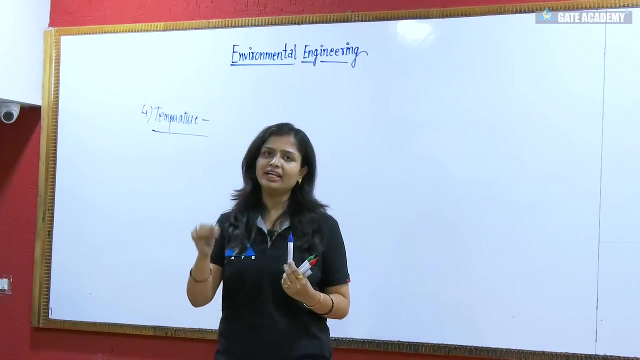 Because temperature of water is important, because It controls the chemical and biological activity of water. If you increase the temperature of water by 10 degrees, Then the biological activity- Suppose there is a harmful bacteria present in it And it is 10 degrees Celsius. Normally we have to maintain the temperature for maximum water supply by 25 degrees Celsius. But in case the water temperature is 35 degrees Celsius And if any amount of biological bacteria was present in it, Then it will double its growth In every 10 degrees Celsius increase. 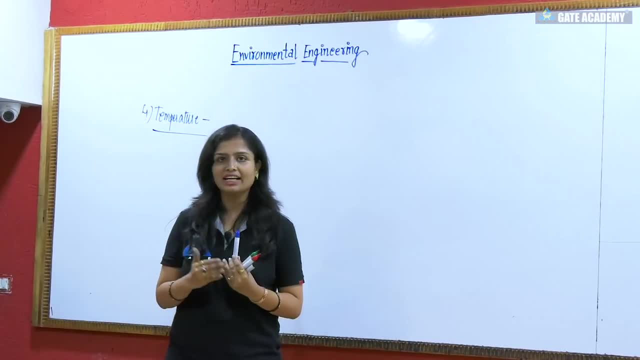 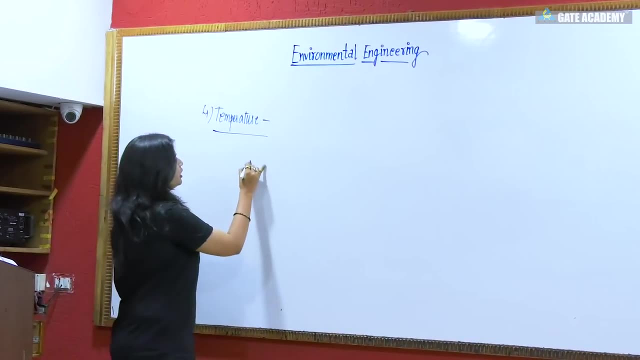 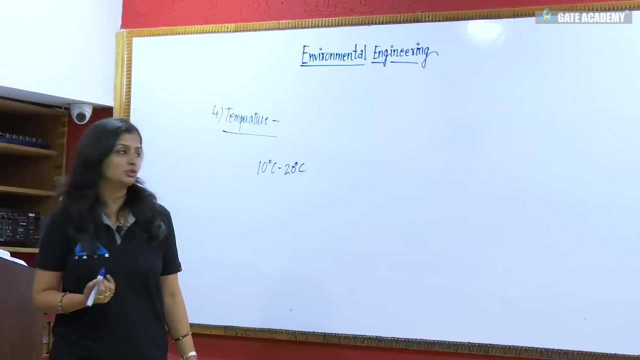 It doubles its growth. The organisms of biological activity. Fine, So this was our temperature part. I told you that temperature should be 10 to 20 degrees Celsius. We can measure it with thermometer. For large surface water bodies We use broken capillary thermometers. 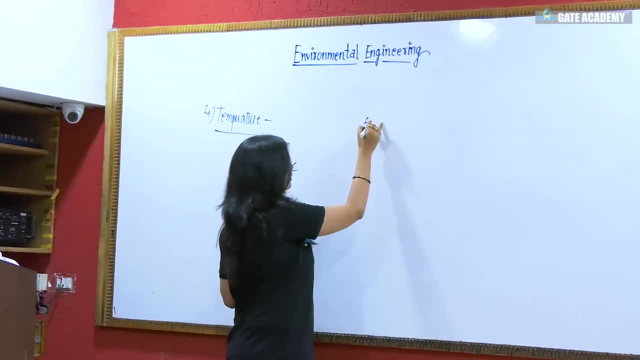 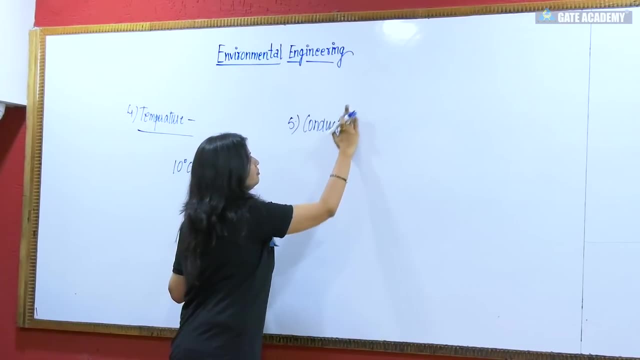 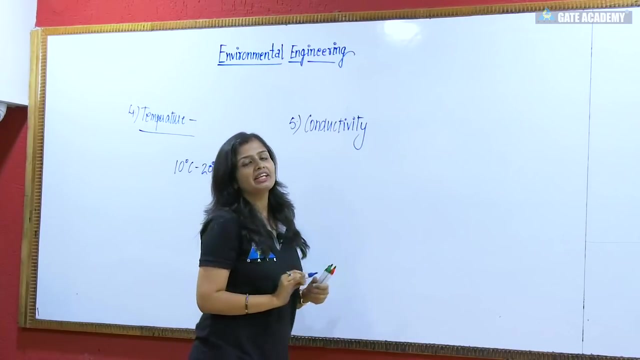 After this I will make you write all the points First understand. Last is the conductivity. This is our last parameter When we talk about our physical parameters. So conductivity is the last one Now when we talk about specific conductivity. 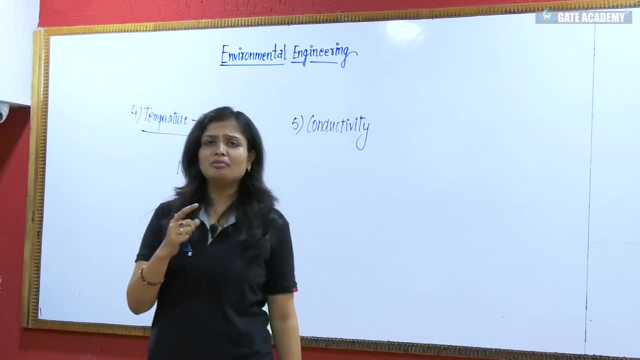 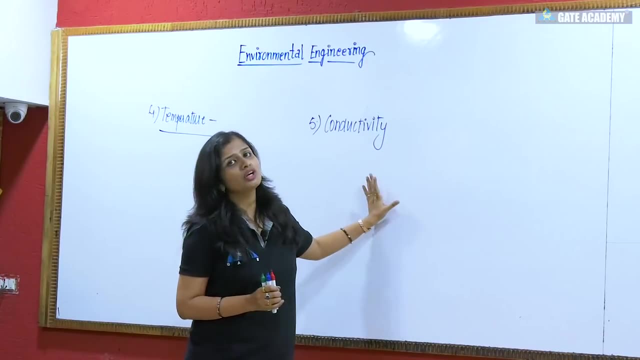 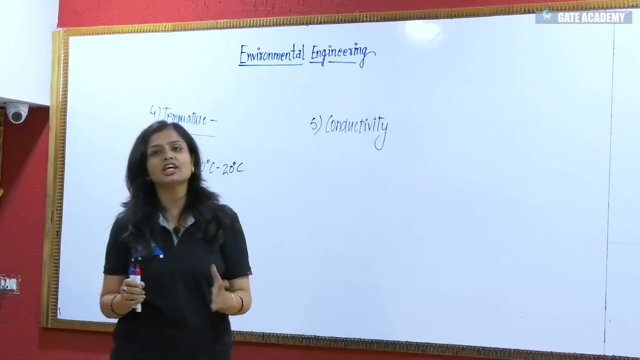 So what do we understand by conductivity? Conductivity means Sometimes dissolved salts are present in water. So if dissolved salts are present, Then they will show conductivity. Fine, You must have read What is the opposite of resistance, What is the opposite or inverse of resistivity. 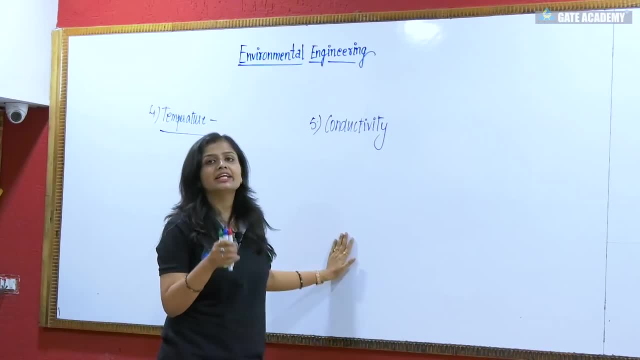 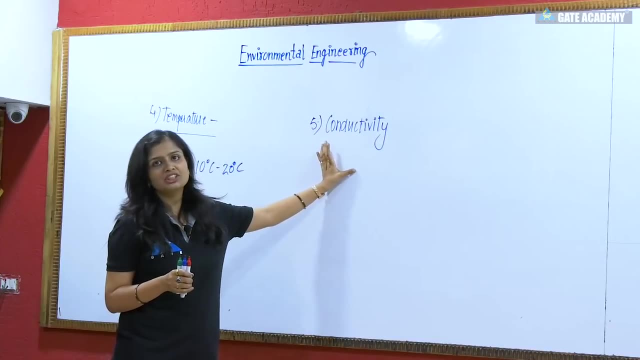 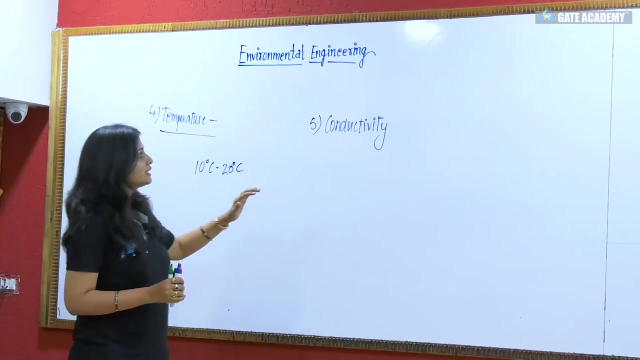 Conductivity. So what happens? It tells how many dissolved salt ions or dissolved salt contents are present in water. This conductivity is measured by portable dionic water tester at 25 degrees Celsius. Fine, And its unit of specific conductivity. You call it conductivity. 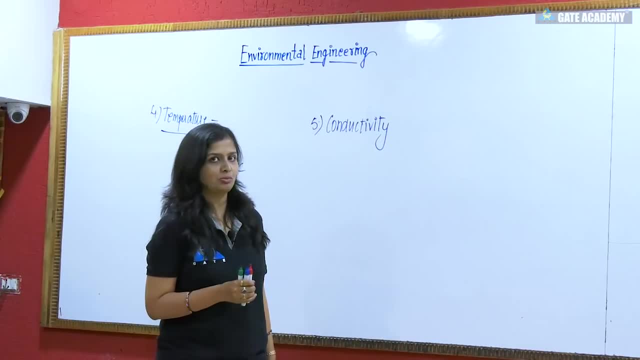 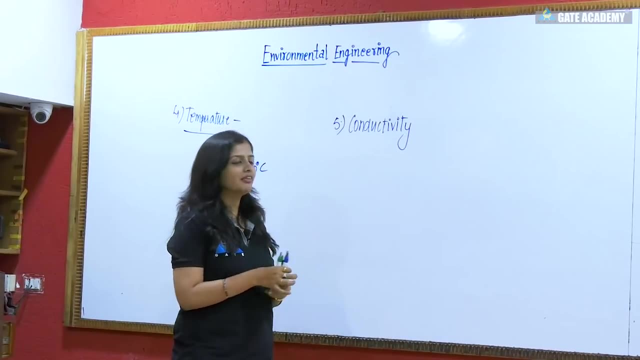 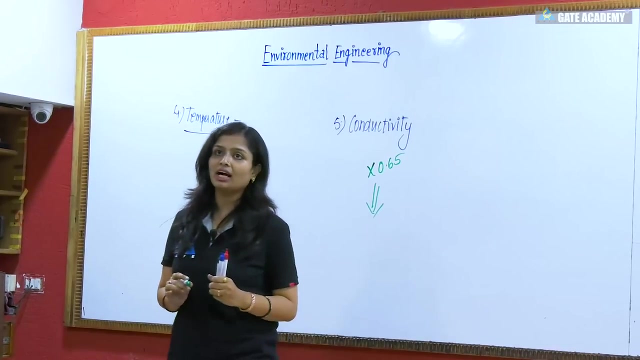 Micromose per centimeter at 25 degrees Celsius. What happens in this? If you want the value of conductivity, If you take a value from the water tester, Whatever your conductivity is, You multiply it with 0.65. So you will get the total amount of dissolved salt content. 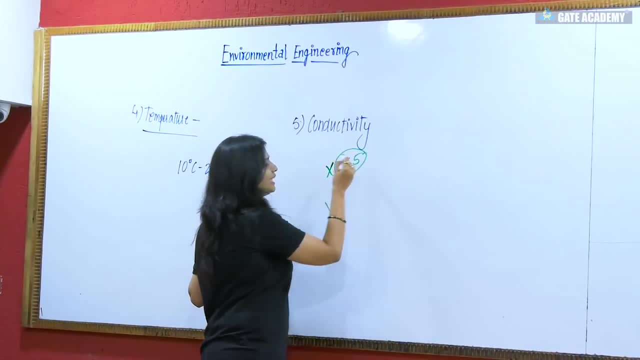 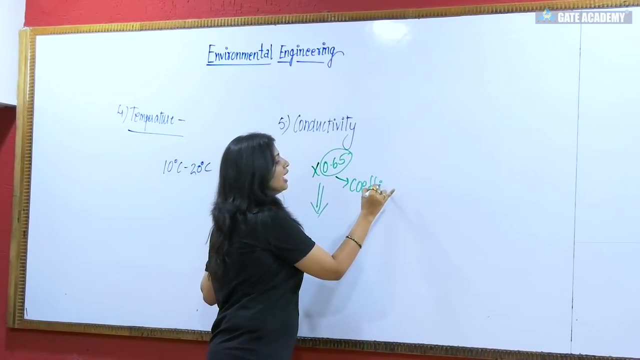 Now you will ask: Where did this 0.65 value come from? This is a general value that we use. However, this coefficient, Its value, differs for different types of salts. We know that It is given in the questions. 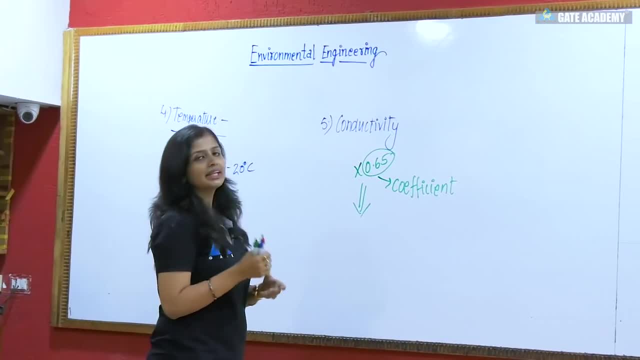 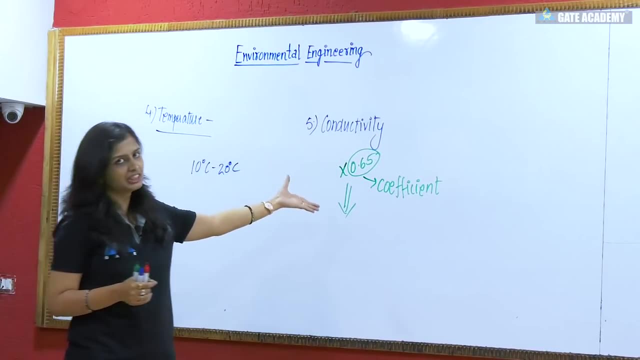 If you are ever asked What is conductivity? How much salt content is there? So you will take the value of portable dionic water tester's conductivity. We will multiply it with 0.65 coefficient. You will get the salt content. 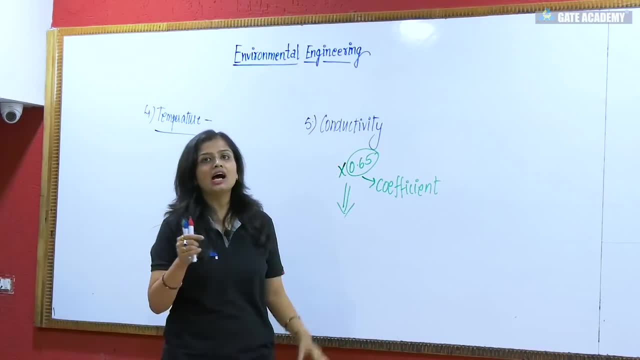 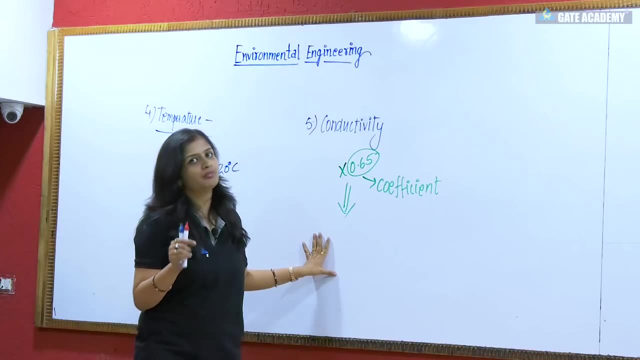 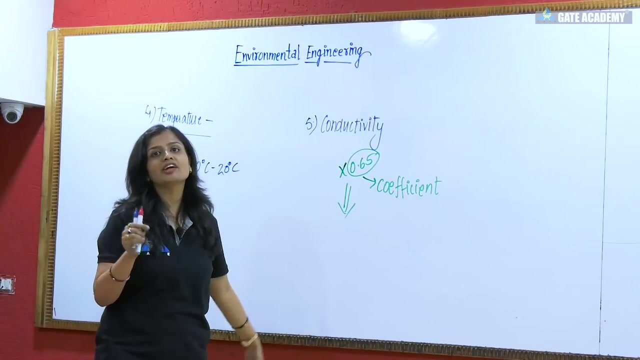 Fine. Apart from this, you should know one more thing: The more salinity, the more salt content, the more conductivity. I am repeating again: More the salinity, more is the conductivity Fine, And we don't want Any amount of conductivity in our water sample. 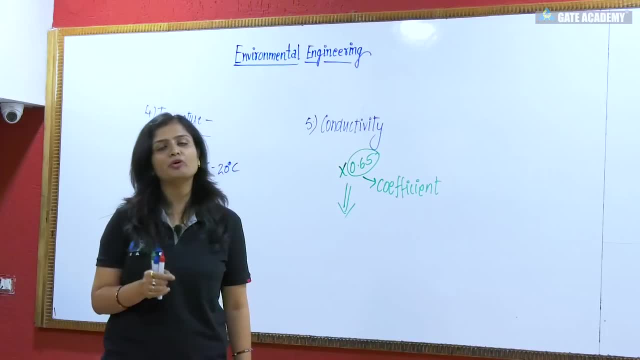 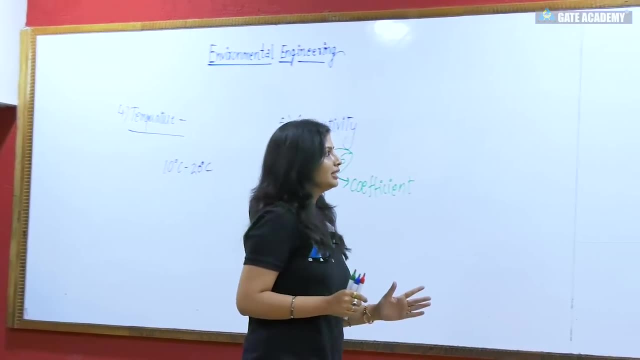 So the permissible limit of conductivity is nil. We don't want conductivity in any amount. So whatever I have just told you In temperature and conductivity, You quickly make notes of it. I have written this for temperature. I will read it for you. 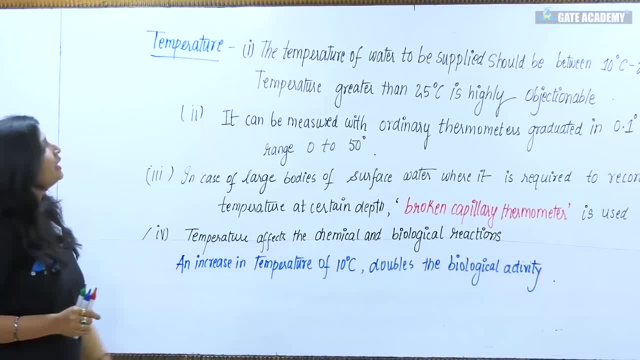 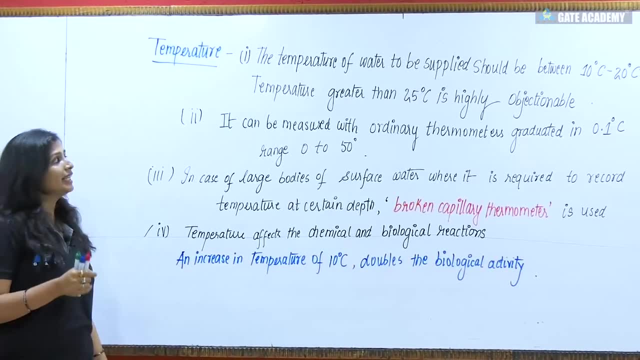 So that you will also get a quick revision. First point: The temperature of water to be supplied Should be between 10 degrees Celsius to 20 degrees Celsius. Temperature greater than 20 degrees Celsius, Temperature greater than 25 degrees Celsius is highly objectionable. 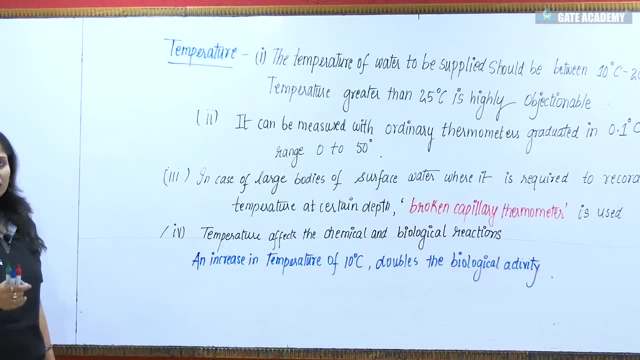 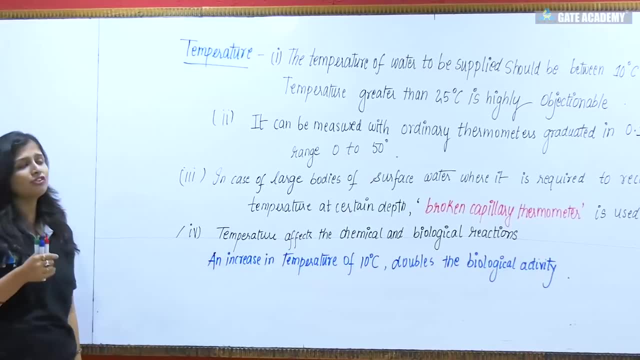 Second, It can be measured with ordinary thermometers Graduated in 0.1 degree Celsius range, That is, 0 to 50 degree. Third point: In case of large bodies of surface water, Where it is required to record the temperature at certain depth. 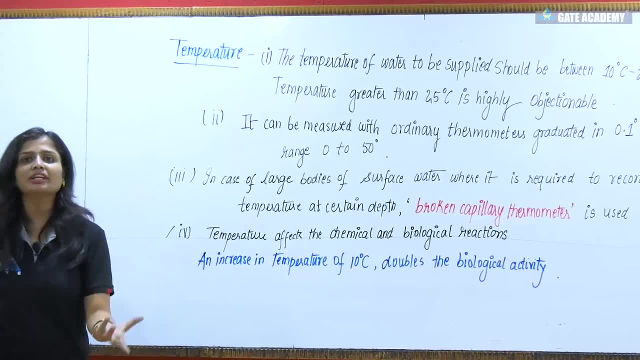 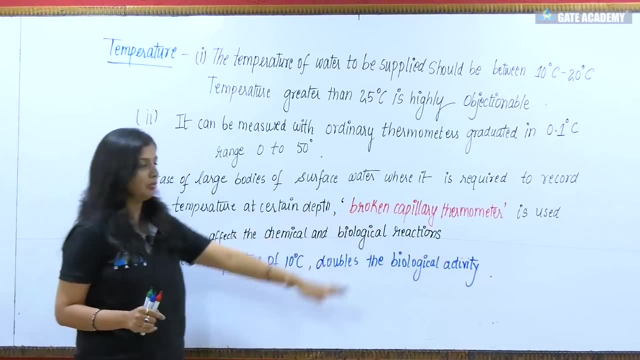 We should know the temperature. What is the temperature of water at a distance of 10 meters from the water surface? What we use there- Broken capillary thermometers, Broken capillary thermometers After this- For that temperature affects the chemical and biological reactions. An increase in temperature of 10 degrees Celsius Doubles the biological activity. So specially what you have to remember here is That temperature is 10 to 20 degrees Celsius. Greater than 25 degrees Celsius is harmful for us, And we can also measure it with ordinary thermometers. 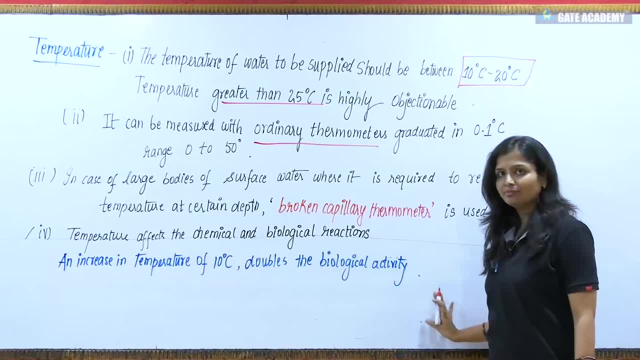 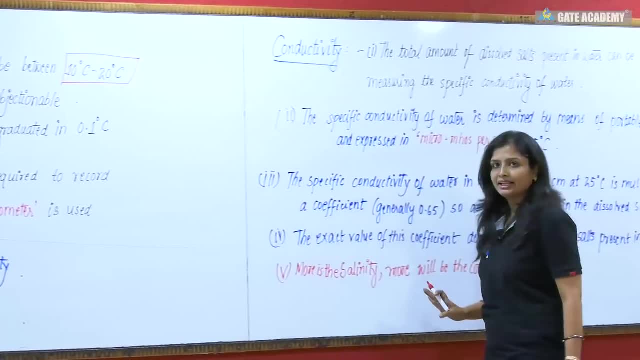 Fine, So I think you have jotted down all these points. Now, after this, we will talk about conductivity, Conductivity, Whatever I have told you in conductivity, I have written all that here So that you note down First what we will talk about in it. 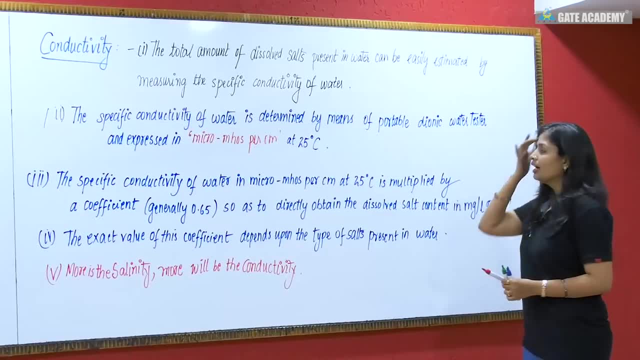 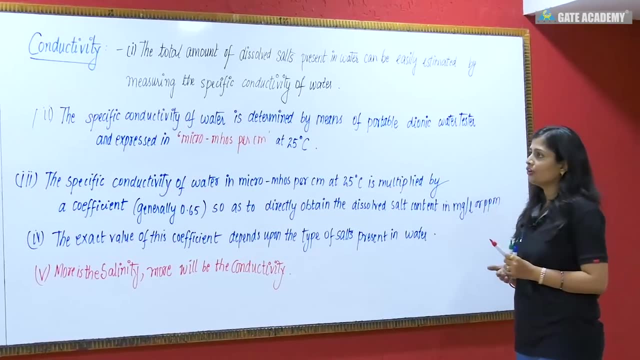 The total amount of dissolved salts present in water Can be easily estimated by measuring the specific conductivity of water. Second, The specific conductivity of water Is determined by means of potable dionic water tester And in which we express this I have already. 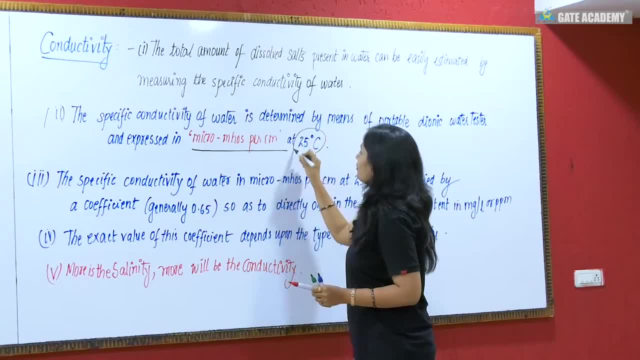 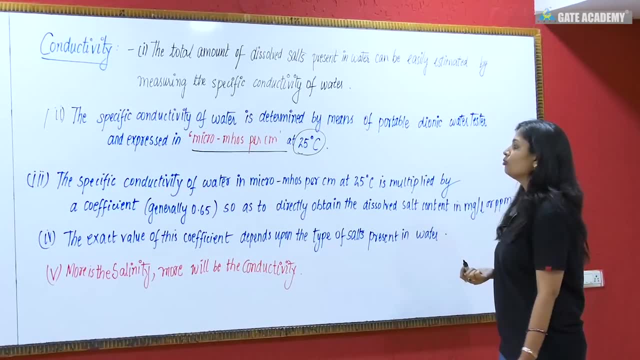 Micros moles per centimeter, And you should also know its temperature. It should be measured at 25 degrees Celsius. Third, The specific conductivity of water In micro moles per centimeter At 25 degrees Celsius Is multiplied by a coefficient. 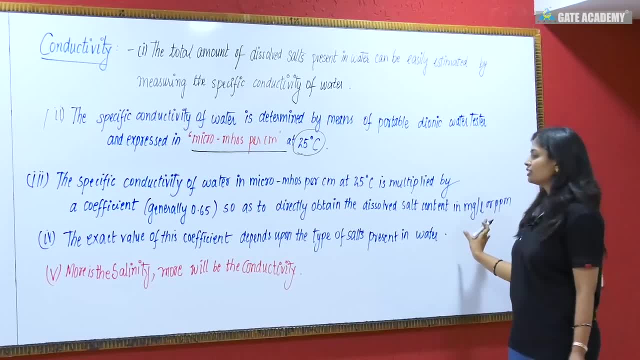 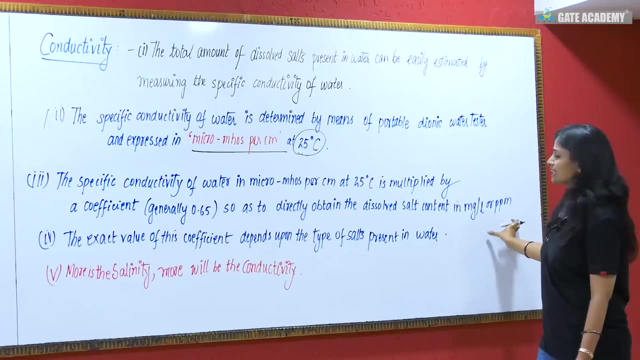 Generally we take it as 0.6.. So as to directly obtain the dissolved salt content. If you know the conductivity, Multiply it with 0.65.. Generally, you will know the dissolved salt content directly, In which you will know the unit.